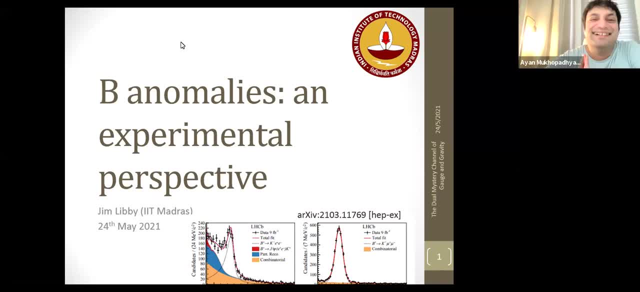 But thanks, thanks for the promotion. Okay and yeah, and also, and also other experiments, and and and And. today he will be talking to us about this new exciting bee anomalies that have been that, that that has become more and more convincing, and he will try to convince us today that it is indeed not something that will change physics in the future. So over to you, Jim. 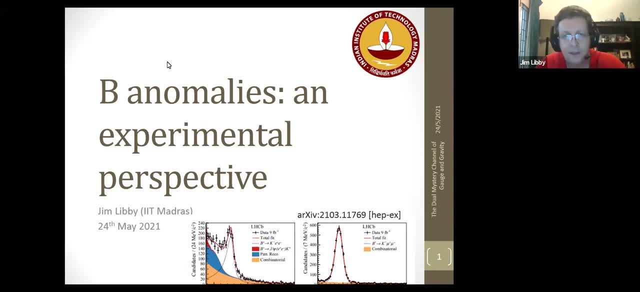 Okay, so thank you, Ayaan, for the invitation and the introduction. So I will be very much focusing on the experimental side of these anomalies. I will at times touch upon the phenomenology as well. but really, what was the genesis of this talk and much of the recent excitement? is this paper from LHCB related to a certain type of bee decay, which I'll describe in some detail as we go through? 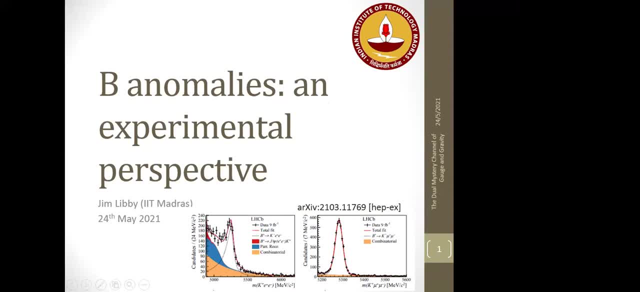 Jim, may I interrupt a little? Yes, please, So is this? somehow the whole of the slide is not being visible at one is. are you intending to do that thing? It is to me. I don't know what's missing. 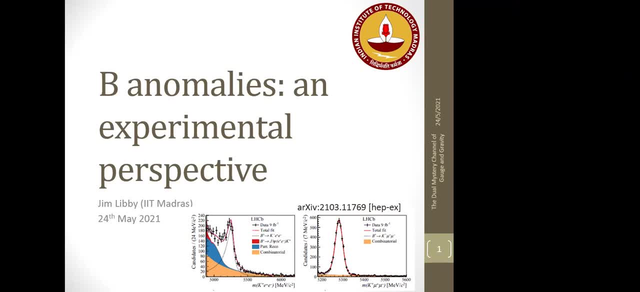 Well, there is this stripe in the right hand side, but I think it's a little bit which also gives the that one. yeah, that's part of your format. Yeah, so are the aspect ratio. Okay, let's change Okay. 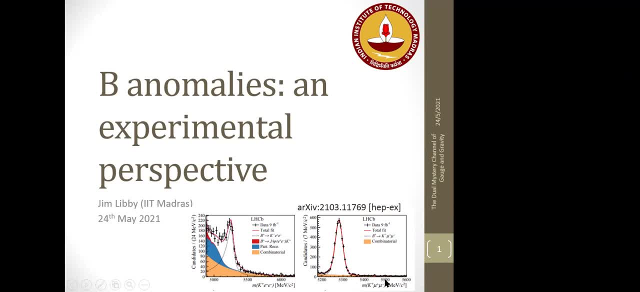 Let's see, I, You could not. I guess the problem is if you can't see the axes, labels or anything at the bottom. Yes, indeed, Yeah, You can't see. No, No, now it is, but previously, I think, when we were scrolling up a little, a part of the slide was not visible, That's all. 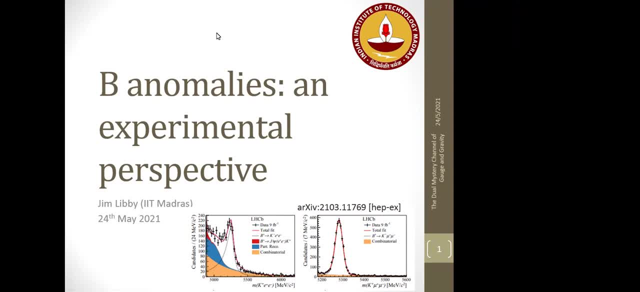 Okay, I'll continue. Yeah, I don't know what to do. This is usually what I do with PowerPoint and it's normally fine. Okay, let's see how we go. If there's a problem, let me know and I can potentially make a PDF or something, and it may be better. 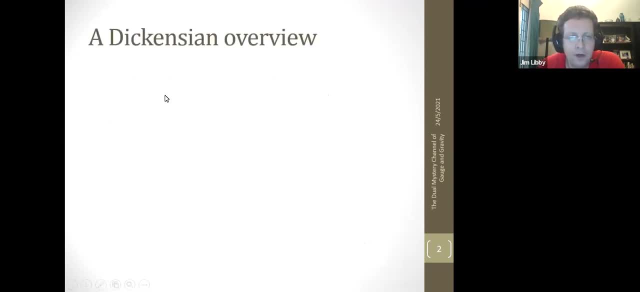 Okay, so I'm going to do an overview and I'm going to make some references to Dickens throughout this. You'll see why when you do that And then you get to the conclusion. But essentially I'll begin with a very brief introduction about bee anomalies in the past. 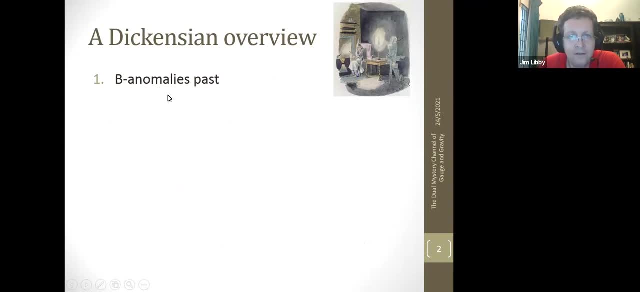 And I'm being rather generic in how I interpret bee anomalies here. This is really about flavour physics and the important role it's played in the development of the standard model, And then, like Scrooge, we will move on to the bee anomalies of the present. 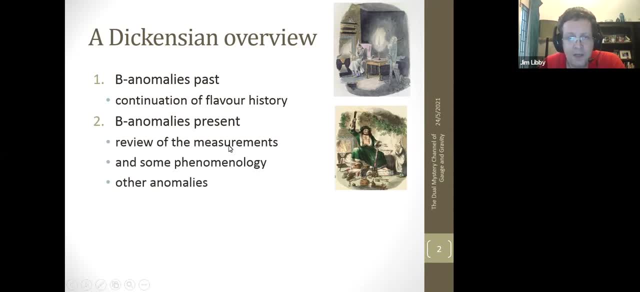 And, in particular, I will review the methodologies. I will talk about the bee anomalies that are being discussed. and I'll talk about the bee anomalies that are being discussed. There's a whole pattern of measurements, Some not quite as recent as the one that's highlighted from LHCB this year, but there's a whole pattern of measurements that need to be discussed when you talk about the bee anomalies. 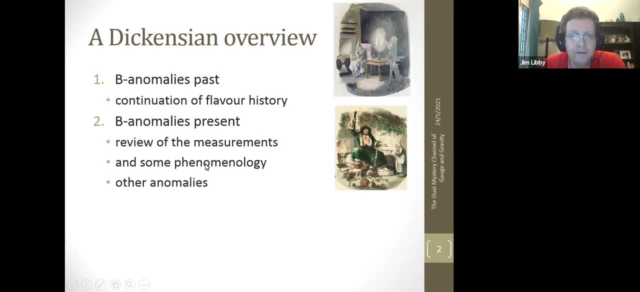 And then I'll talk a little bit about the phenomenology that may describe these, And then I'll refer to some of the other anomalies that are getting press as well at the moment, most notably G-2.. And then I'll talk about the bee anomalies in the future, which essentially is: 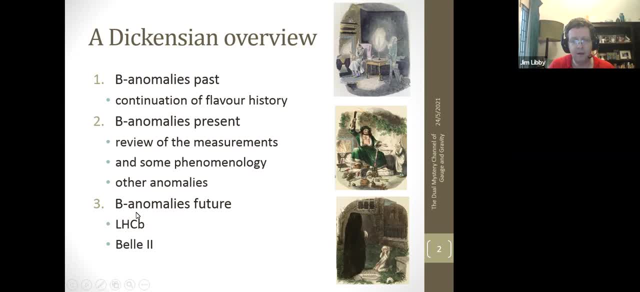 talking about two experiments. I'll be very brief on LHCB, though they're the ones that are driving a lot of the measurements that we see today, But I'll talk a lot about Bell 2, which is what I work on principally. 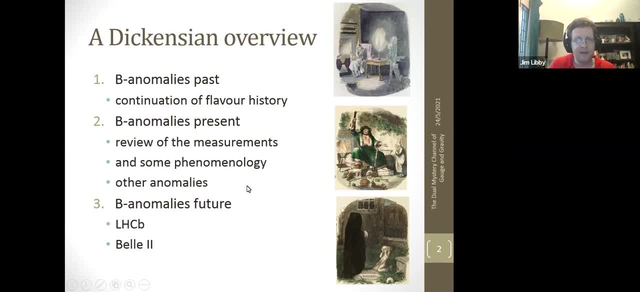 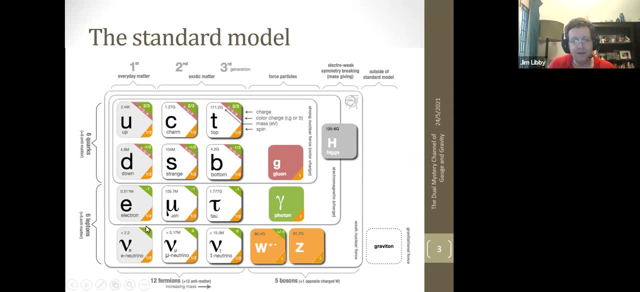 So hopefully it won't be as a distressing experience as this for you, but we'll see how we go. All right, so such a talk would always begin with the standard model, and what I'm going to be talking about today is the way that bee anomalies work. 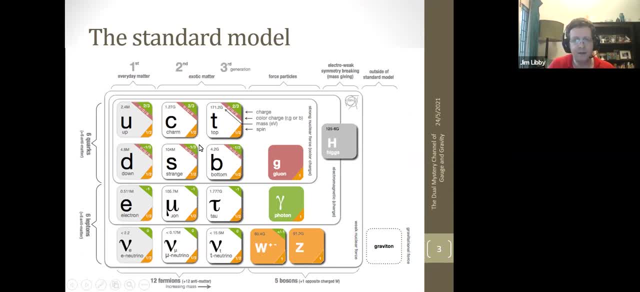 So we have a weak interaction amongst the quarks. That's really what flavor physics means And this paradigm that we have in the standard model of three generations, three forces, local gauge, invariance leading to the force carriers, and then, ultimately, the masses explained by the Higgs boson. 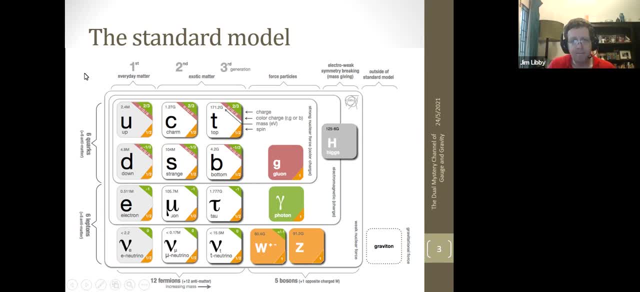 it's been extremely successful over 40 years since Glashow, Weinberg and Salam proposed this, So successful, in fact, that it's been a while And we've been awarded, I think, roughly 14 Nobel Prizes for different aspects of this, and many of these are clustered around. 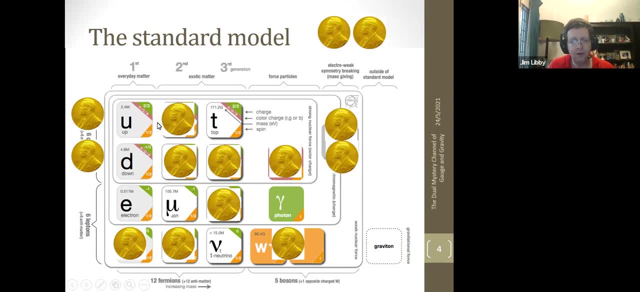 what's here in the flavor sector and also in the weak sector, And I will talk a lot about how the not a lot, but I'll introduce how the standard model was built up from some observations coming from flavor. But of course we know this is not the whole story. I don't want to repeat the usual things that are said that there are. 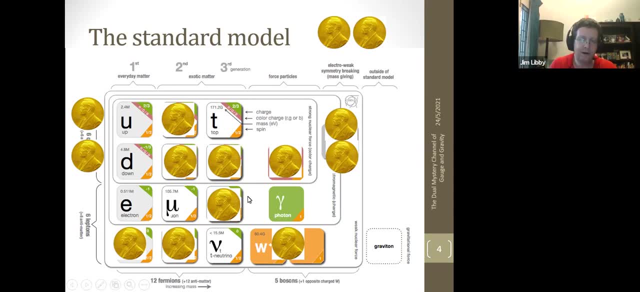 obvious problems with the standard model. There's a lot about matter, and then there's various aesthetic problems related to fine tuning and this three generational structure not really being clear why we must have that, why not four, why not five? And 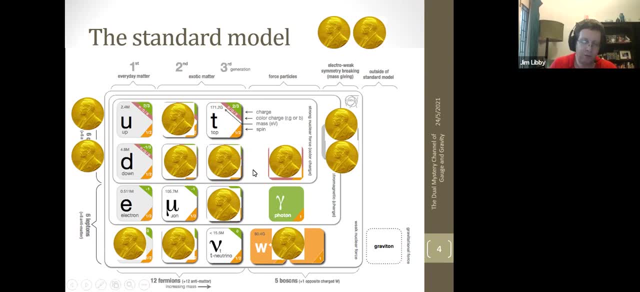 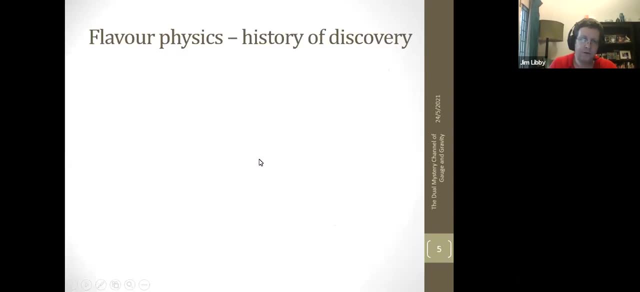 the goal has been in collider physics is to try and find measurements that would disagree with this picture. So first I'll just do my history and talk about flavor physics, because it really emphasizes the role that it plays when we're looking for new physics in these types of measurements. 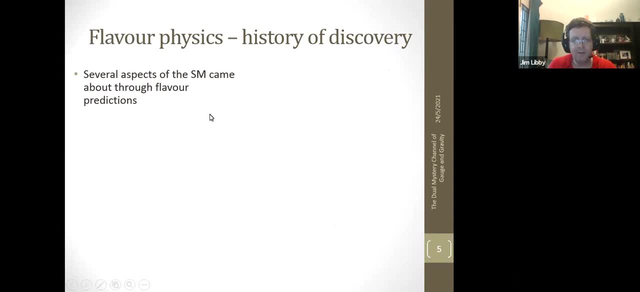 So several aspects of this standard model that I just showed you came about through flavor predictions. Probably most famously is the gym mechanism whereby the suppression of this neutral K-on decay- the K long- to two leptons, was resolved by Glashow, Illilopes and Maiani by suggesting that one extended the Kbibo mixing that was there amongst the up-down and the strange quarks, to add a fourth quark, which naturally led to a cancellation that would suppress this rate. 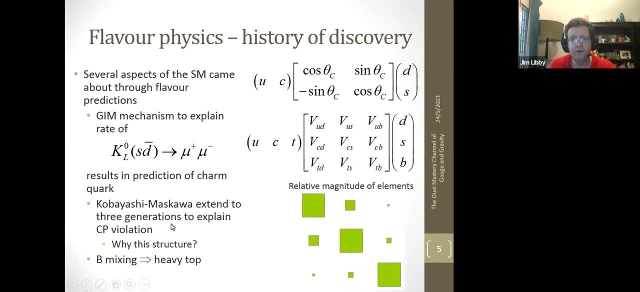 Then Kobayashi and Maskawa actually took this further and realized that one could get CP violation within this quark mixing matrix If you extended it to three generations, and this was even before the charm quark was discovered. so they predicted the top. 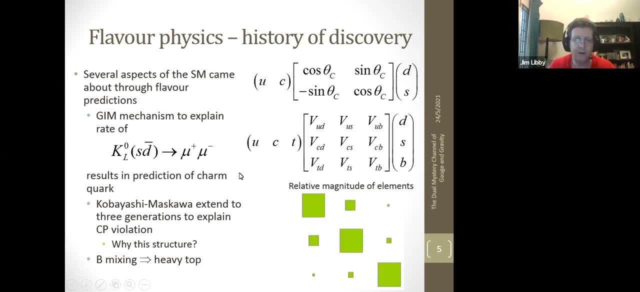 and the bottom quark, ultimately a third lepton as well in the tau, and this, of course, turned out to be the correct paradigm, But it also emphasizes one of the issues that one has with the standard model is that we really do not understand the numerical values. 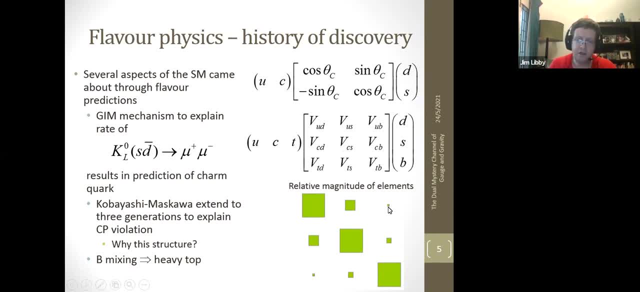 that go into the four parameters that describe this matrix. There's a strong ranking of the elements here where, if you couple together the first and the third generations with VUB and VTD, the size of those elements is much smaller than those on the diagonal. 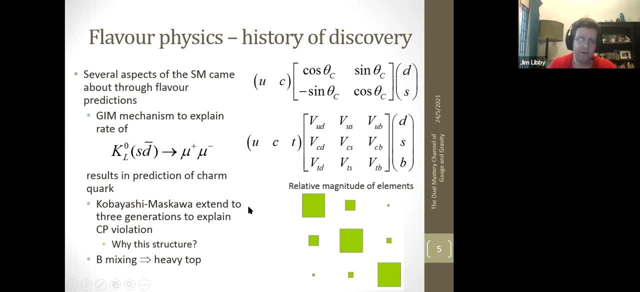 So where this structure is coming from is one of the outstanding problems of the standard model, But one I'll just highlight here before moving on to the rest of the talk is is bee mixing and how it predicted that there must be a heavy top quark. 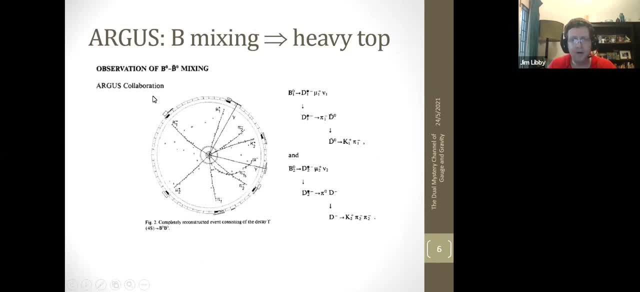 So in 1987 the Argus collaboration, which was really one of the first original bee factories operating at the epsilon 4s producing pairs of bee mesons, discovered the bee meson oscillations, and the signature for this was to see: 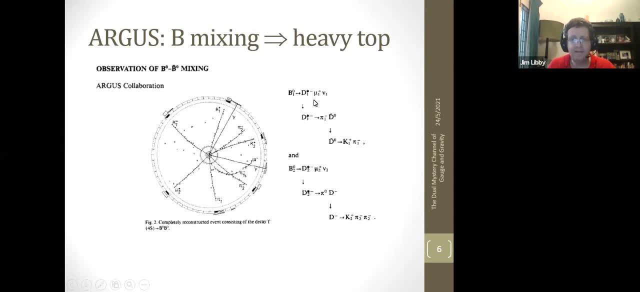 semi leptonic decays of the bee, which are the predominant decays where you have like sign di leptons. So here you have a muon of positive charge and another one on the other side, and this is a very nice signature. And also this picture emphasizes something about E plus, E minus collisions. 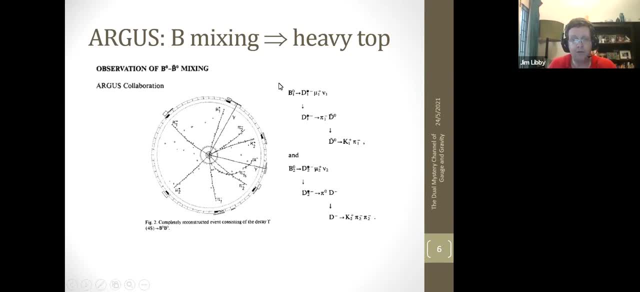 producing pairs of bee mesons, Which is what we do today at Bell 2 as well, that one has a very clean, pristine environment in which to study these decays. Now, the mechanism for bee mixing is dominated by this loop process whereby you have Ws and top quarks in the loop mediating this. So this box diagram, which is basically changing flavor by two units because you have 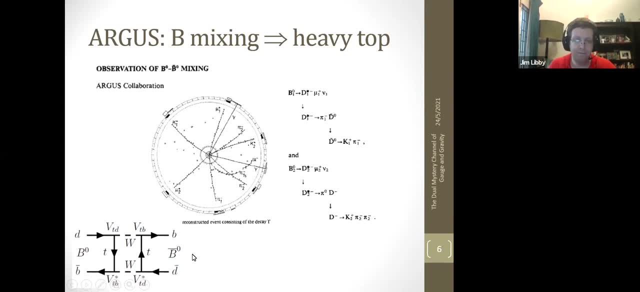 Ws and top quarks in the loop mediating this. So this box diagram which is basically changing flavor by two units, because you have beauty of one on the left hand side, the initial state, and beauty of minus one on the final state. So it's changed by two, these delta F equal to transitions. 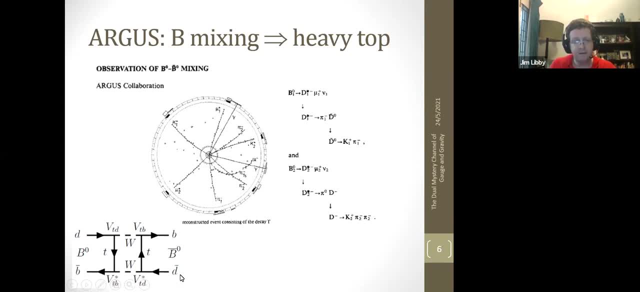 And the rate at which they observe these types of events, predicted that the mass of the top quark had to be greater than 50 GeV, and it then took another decade or so to actually discover this at the Tevatron, with a mass of 175 GeV. And the mass of the top quark had to be greater than 50 GeV, and it then took another decade or so to actually discover this at the Tevatron with a mass of 175 GeV, And the mass of the top quark had to be greater than 50 GeV, and it then took another decade or so to actually discover this at the Tevatron with a mass of 175 GeV, and then took another decade or so to actually discover this at the Tevatron with a mass of 175 GeV. 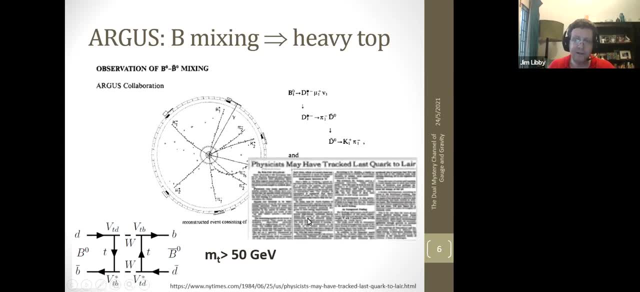 In addition to this, like most things that has already been discovered, In addition to this, like most things that has already been discovered At UA1 and UA2 or UA1 by Rubier and others- this is a headline from the New York Times from three years earlier that said they'd already found the top quark. 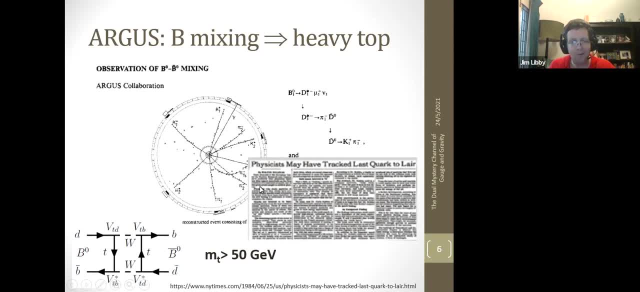 So what I'm saying here is that these precision measurements in bee physics have helped predict other features of the Standard Model, in the same way that the Higgs was predicted from precision hechoit on photo All star with measurements where it's it'snam. That's one thing. when you hear temas of 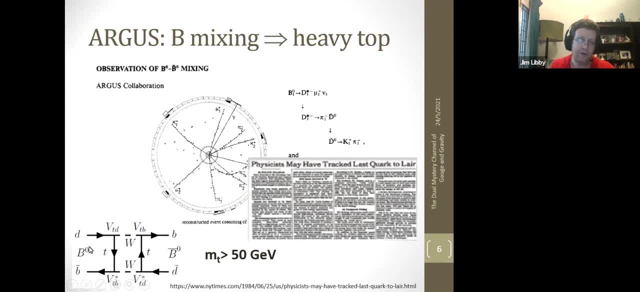 where its mass might be roughly, and also beam isons with masses of 5 gv are probing mass scales an order of magnitude higher than its own mass, and- and this is really what we're doing today- is we're using such processes to try and understand mass scales at a much higher value than the big. 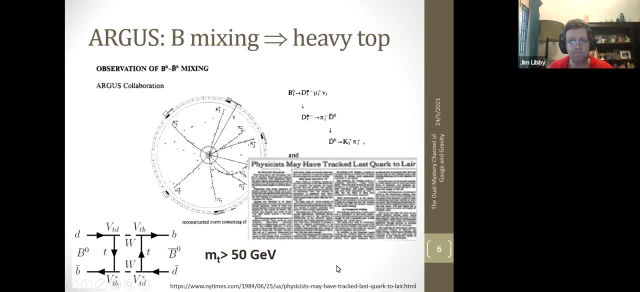 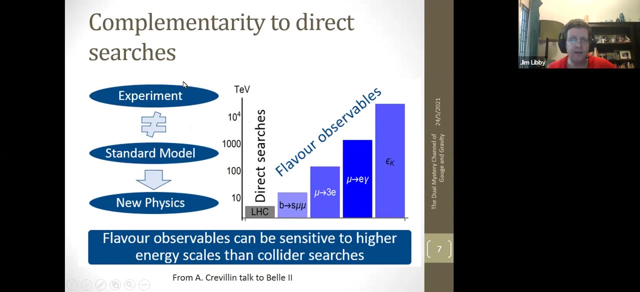 quart mass, which we can do through these types of precision measurements. so this has played an important role in us understanding the structure and and the hierarchy that's there in the standard model as we've gone through over the last few decades. so this is a nice slide that i've 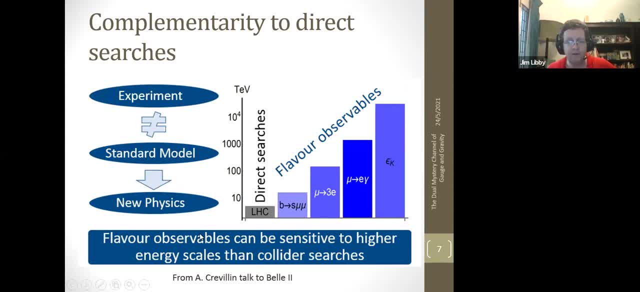 stolen from a talk we were given on bell 2 after the recent anomaly uh announcement from lhcb by andres crevelin, who's one of the people who works a lot on b2s, mu, and basically what we do is a simple flow diagram that we make our 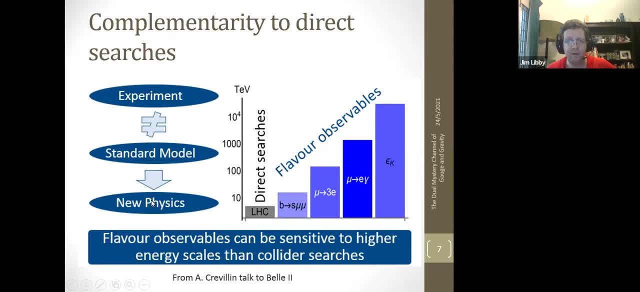 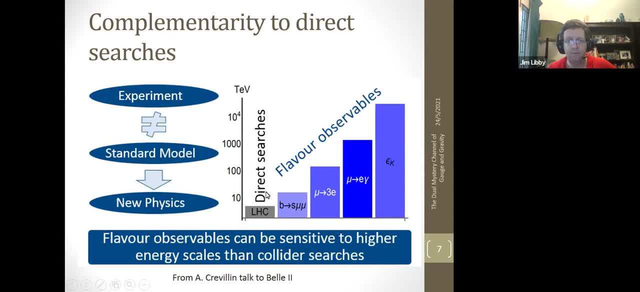 and this complements what's done directly at the lhc. at the lhc you have 14 tev of energy and you can make massive particles of ta- tv scale potentially- and through the last 10 years, 12 years, they've been successively setting as good a limit as possible on these. 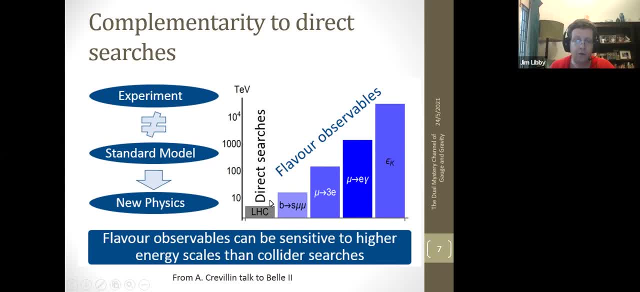 types of new particles, whether they be super symmetric or otherwise, but they are limited by that center of mass energy to make these direct discoveries, whereas if you look at precision measurements of flavor variables, so this shows some here in the quark sector. this bs to mu, mu and epsilon k related to cp violation in the kaon sector, as well as lepton number. 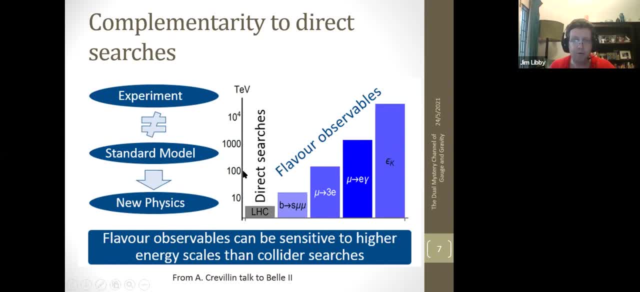 violating decays of muons. you are actually probing mass scales, or you can probe mass scales that are very much higher than what you're working at, because you have very strict limits on what can actually be happening in these loop processes that will mediate these decays. so this is an indirect search. 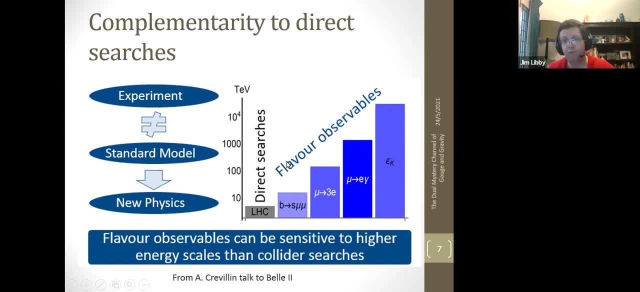 for new physics. now, as you'll see as we go through, the drawback of this is: it's not necessarily obvious what the new physics might be, and i'll talk about jim. can i ask something? sure, sure, so, uh. so your point is that, uh, the, somehow, this b, quark oscillations and this b, this beam essence form, give a very clean environment, so it. 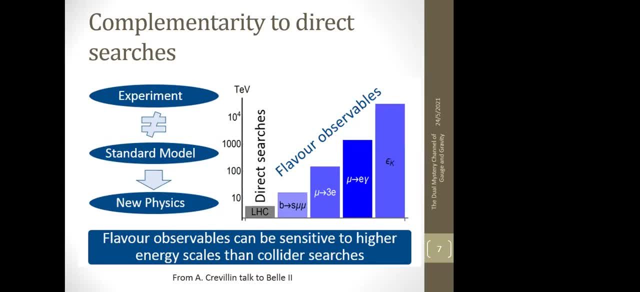 was not quite clear. just from the properties of, say, the tau lepton or something, what should be the mass of the top of b, but uh, but from this you could get a clean estimate. is: is this: uh, that's correct, that's correct. so sorry, just going back to this. so 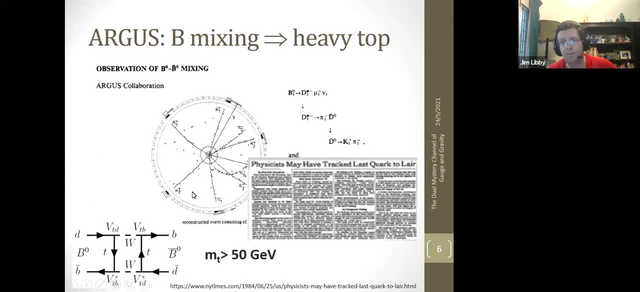 so this box completely drives the rate or the mass difference between the two cp eigenstates and that tells you the rate of bs, of b- sorry, not bsb- oscillations, and and you can interpret that as a limit on, on the mass you use. it has to be heavy, you, you don't you? so i can't remember. 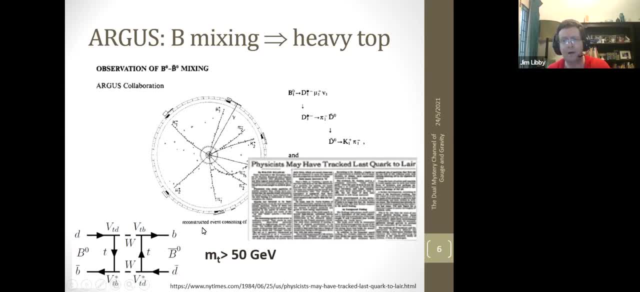 exactly. i think it's a quadratic dependence, but i can't remember um and and. so the limit's a little loose as you go to higher masses. but you know it must be a certain uh. you can't be too light, otherwise the rate would have been much slower. 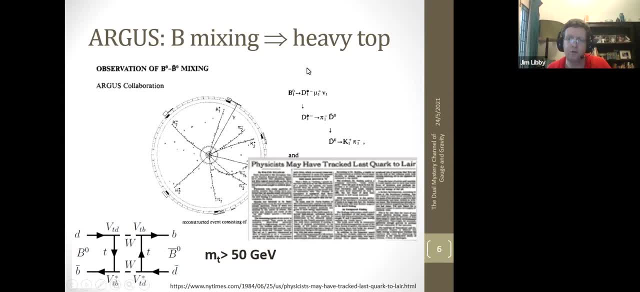 so this, this relatively fast oscillations, told us that the mass of the top had to be quite heavy, and that's what it does. it's all kind of these kind of precision measurements that are looking at loops. allow us to make some constraints on what the part unobserved particles in the loops might. 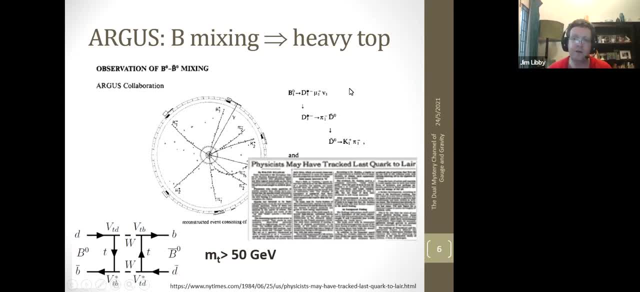 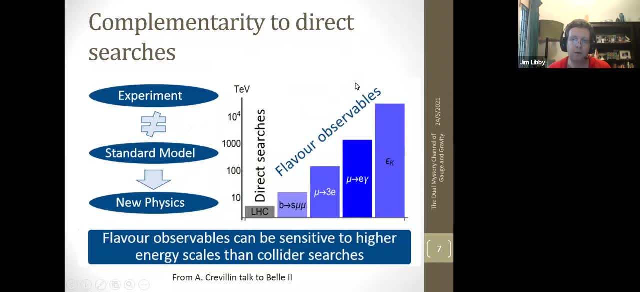 be, uh, influence the observable that we see, and that's very much the story of what we do now i see. okay, so this is the idea and it we like to refer to it as being complementary, because if you see a direct signature at the lhc, that's fantastic and it's a very clear observation. 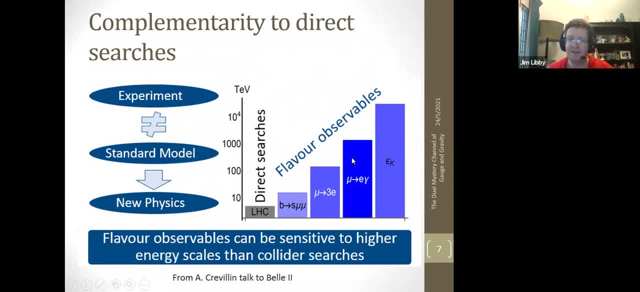 whereas you, if you're seeing deviations in a variety of measurements, it's it's also good, but the interpretation is not so straightforward, okay, so that's something else you must bear in mind as we we go forward. so the one here that really matters is this: to mu mu, which i'll start to talk about when i get to the present, uh, observable measurements: 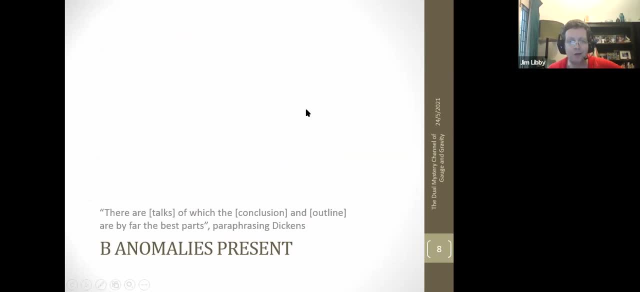 so this now brings me to the meat of my presentation. you can look at this quote which i paraphrased from dickens, telling you maybe the beginning and the end of most books and maybe talks are probably the easiest things to look at. but this is i'll. 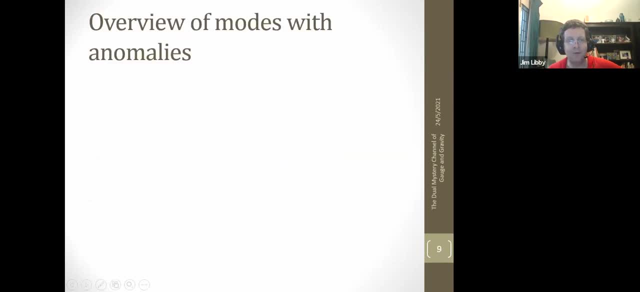 move on to my, my main course now. so i'll talk about the present. and there are really two types of anomalies in the b sector and they're related to two types of processes and it's quite important from the beginning to understand what the principal differences are between them. 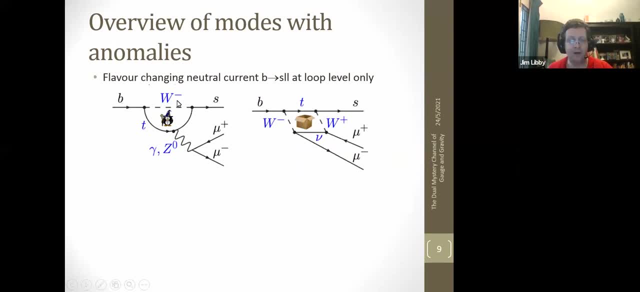 so this bs to mu mu or bs to ll type of diagram is a flavor changing neutral current where you have a b quark transforming to an s quark and this can only happen via a loop process. in the standard model the z does not couple between generations. 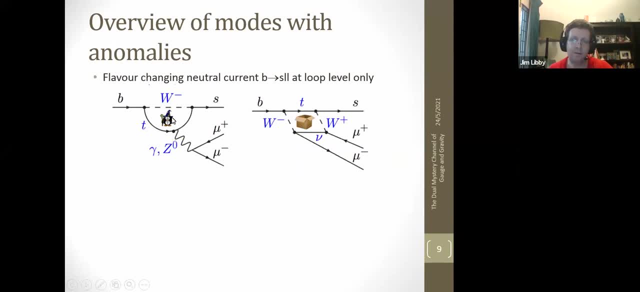 So you need to have this penguin loop, which I'll mention a little more about on the next slide, or you will have this box diagram where you have W and a neutrino, or you have the top quark, Z0 and photon here. So again, you're sensitive to all these different particles in the standard. 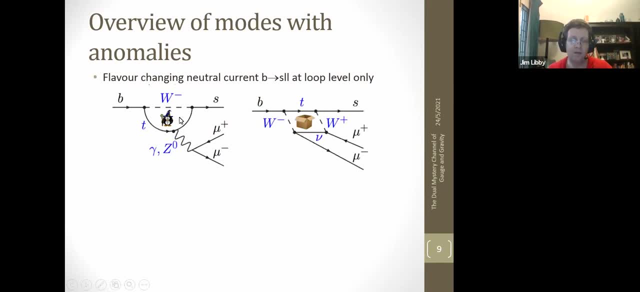 model within these diagrams. but the lesson is that perhaps we can substitute some of these particles with ones beyond the standard model and alter the observables that we see in these types of decay. So this is this loop process, which I'll talk more about in the next slide. 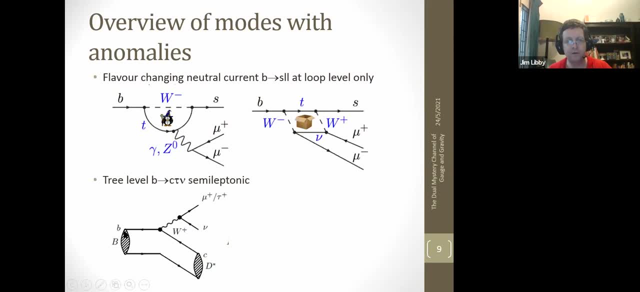 but there is another type of anomaly which is referred to, which has happened in actually the most common type of B decay, which is in a semi-leptonic decay. but it's the first time in the last decade where we've actually measured tau leptons in the semi-leptonic decays. 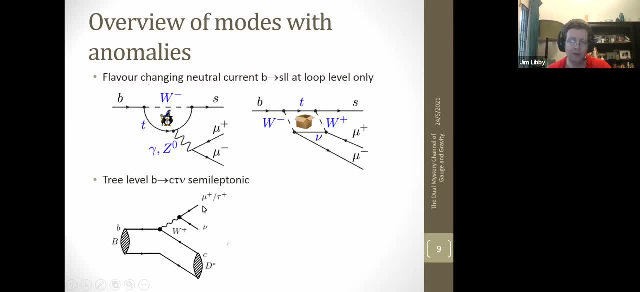 and, and these rates have found to be somewhat anomalous compared with what's expected when you look to semi-leptonic decays, where you have a muon on an electron as the lepton in the final state. So this is the most straightforward and most favoured type of B decay has a branching. 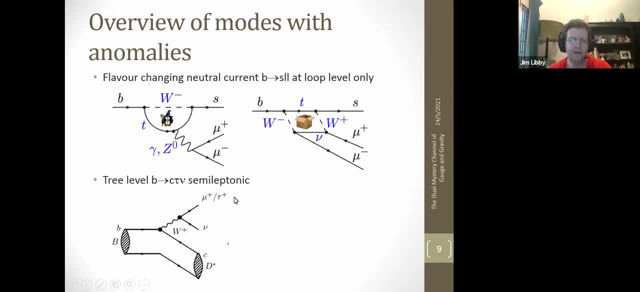 fraction of around- I think it's 11%. I should remember that Now there are pros and cons with these. Now, these loop decays, these loop diagrams, are great for the reasons I've already mentioned, that within these boxes, you actually reach mass scales that are very much higher than what you can probe directly. 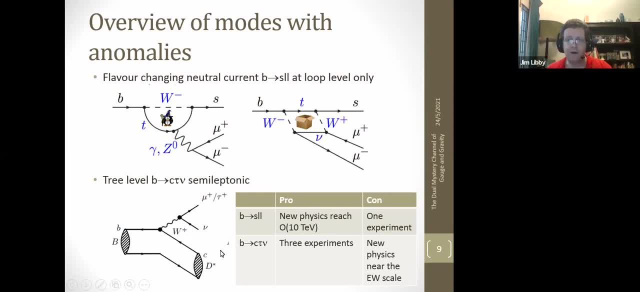 Whereas with this tree level diagram, if you're going to modify this with some new physics, that new physics has to be approximately around the mass scale we're already probing. so you then have to find ways to describe why we haven't seen this already in our collider. 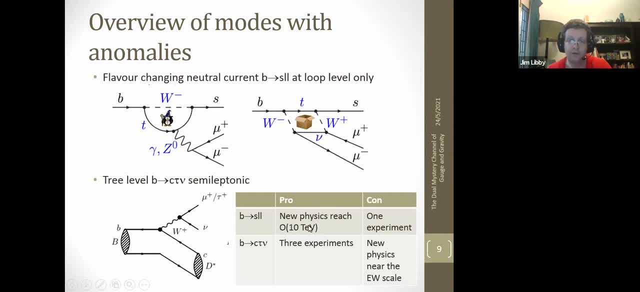 searches at the LHC, for example. So that's about the mass scales probed and that means the interpretation is somewhat more difficult for the B to C tau nu than these loop diagrams. Then there's an experimental difference between these types of anomalies, which I'll go through. 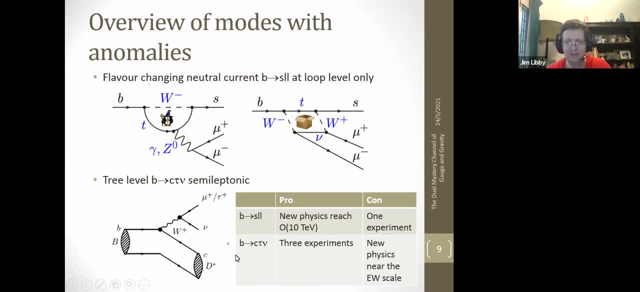 that this B to C tau nu has essentially been seen at some degree by three different experiments, whereas LHCb is the only experiment with precision currently to be able to say something meaningful about these Bs to mu mu. So a gold standard that we have in experimental physics is if you can corroborate your measurement. 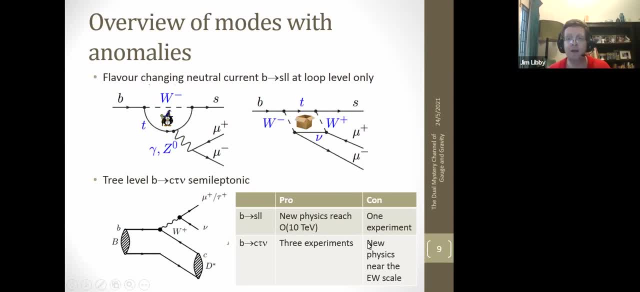 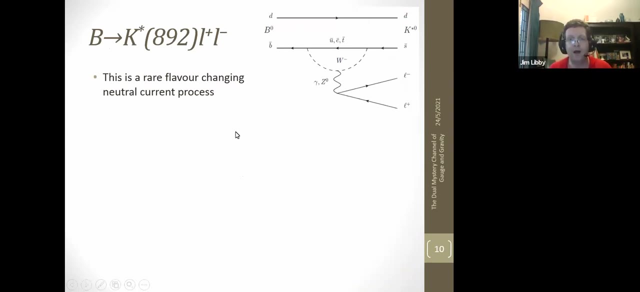 by more than one experiment. that reproducibility by another experiment is not yet there with the B2S mu mu anomalies. So, with that said, I'll talk more about this B2S LL or B2S mu mu, as is what LHCb has measured. 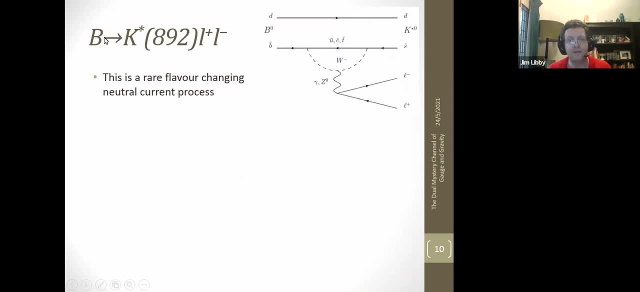 and the prototype for this. and the most interesting, I think, is this B to K star LL, where your strange quark is hadronized into a vector meson and you have this. penguin loop diagram is the dominant one, as well as the box, and here's John Ellis, who came up with the 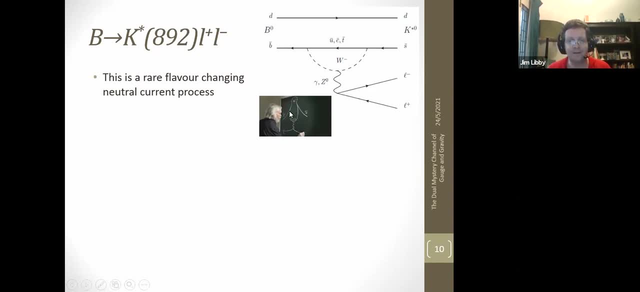 term penguin. I suggest you research. It's a rather amusing story as to how he came up with the name penguin. It was a losing or winning a bet. losing a bet: He had to to get the word penguin in his next paper and he managed to dream up that- this diagram- somehow. 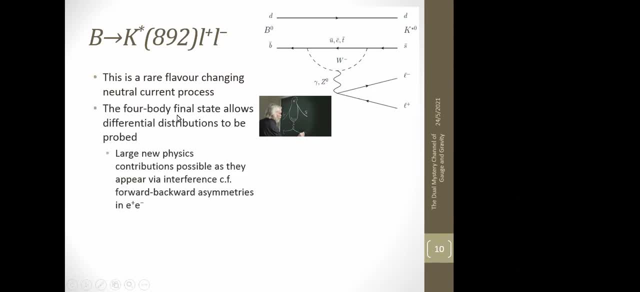 looks like this. Now, what's so nice about this K star LL is that there's a four-body final state and that means, because the K star decays to a K on and a pi on, you end up with many differential distributions that you can measure, which are very sensitive potentially to 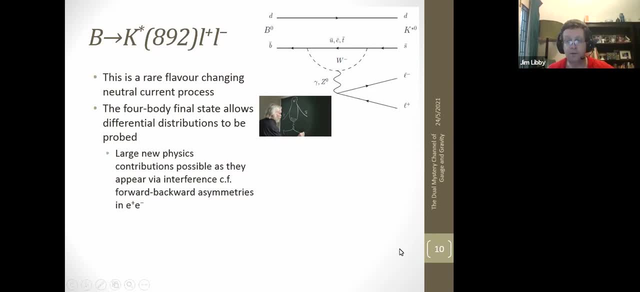 interference which may not alter the total rate that you might have, but could alter significantly these differential distributions. and history again tells us something here that if you look at the forward-backward asymmetry for E plus, E minus to die muons, for example, 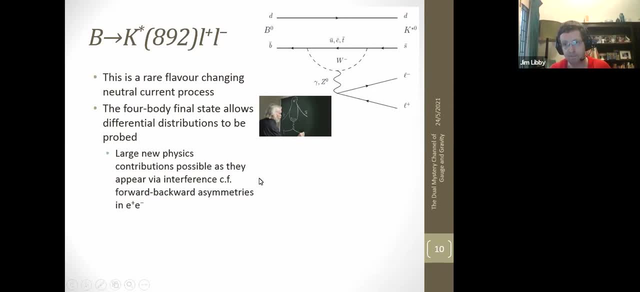 the overall rate is largely unaffected by the gamma Z interference, but if you look at the forward-backward asymmetry, there's a very large effect, even a long way from the Z mass. So this is what we're doing with these types of decays. 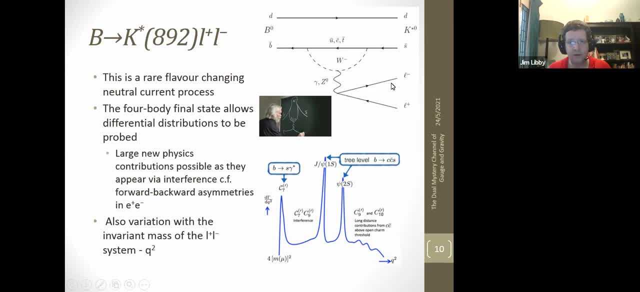 and also there's another degree of freedom that one has, in that the dilepton system and all the measurements are parameterized in terms of the invariant mass of this dilepton system. So here we're looking at the differential rates as a function of this invariant mass of the dileptons, and there's a rich structure here. 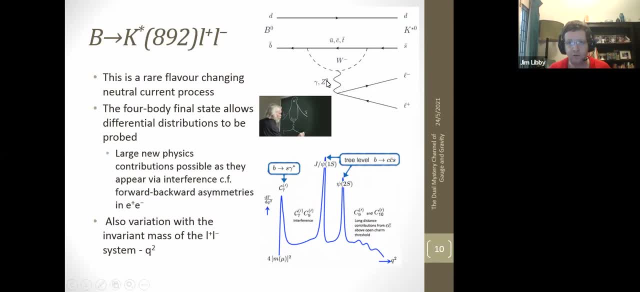 There's a very low mass peak which is related to the photon pole. that's here, and then you have these two peaks, which are not actually loop diagrams. they're related to decays of the Charmonium system and these are tree level. So these actually 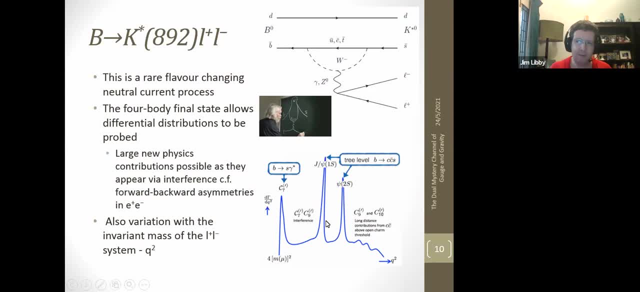 cause theoretical issues but experimentally are hugely useful because they're high rate control samples that we can use to calibrate the measurements. and then there are different regions. I'll talk more about these- C9's and C2's, and we'll come back to these in a bit. 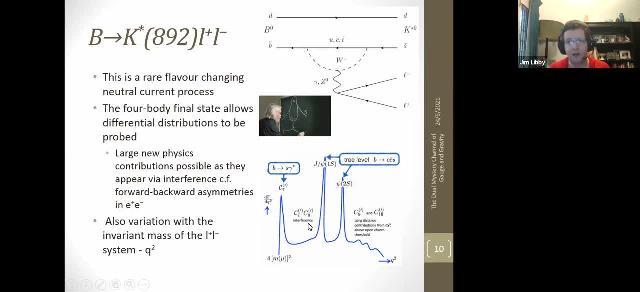 but the calibration and the ponding we're looking at here we're looking at, there's a really large variation. there so 10 parameters. These are Wilson coefficients, which are a way, in effect, to field theory, of parametrizing potential new physics contributions, And again, in different regions of Q squared. 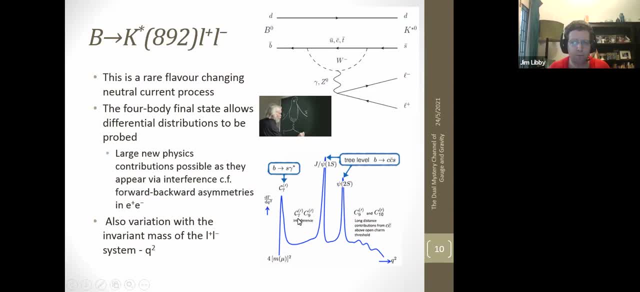 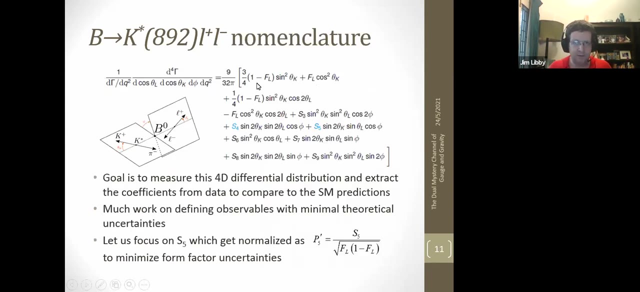 you're sensitive to different potential new physics operators. So this is a very rich phenomenology that's there in these types of decays for you to be able to study possible new physics effects. So just to define the nomenclature here because I'm going to show: 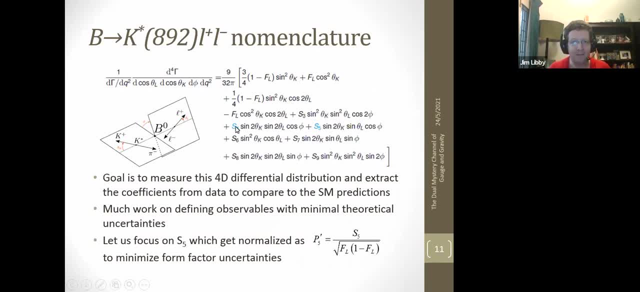 you the first anomaly, which has got a rather odd name, and it has to be defined in some way. So you've got this four-dimensional differential distribution which is in terms of Q squared and then the decay angles of the K star. So here you have the rest frame of the B. 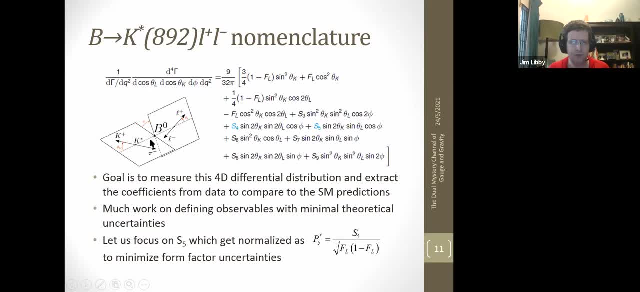 and you have a direction defined by the back-to-back motion of the K star and the dilepton system, And then, in the rest frame of the dileptons, you can identify a decay angle with respect to that direction. And similarly you can do that for 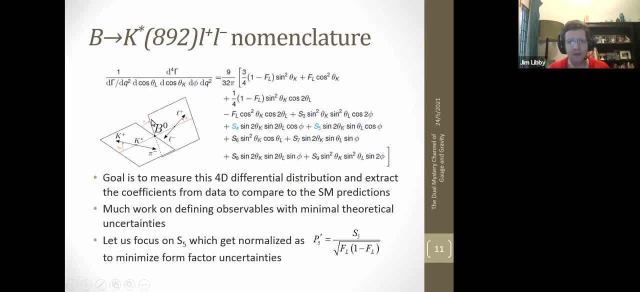 one of the particles coming from the K, And then there's some angle between the two decay planes. So with these three angles coupled with the Q squared, you can parametrize the decay. And this is this expression here, with these various dependencies. Now I'm just going to highlight here this S5 parameter, because that plays a role later on. 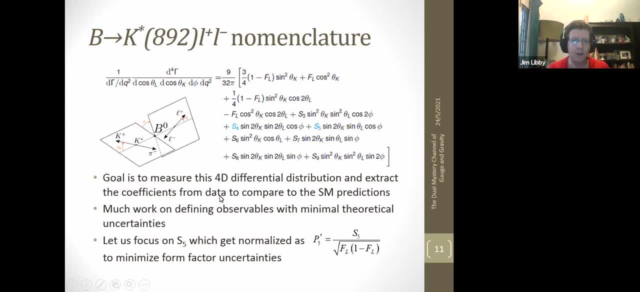 And you can predict all of these within the standard model. And a lot of work has gone on to defining observables that have minimal theoretical uncertainties, And one way of doing this was to sort of normalize them in some way or divide through by other parameters. So 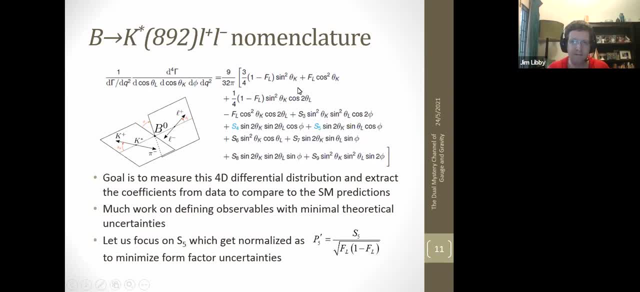 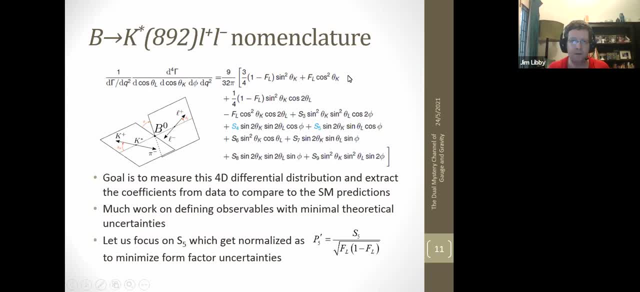 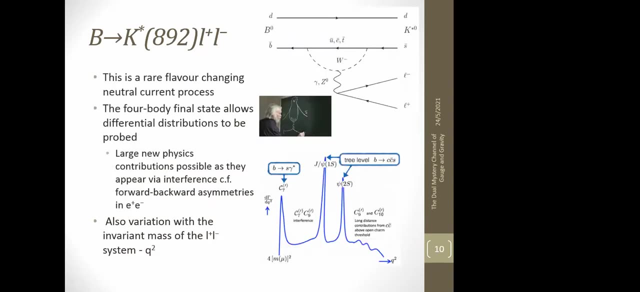 for these measurements. And this is this P5 prime. So, moving to the next slide, this is the first. Jim, sorry, I'm going to interrupt you. Sure, About your previous slide, the slide before this, Yes, So maybe you're going to talk a little bit. 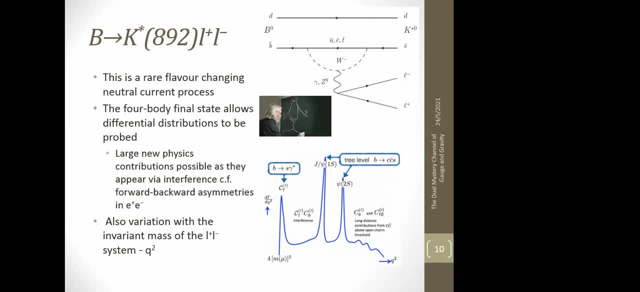 you're going to talk about it later, but I'm very curious to know. So you said that in this Q-square space itself you get a lot of this sensitivity to higher dimensional operators. So are some of these really interesting in the sense of they violate some standard model? 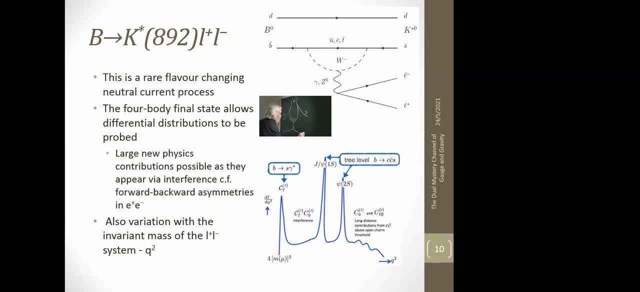 symmetries or have some very good signatures, or some of them could be more interesting than others. I think so. for example, this region which has dominated by this B2S gamma transition- because we actually measure B2S gamma rather well already- this is probably considered somewhat less interesting region than the region. 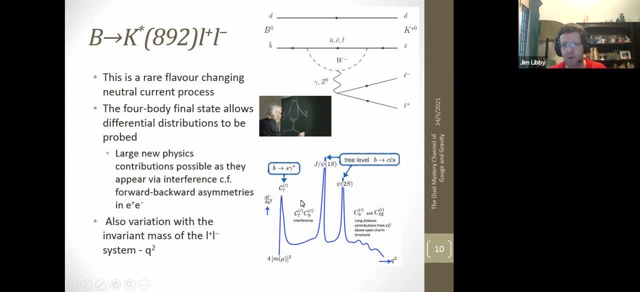 that lies in between that and the J-side peak, where you have this interference between these two different fork walk operators, And I'll show you why this region is in particular interesting. And then the higher Q-square opens up some different potential operators: the C10 operator, which I won't talk about so much in the future. but then there are long-distance. 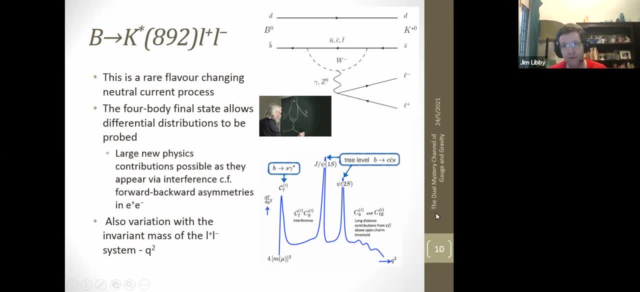 CC bar rescattering effects which are somewhat harder to control theoretically. So there's different theoretical problems here. So ideally you'd see a pattern of some regions either agreeing with each other or not agreeing with each other, And then you'd see a pattern of some. 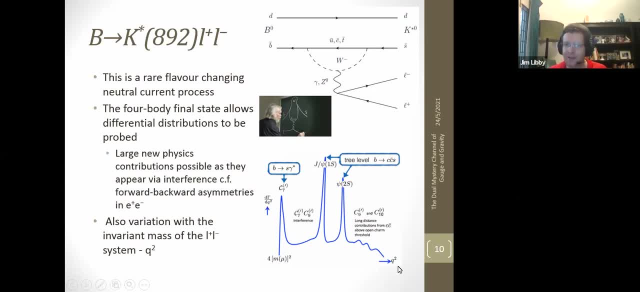 regions either the standard model not agreeing or all regions not agreeing, And that will tell you something, because you'll mean that different fork walk operators are influenced by new physics. Okay, so either one is two is three. you don't know until you make all the measurements. 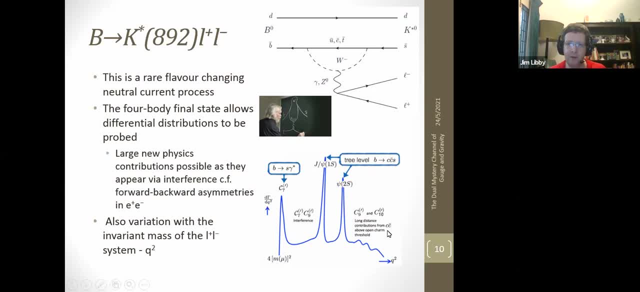 Okay, so that's the reason why it's interesting to divide it up in this Q-square. Okay, thanks, Does that answer your question? Yeah, yeah, Okay, thanks. So you're saying the fork walk operator sector can be probed at least by this pattern? 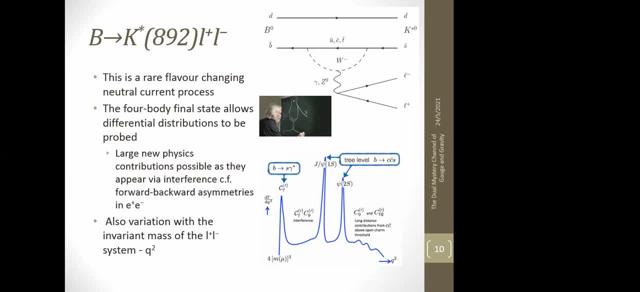 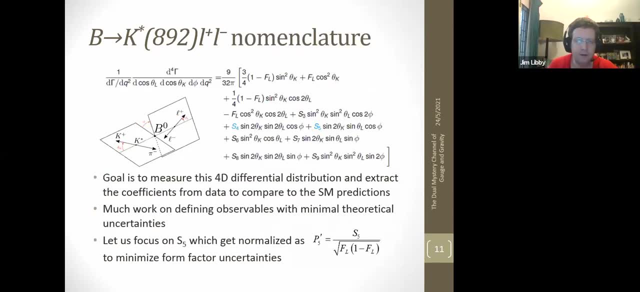 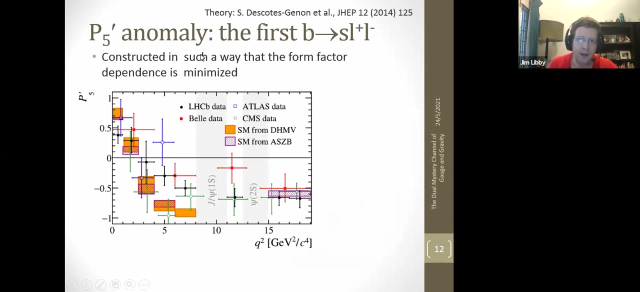 And I will show this in a bit when I come to the interpretation. Okay, Okay. so yeah, I'd introduced this rather ungainly nomenclature that's there to measure these differential distributions, And now the measurements themselves came in 2016,. so it's about. 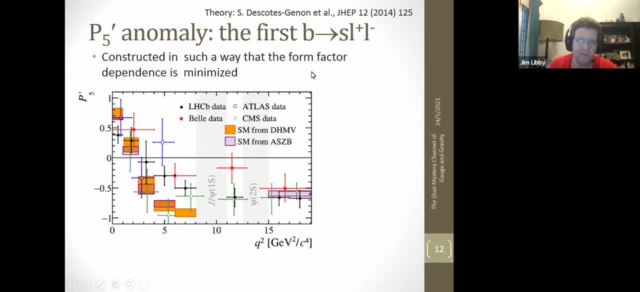 It's about five years ago now, but this is the paper where this P5 prime variable was proposed And this very messy plot. you should focus first of all on these black points, which are the LHCb measurements of this P5 prime variable, which is this coefficient of this angular distribution. 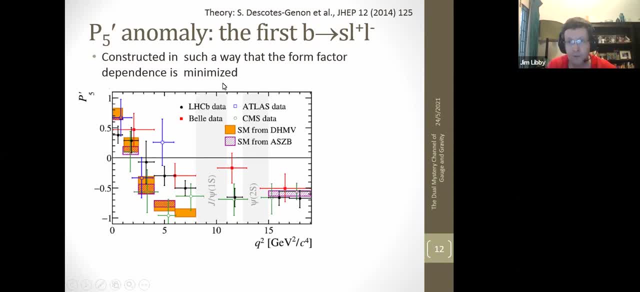 So they fit this angular distribution or this four-dimensional distribution and extract these coefficients and then just measure them as a function of Q squared. And there's this run of points lying between this photon region and the J psi which are all well above the standard model predictions which are given here in orange and purple. 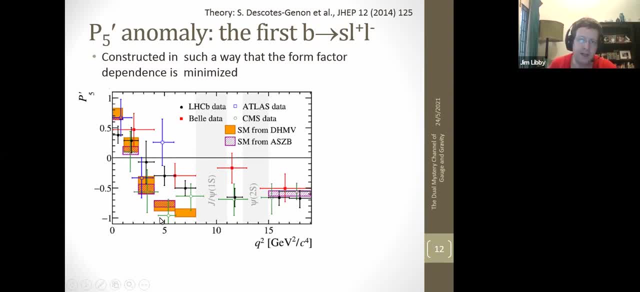 And this depends on which hadronic parameters you're choosing. You can decide how you want to parametrize your hadronic form factor, which is an unknown, And this is consistently high. Now there are other measurements coming from ATLAS and CMS, and also from Bell. 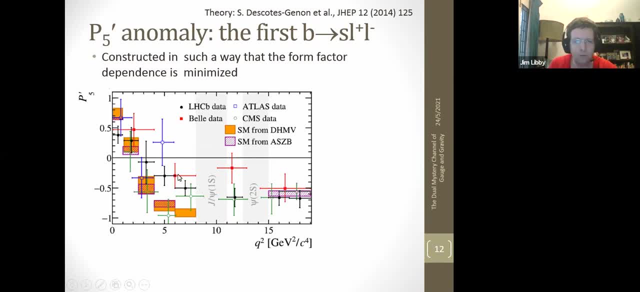 but they do not have the statistical precision And it's all rather messy because they choose different regions of Q squared to make their measurements. But you see, Bell And ATLAS and LHCb are consistently high. The CMS fluctuates downwards. They seem to agree with the standard model. 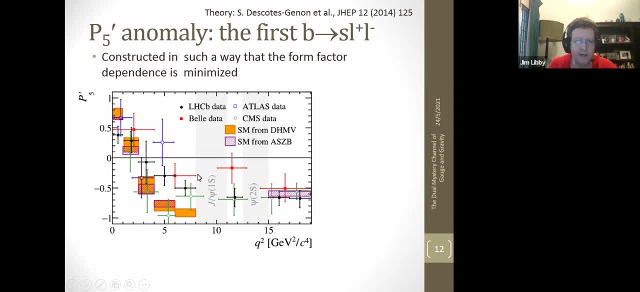 But given all the precisions- and I'll show global fits later on- essentially this comes out to be more than a three-standard deviation from the standard model. But because of the theoretical uncertainties here, combined with the fact that it's not as clean a measurement as some of those that I'll show, 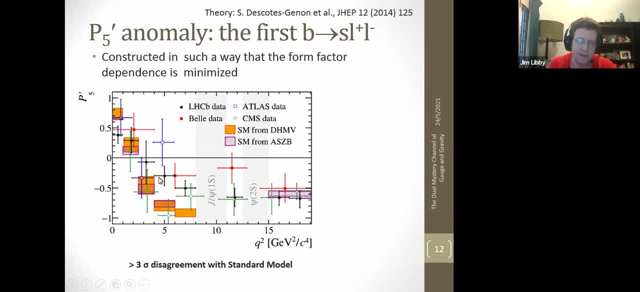 later on. this is extremely interesting and has been for some time, But people are always unsure about whether it's the theory or there's only one measurement. But LHCb have done a very thorough job with this And you see referring to my answer to your question. 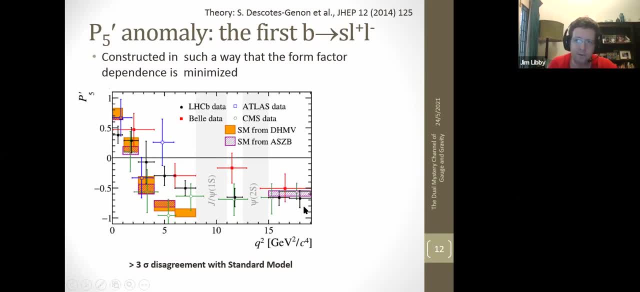 that, at this high Q squared, there seems to be good agreement between the data and the standard model prediction, And it's just in this interference region which would then be telling you something about where the what the new physics might be in terms of the operators. 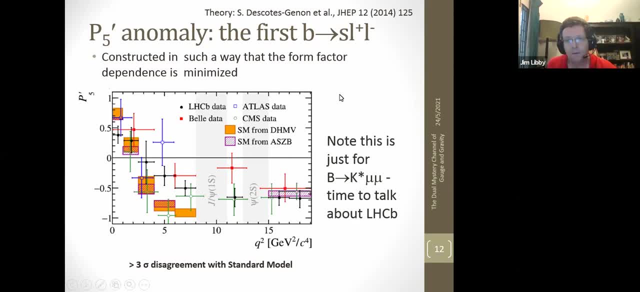 And you'll see that when I show the fits a bit later on. But there's an important point, moving to the experimental side of things here, that this is just for muons, And so it's a good time, given there's probably not a huge amount of familiarity with it. 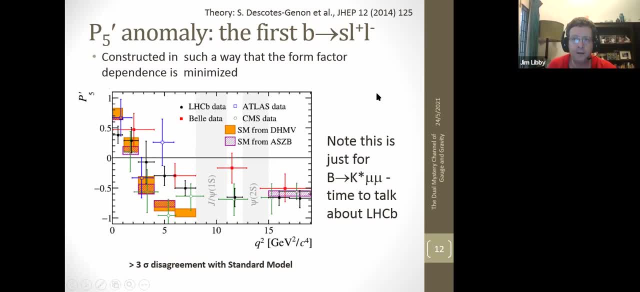 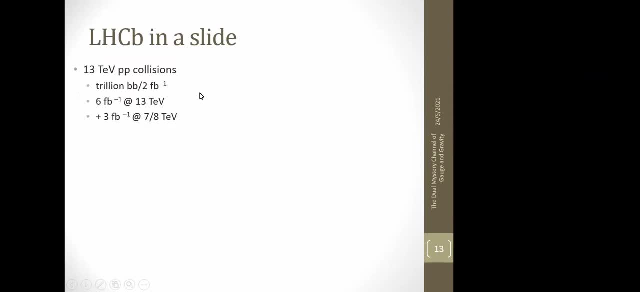 to discuss the LHCb experiment in a single slide. But I'll just explain why it's the case that they're just looking at muons here. So the LHCb, Hello Jim, Hi, Hi Harry, Yes, Hi Jim. 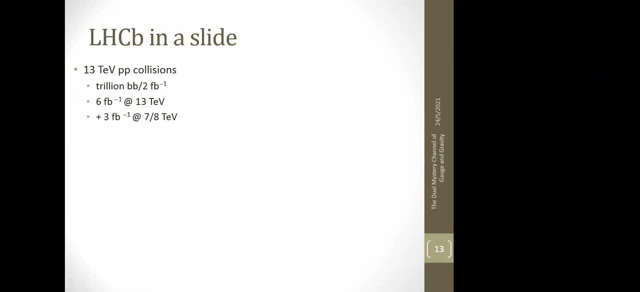 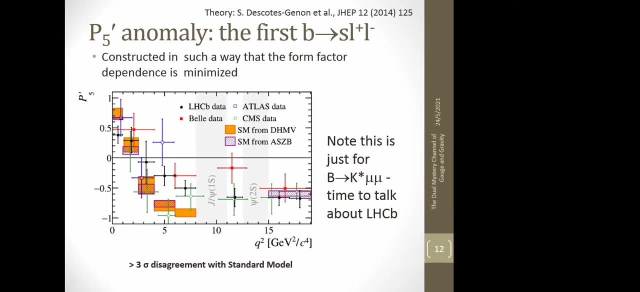 Hi, hi. Can I ask you a quick question on that previous plot Sure? So I was just wondering. it seems like there is some tension between the LHCb and the CMS data, is there not? Yes, But when the global fits are done- and I'll show you the results of that later on- 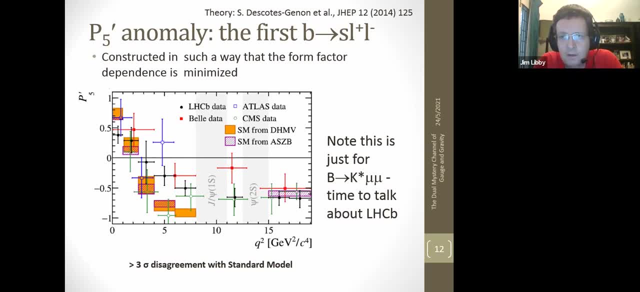 given the limited statistical precision of CMS compared with LHCb, it doesn't lead to a very large pool. that's a problem for those fits. So there is some tension, but it's a few order of two standard deviations. It's not more than that when you put everything together. 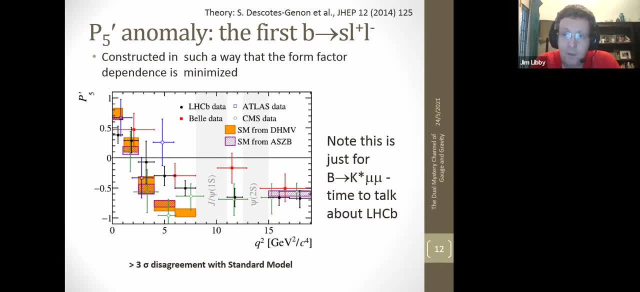 So it's not significant at the moment. But bear in mind there are going to be much better measurements, particularly from CMS, at some point in the future, because they've got this large part B data, So it'll be interesting to see how that develops. 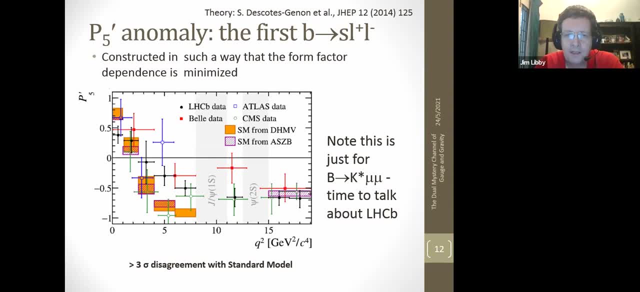 Now, I'm not an expert on these measurements. I know the LHCb people feel that they may not be quite as robust as in some of the things that they've taken into account, But I wouldn't want to speculate further on that. 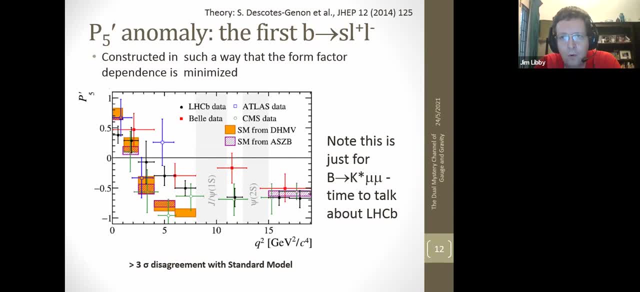 I think that's only time. we'll tell when there's more information. Yeah, I guess you know it gives one pause because CMS seems to agree with the standard model prediction. So I don't know if it counts for something. but 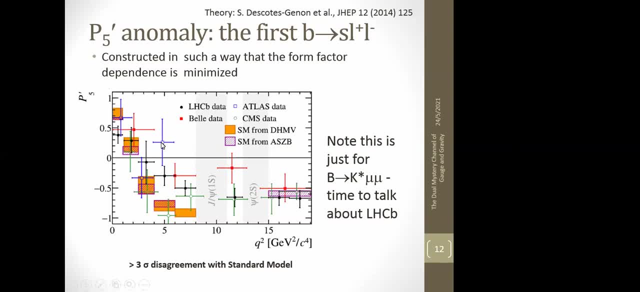 Yeah, On the flip side, Srihari, you can look at the Atlas point and say, well, yeah, I don't, you know. Well, if you're a conservative and if you want to take a conservative view, then you would focus more on the CMS agreeing with the theory prediction. 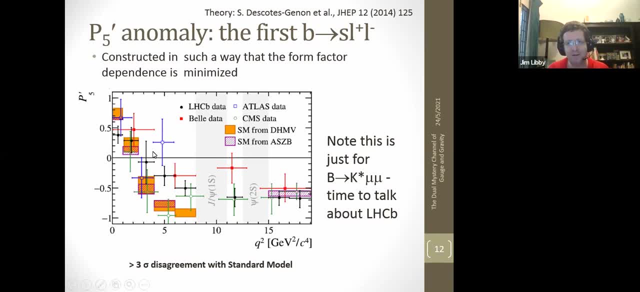 Okay, Well, I'm a frequentist, So each point is only as good as its error bars, Yeah, So I'll show you the global fit, And there I think it's convincing that something is going on Right. So, But let's talk about the other observation, which 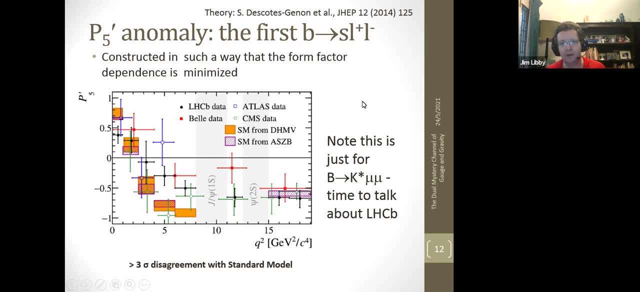 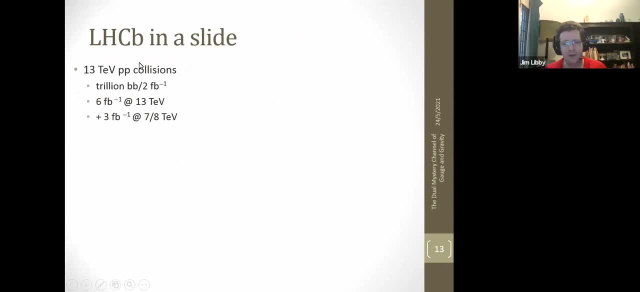 Well, I'll talk about the experiment and I'll talk about the RK and RK star. So LHCb is operating with these 13 TeVpp collisions And the reason for that is that in every two inverse femtoband of integrated luminosity. 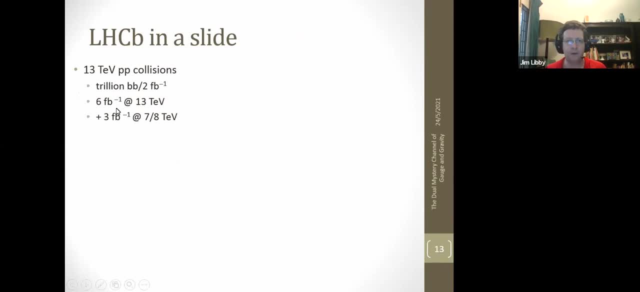 one gets a trillion- 10 to the 12th- 12 bb bar pairs and they've collected so far nine inverse vector bands of data, some of it slightly lower energy, where this number would not be quite correct. but they have produced many bb bar pairs at their collision point and collected many of them, and they are a forward geometry. 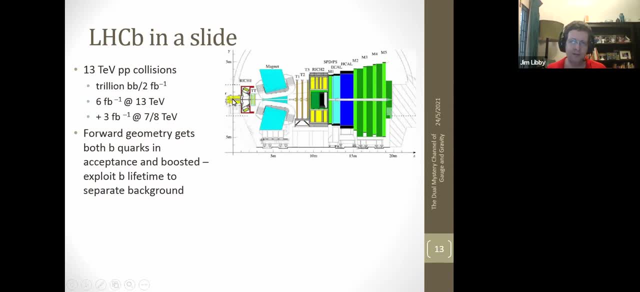 experiment at the lhc. so the collision point is here on the left hand side of the schematic of the experiment, and the reason for that is that the b quarks primarily get boosted into the high rapidity region which is being instrumented here. so you get both b quarks within this acceptance. 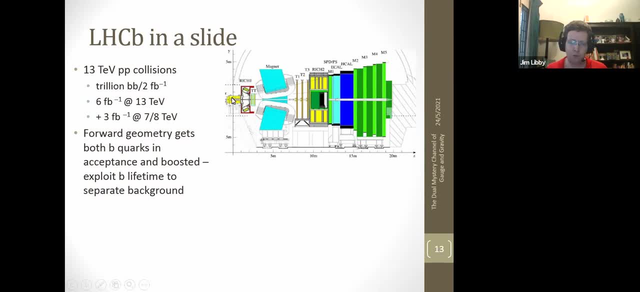 so this increases your efficiency further. there's also a huge advantage of having your b quarks boosted, exploiting the long lifetime that they have of around 1.2 picoseconds or so. it means that the vertex of decay of the b quarks is going to be a little bit more efficient and the b quarks are going to be a little bit more. 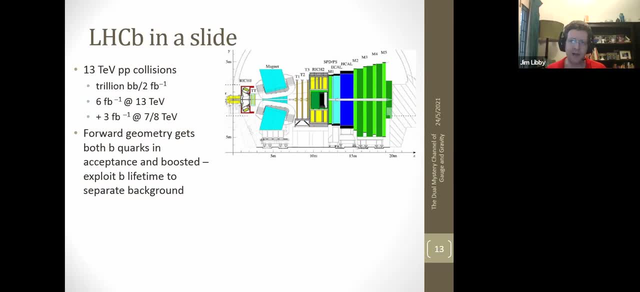 efficient and the b quarks are going to be a little bit more efficient and the b meson is well displaced from the primary vertex and they can sort out background very readily using a high precision vertex detector that they have. so it's also there for time dependent cp violation. but i'm 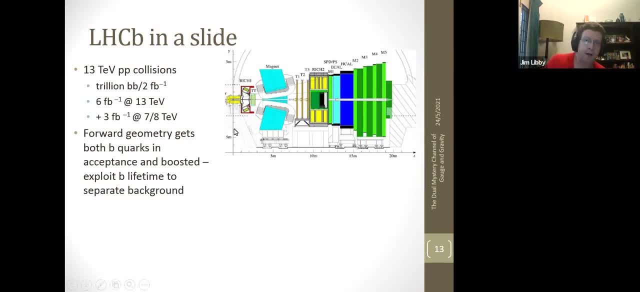 not talking about that today. that's an entirely different topic, but so so this was designed from day one and gives it a competitive advantage over a cms and atlas for doing b physics, and the other reasons for that are they have ring imaging cherenkov detectors to cleanly separate pions and kaons over a momentum range from around 1 to 100 gv. 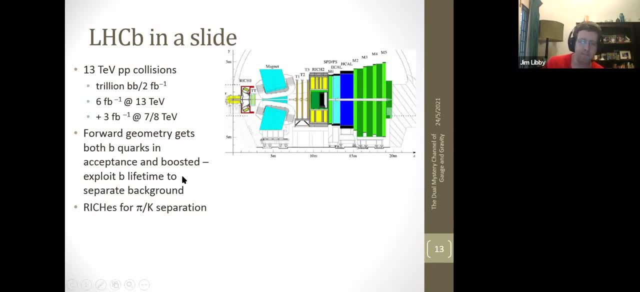 which is important for identifying final states of interest. and they also design their trigger just for b physics. so their full trigger bandwidth is dedicated to collecting not actually just bees. they also collect charm quarks very. charm decays very readily as well. but why just the muons is? 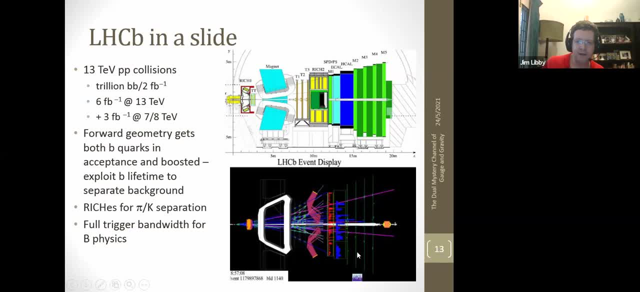 somewhat, somewhat clear now, and if i show you an event display here. so, um, they do their tracking with the dipole magnet. so you see the tracks are curved here. they get kicked as they go through the dipole magnet. um, but there are many of them. it's a pp collision. there is high multiplicity. 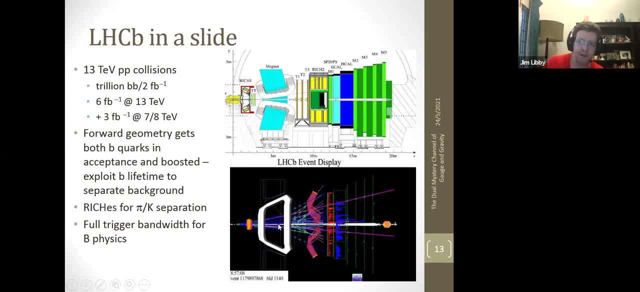 environment, even though they detune the luminosity at lhcb. so it's a very busy environment downstream here and this red here is their electromagnetic calorimeter, which is extremely busy, and they're very busy with lots of hits from photons produced from pi zero decay, for example. then here they have. 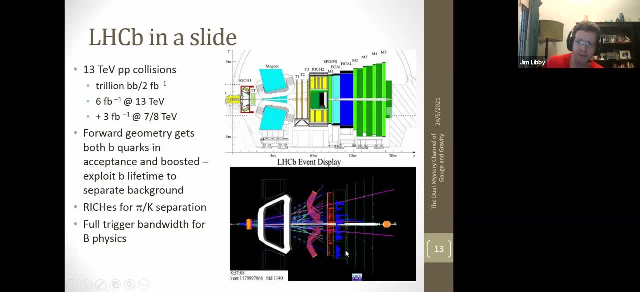 a hadron calorimeter which is largely used for triggering. it's not used for any energy flow type measurement that you might be used to from the other general purpose detectors. but these two purple lines here, these are the two muons. so they have this muon filter system but they have iron. 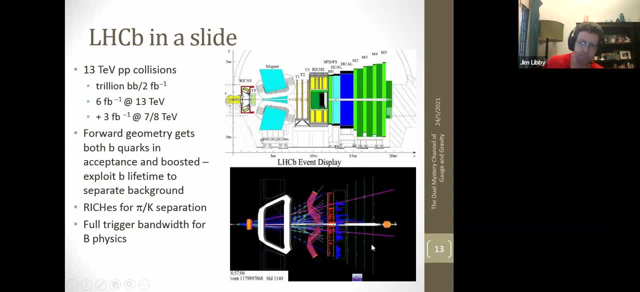 sandwich with their muon detectors. in between gas detectors and uh nwpcs and rpcs are there and these allows them to identify high momentum muons coming from bdk very, very readily, and they can then track them through their their precision tracking and they'll get their vertex position. 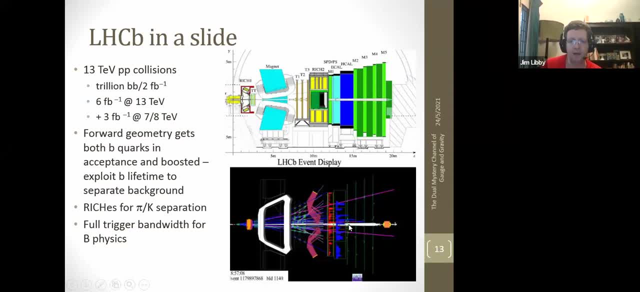 so this is a bs to mu candidate, actually that i'm showing. but the problem is that to identify muons is highly clean, whereas this trying to identify electrons in this high multiplicity environment here is very hard and um. that's why these angular measurements have not yet been done. 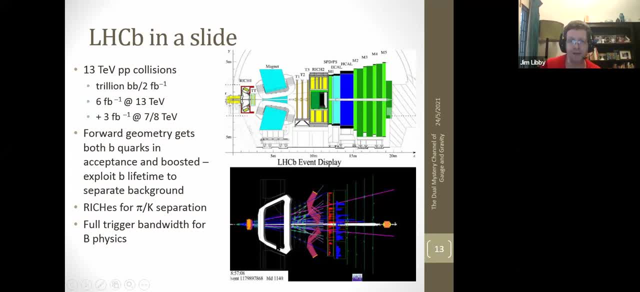 and they're not going to be made with electrons, for example at lhcb, and i'll talk more about why that's important. as i go through the talk, i'm going rather slowly here so i need to speed up- isn't the electrons? overall, some q square measurement has been done. 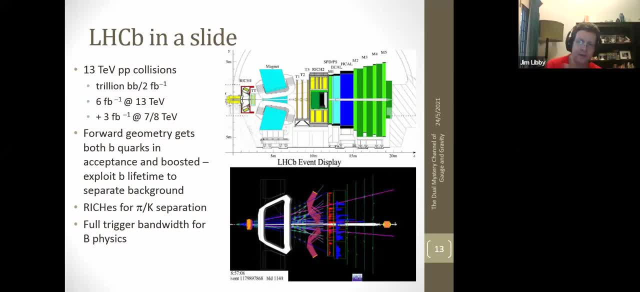 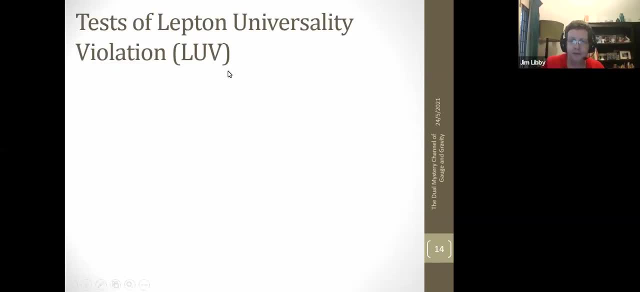 if not the differential i, i i'll come. there's the next couple of slides, so i'll talk about this. yeah, so now i move to these recent measurements, these tests of lepton universality. so they're really updates of older measurements. but what's being measured here is just a ratio of the differential branching fraction as a function. 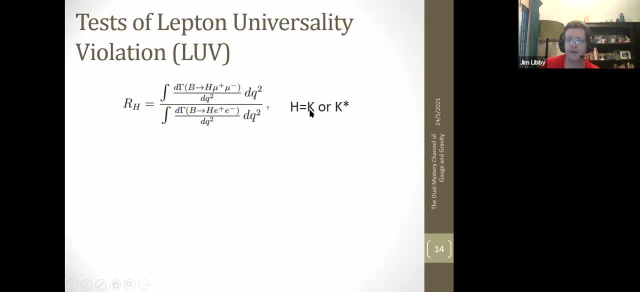 of q squared integrated over some q squared range, and this is done for both- uh, pseudo scalar and vector k star, done for both types. now this ratio is extremely robust theoretically. it's very, very clean. it's got like a, it's one to a few percent. it's got very small theoretical uncertainties. 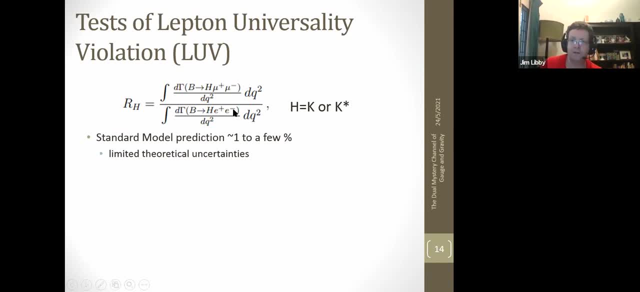 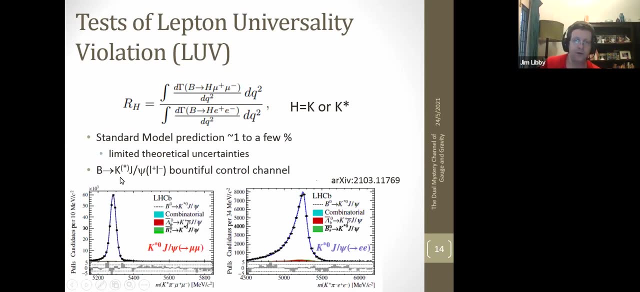 involved with it, because the uncertainties to do with form factors just drop out in this kind of ratio measurement. it also has this control sample which is coming from this uh b to s cc bar, final state where you have a k or a case k star with a j psi, and these are data plots. 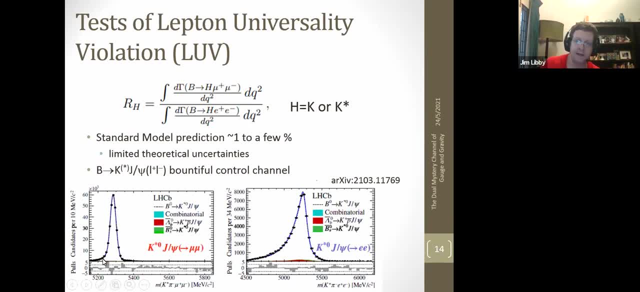 they look like monte carlo plots, but these are actually the data that lhcb have in these control modes where they can separate out these b decays using the lifetime and the time, and then it's just whatever they see that reconstructed as a k star and two lepsons. 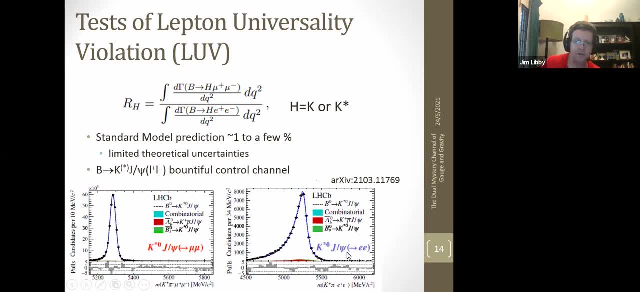 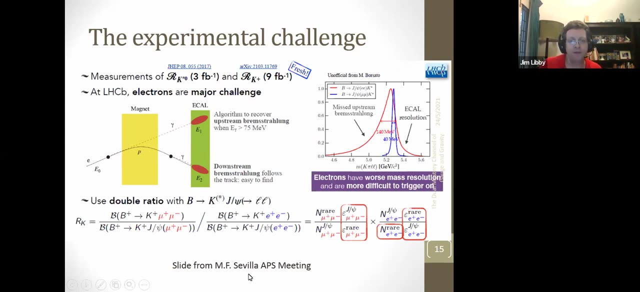 is pretty much a, b, but as you can see, the electrons on the right hand side is a much broader distribution and also the scales are different on these two plots, so it gets even more stark than this. so i've just borrowed a slide from a recent talk by manuel sevilla at the 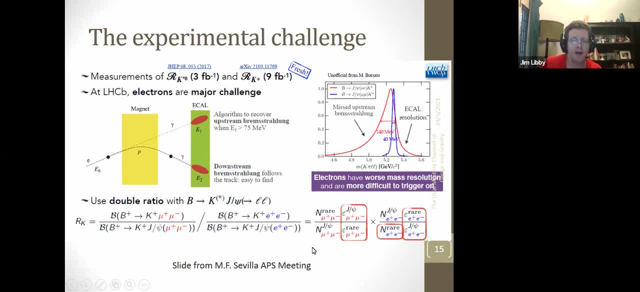 aps april meeting was in pasadena, um, and here he's showing how hard it is to reconstruct these electrons at lhcb. so, as i said, they have this dipole magnet so as your electron goes through it gets a big kick from which you actually measure its momentum, but it can. there's also a significant amount of material, both. 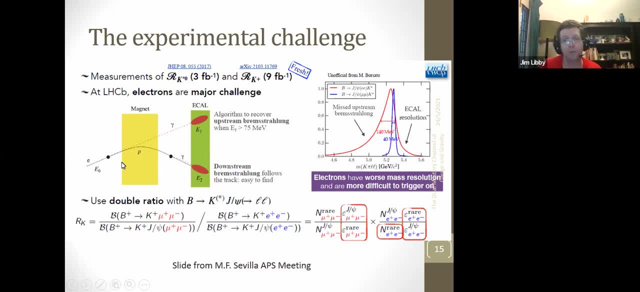 in the silicon detector- the rich detectors- there's a vacuum chamber in which the silicon sits, so there's a significant amount of material- what we call radiation length- before the electromagnetic. so there's a large chance of bremsstrahlung and- and these photons from bremsstrahlung have to be 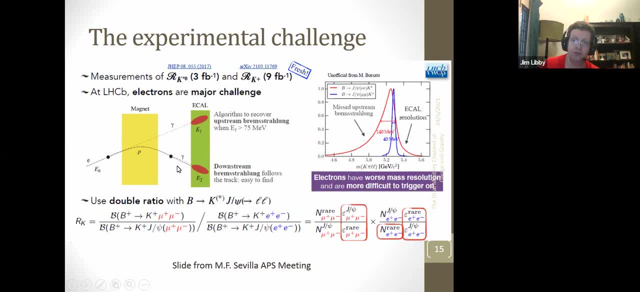 added back in to try and improve your resolution. and- and in this plot here it shows: even with the best bremsstrahlung recovery that they have, they still have a long tail going to low values of the b mass because they haven't captured at all. there's a lot of energy lost, so it leads to. 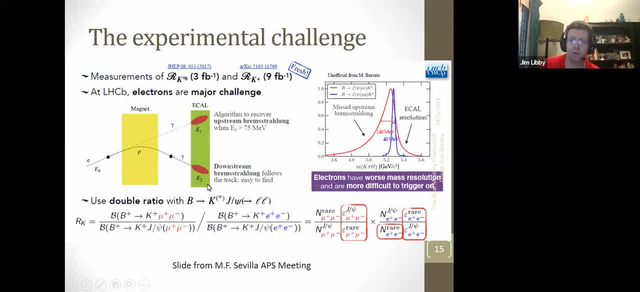 a very broad distribution and it also leads to problems trying to trigger because you lose pt or energy from these clusters and they're triggering on these uh ecal clusters. i can't go into the details of the trigger, but it affects their efficiency, so their efficiency is much lower. 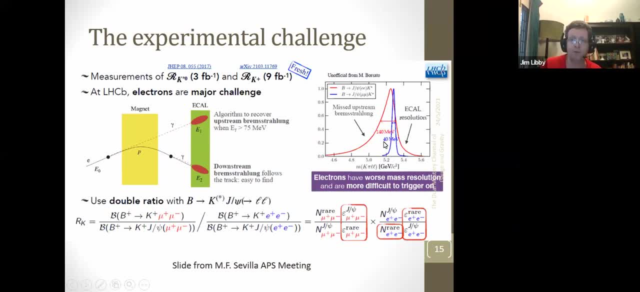 for electrons and the muons. so they have these double problems of efficiency and resolution being much worse. but they somewhat overcome that because they use this control sample and they take a double ratio. so issues with the trigger efficiency and, uh, largely the trigger efficiency and the reconstruction efficiency cancel out in these double ratios and they make a lot of progress in. 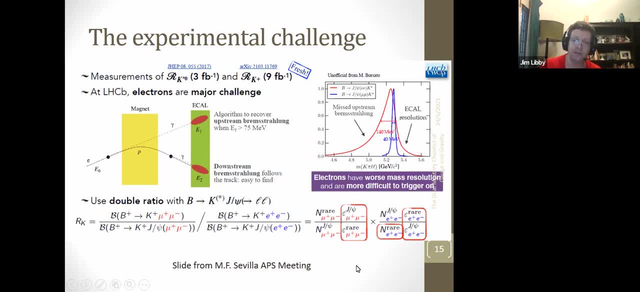 they measure this R parameter as this ratio of ratios essentially, So a lot of the experimental effects drop out. So this gives you significant confidence in the measurement because they have this control sample. No one would believe this was done on Monte Carlo, for example. 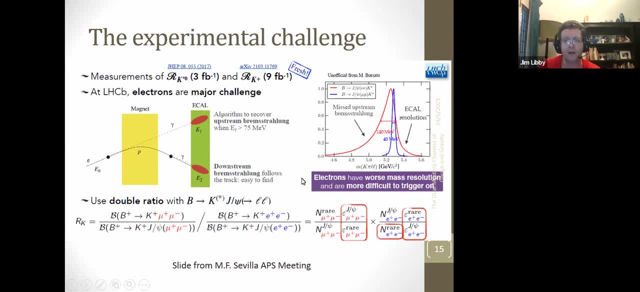 But because they use this data control sample, it's quite robust. And then the two measurements they have in the new one is with their full data set. So be aware that they're going to update their RK star at some point in the near future. Hopefully it's been a long time coming. They. 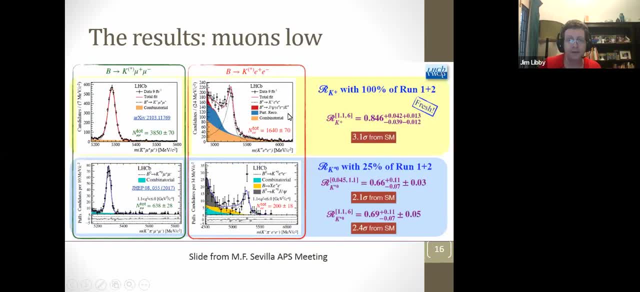 stopped taking data in 2018.. So these are the results. On the top is the RK. So this is where you have a K to mu mu or a K to EE. But you do see now when you have the much rarer loop process. 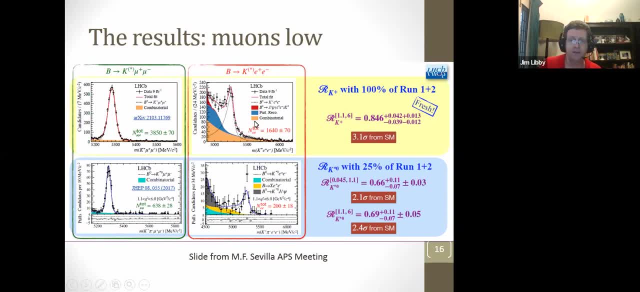 rather than the J psi. there is significant background underneath the electron sequence. So you can see that there is a significant background underneath the electron sequence. So you can see that there is a significant background underneath the electron signal at least. And then they have to understand this electron background. Some of it is: 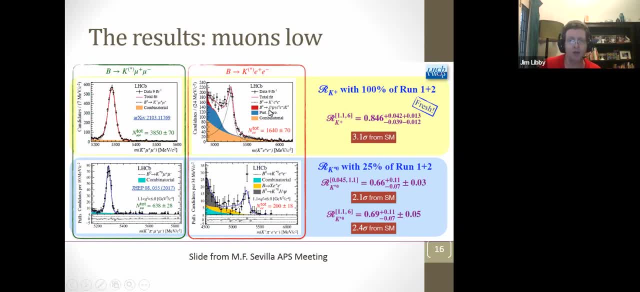 combinatorial which can be easily fit, But some of it is partially reconstructed, decays of one type or another And that's somewhat harder to model. But they've done a careful job. But they have half the number of electron events compared with the muons. Sorry, a very stupid question. What is 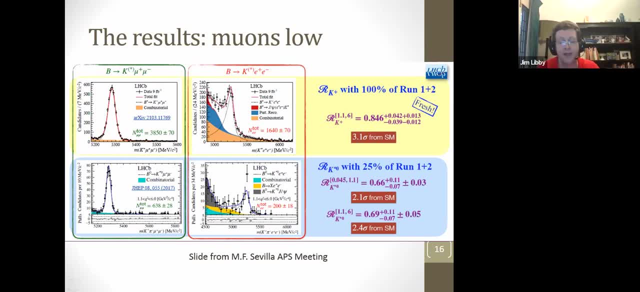 this x-axis here, Sorry. the x-axis is the invariant mass of the final state particles, So it should peak at the B mass, Okay, So it's just the B mass. It's just the B mass, Okay, Thanks, Yeah, Sorry, That's my complacency. I look at these plots. It's just the mass of the B. This is where. 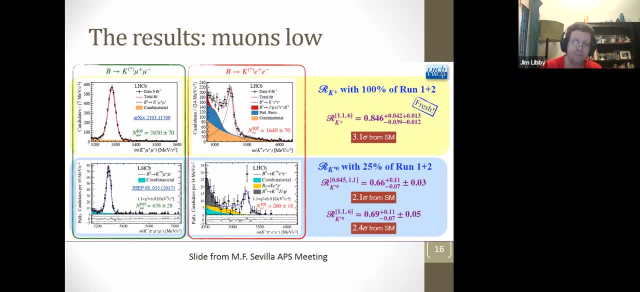 primary plot that they always show when they're separating a signal. But it's also remarkably clean on the muon side. There's very little background. So these measurements all are low for the muons compared with the electrons. So it's just the B mass. 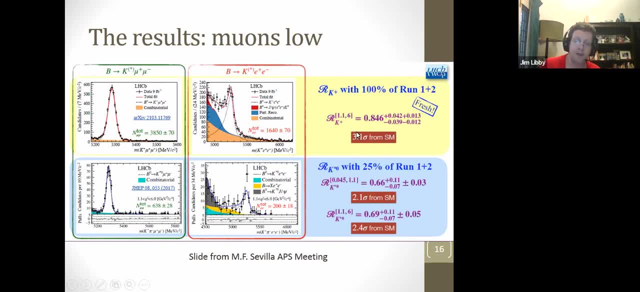 And this one that was released near Morion is now the first one to creep over three standard deviations, And the standard model prediction essentially has limited uncertainty in comparison. So this is now a three standard deviation discrepancy, Jim. So yeah, Srihari. 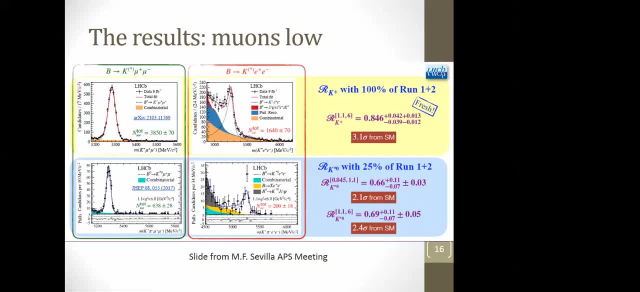 Yeah, So the JSI being used as a control sample, So you need to extract, So you need to extrapolate a little bit out of the JSI region in order to make that RK measurement in this double ratio. But is that, you know, like clean? I mean there's no real, you know. 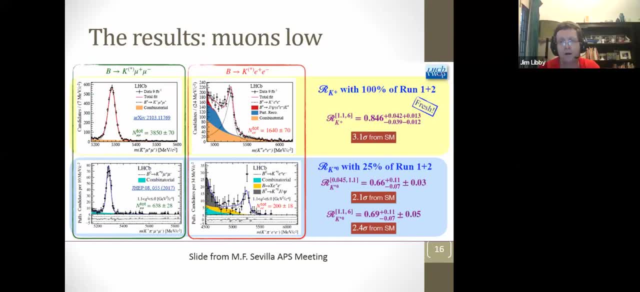 like uncertainties coming from there, There are uncertainties. So, if you see the systematics, the fact that the momentum distribution of the dileptons coming from the JSI does not exactly match that coming from the signal, But you do all these corrections. 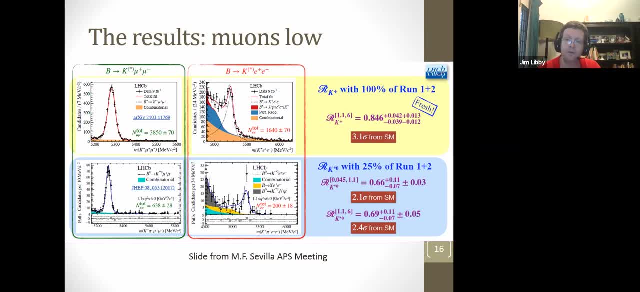 You have the same bins of the momentum, right, So you break down that control sample to best utilize it as you can. But there is an uncertainty that comes from this. But that's very understood and you know. it's like it's not a cause for worry or anything. 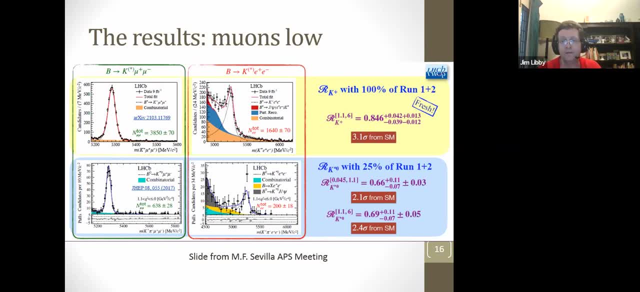 It's, I think, pretty well understood, But it is a cause for concern. that well you know if something has gone wrong here. but i just like to emphasize that the electrons are actually. the electron mode completely agrees with the standard model prediction. it's the muons that. 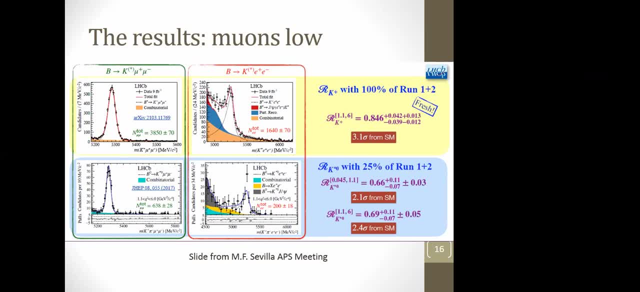 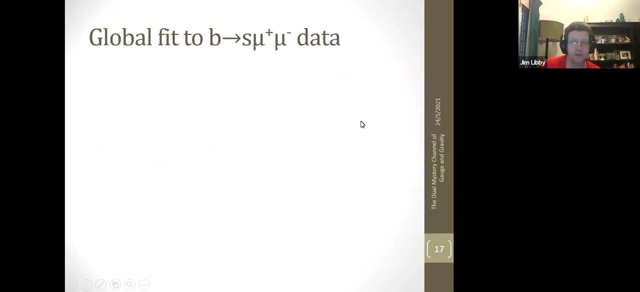 are low. so so it's. so it's kind of you know, if it, if it was the electrons were high, then you'd be like, yeah, maybe, but of course this needs to be corroborated either by atlas, cms or, in the future, bell 2. okay, thank you. so all of these measurements can then be put together and then there's a big 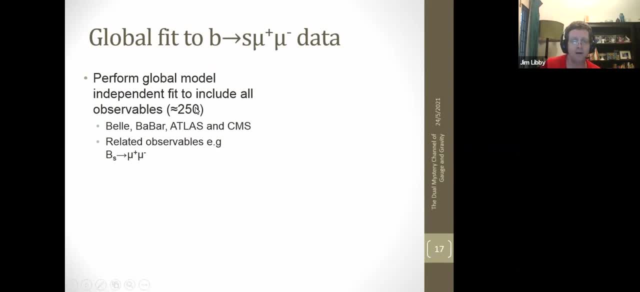 industry in doing these global fits. and there are now many, many observables, because you have all these double quadruple differential distributions in in k star of mu mu in particular. but you can throw in everything coming from bell, bubar, atlas and cms, as well as from lhcb, and there's things. 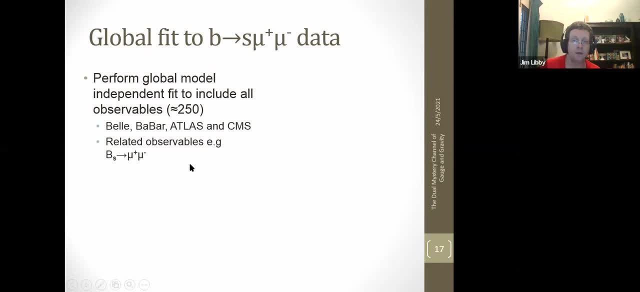 like bs to mu mu, which is the same four quark operator involved, and you can then fit all of this in terms of different combinations of of these four fermion operators, and this is always parameterized in terms of these wilson coefficients. now, what's shown here is not the wilson coefficient for c10 and c9, which is 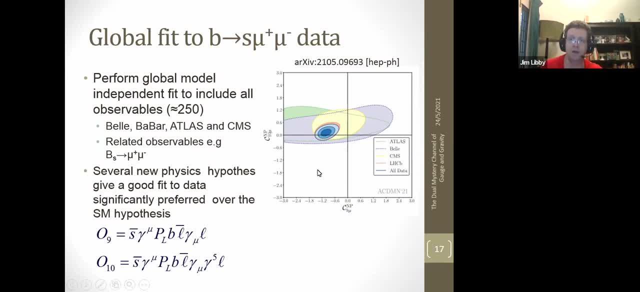 basically v minus a theory here. this is just a deviation from v minus a standard model. um, this is a new piece which should be coming from the new physics. now, if you fit all of these observables together, you get this blue region here, and if the standard model were correct, you'd get something here at zero zero. 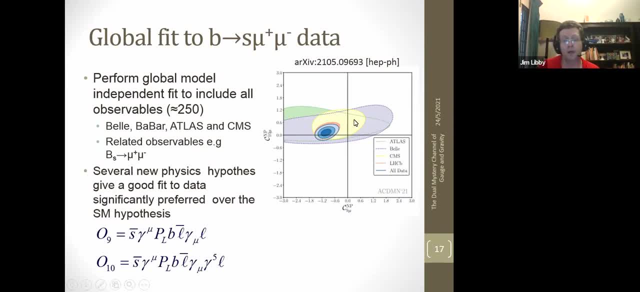 and the authors of this paper uh, say this is a six to seven sigma standard deviation, and then there are assumptions. in this you're just using these two operators, but if you go and look at this paper, there are many permutations that they have and they're not going to be able to. 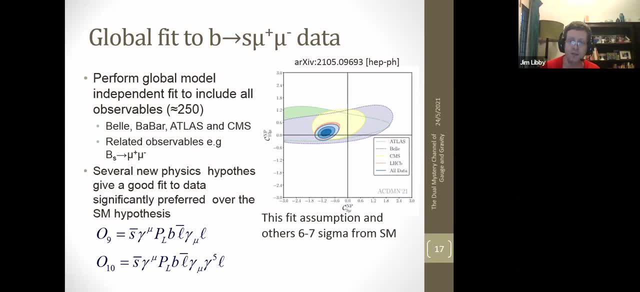 give you the same kind of the same kind of the same thing. but you can look at a number of these and they show a number of different kind ofometry that have the same kind of that has been found and then they'll all have the same kind of the same probability that they have and 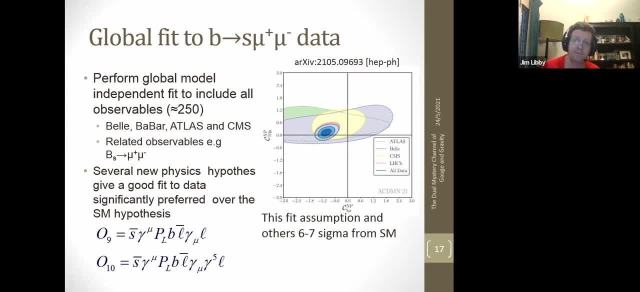 many of them show significant deviation, but of course you'll need more and more measurements to pin down which is the most favored, but this is one that's very clear. i think this has the best chi squared of all of them, and but i also want to emphasize the dominance of lhcb here. 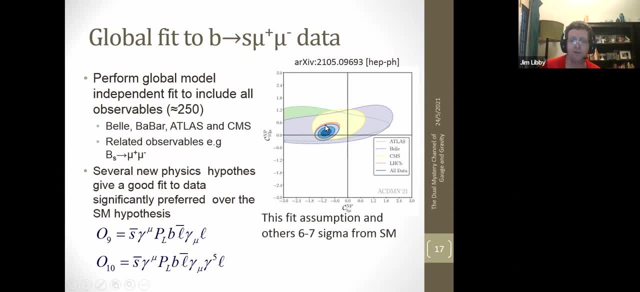 so lhcb is measurements alone is this red region and all the other experiments combined are not really contributing very much to this global fit. so that goes back to what i was saying about that p5 prime distribution. so, even though i talked before about lhcb and the good part of this, because 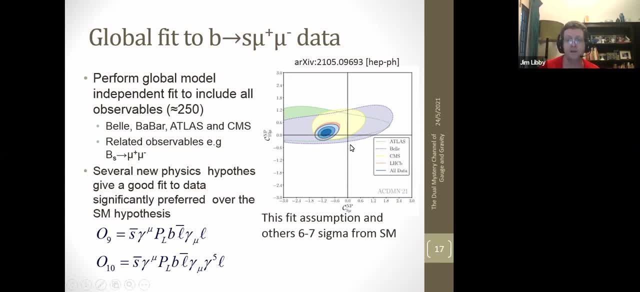 the best part is that it's pretty significant. we've got the highest p5 distribution. so that's though. there are those points. because they're larger uncertainties, they mean they don't have very much weight when you do the full fit in the end. Jim again, can I ask something? 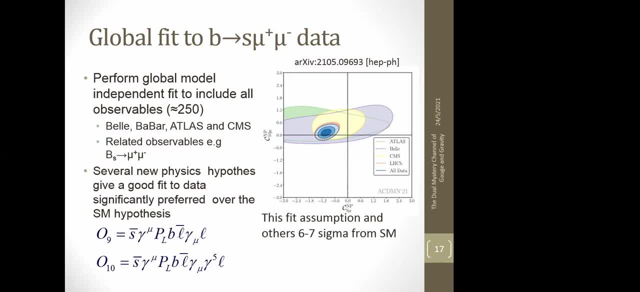 So in this case this O9, O10, will they also be important for some other processes- not say BBKs like some Higgs, triple tree body decay like to photons or I don't know? something simple like some other kind of ways you can corroborate to this operator. So these kind of things are. 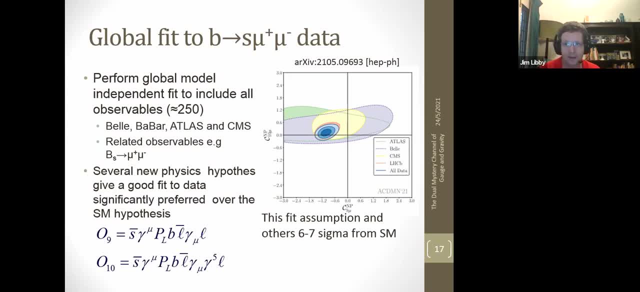 done in a way that they will escape other bounds. right, They're coming, but there aren't, you know, the coupling of the B to the S quark. that's only coming, really, in these flavor observables. okay, So this is a four quark operator, between the strange and the beauty quark that we're. 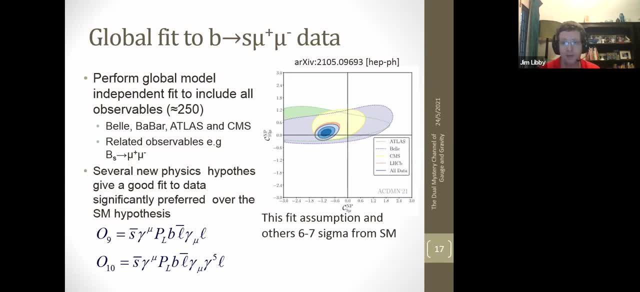 talking about here. Now, when you start talking about which I'll, I think I'll, you start talking about which I'll, I think I'll do. in the next slide you talk about what your new theory might be if you're a model builder. 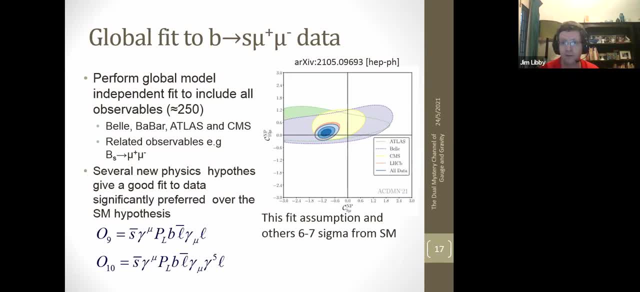 then you have to worry about what that does in the top sector or the Higgs sector or whatever else. okay, But these are. this is just an effective field theory approach. These are the coefficients. These operators are the ones. if you deviate these a little bit, you can explain the data And this. 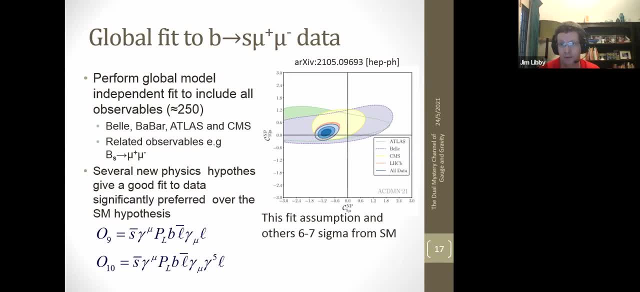 is essentially just adding some more left-handed current, Very naively. this is what this, this is doing, this C9 and C10 combination. So yeah, you're completely correct, You have to worry about other constraints, but that comes when you do the model building, I see. 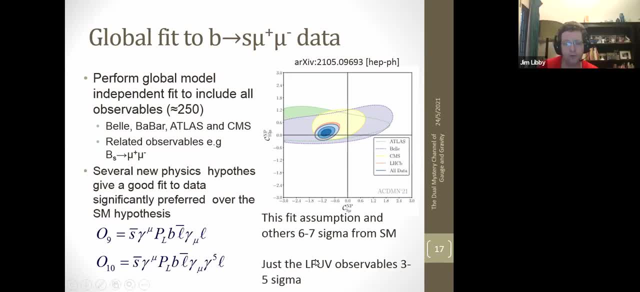 So so just to also: if, if you take out the angular distribution, if you take out P5 prime, the significance weakens a little bit. It's it's like three or five standard, three to five standard deviations away from the standard. 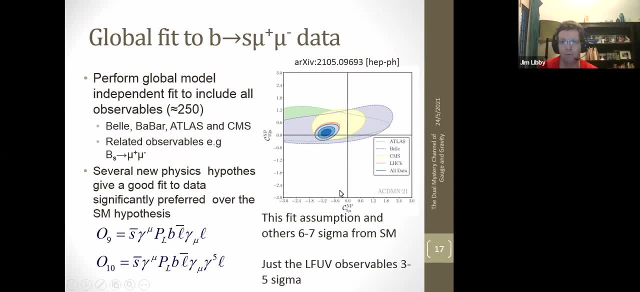 So, so that P5 prime variable is really important for driving the incompatibility of the standard model with the data, But this, of course, is still Sorry, just to just to ask again. So these two operators are special because they have coupling S and B And yeah, yeah, These are the only ones that can contribute to that. 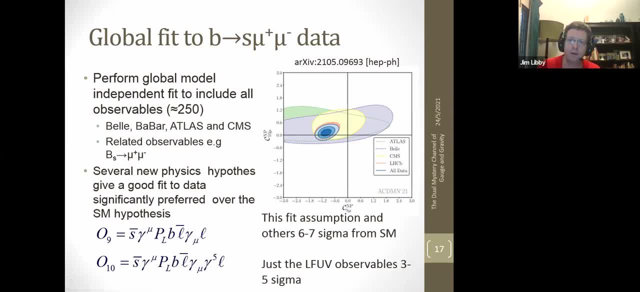 that BSLL process, right. So this, this, this is all. Yeah, we're looking at, that's all we can do in this effective theory, right, but you've got. whatever the rent structure is, you choose your operators and you know you're effective Hamiltonian and you. 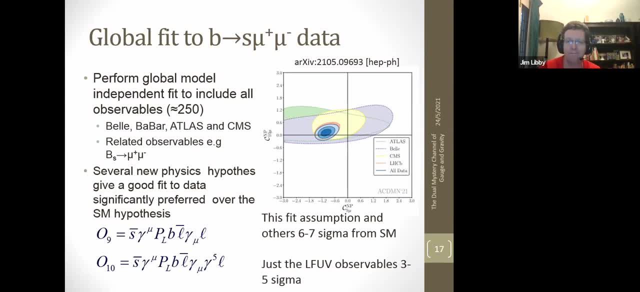 get this. this is not saying anything about what the real driver of this would be. it's just showing you this is. this is what it's going to modify, though there are many permutations for this. there are like 13 different permutations. if you read the paper, obviously I can't go through all. 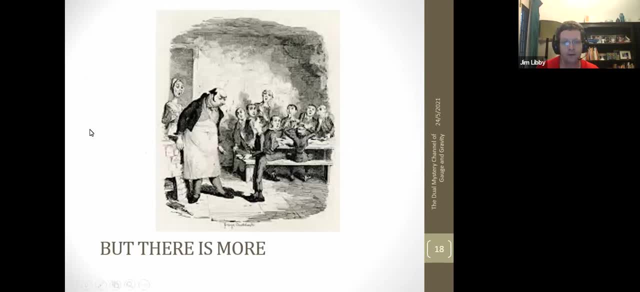 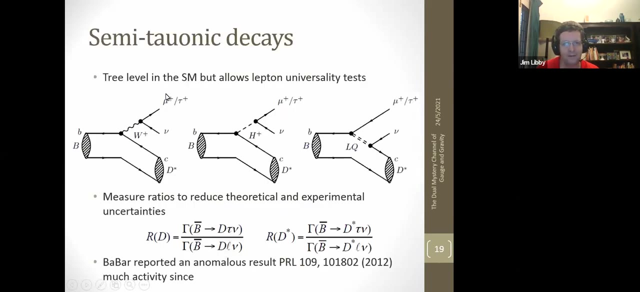 of those. so I'm going to get to the. so get back to my Dickens. this is, I'll put all of a twist- asking Mr Bumble for more and, unlike him, you are going to get some. so there are more anomalies. this is going to these semi-taunic decays now. now, this is tree level, as I mentioned before. so 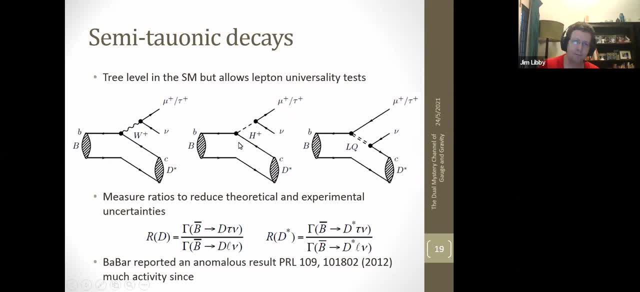 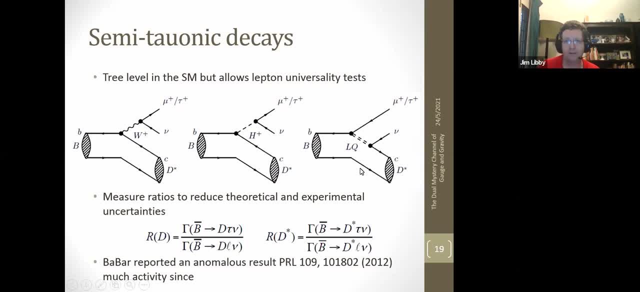 model theories, or something I'll come back to, is you can add a lepto quark that couples to both quarks and leptons and this will potentially mediate the decay as well. and what's done here is again a very robust measurement theoretically, because you take a ratio between the taunic. 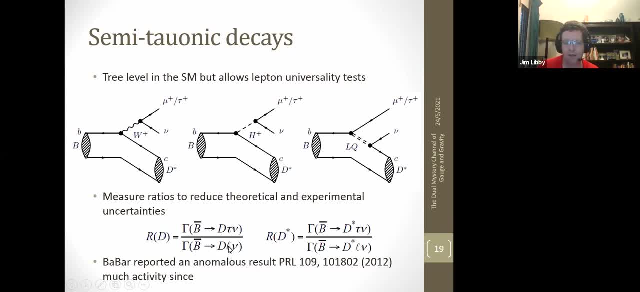 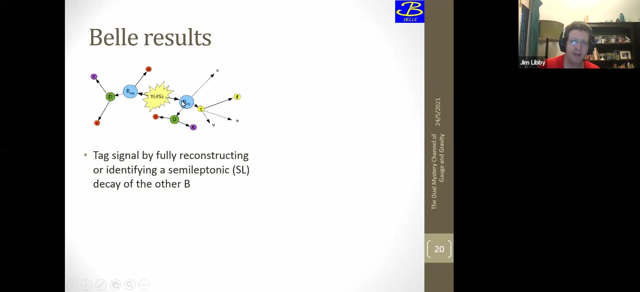 decay and the electron immune ones, and you can get very precise predictions for the standard model from this. now, this is the oldest anomaly of all this. there was a paper in 2012 from Babar that first reported the, the semi-taunic branching fraction, and it's just been off ever since, but many other measurements have been made. 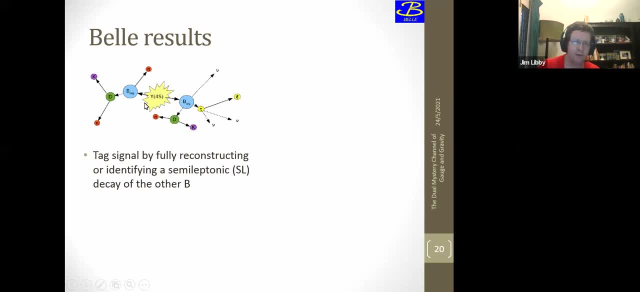 so Bell have got several results on this. I'm just going to highlight how they do this, because this is interesting for the second part of the talk. I'm going very slowly, I'm afraid, but I will try and speed up a little bit. they fully reconstruct events here, so you have two b's. 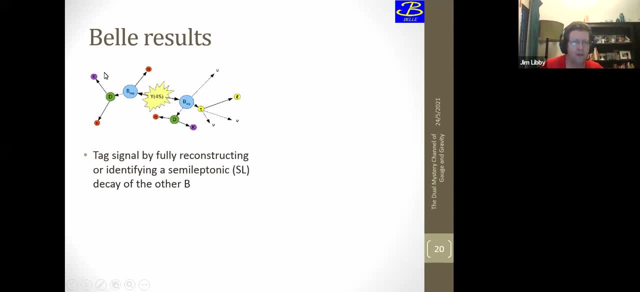 produced at the epsilon 4s. one of them gets fully reconstructed to a d pi event here. so you know fully the kinematic center of the side where you have your d to tau nu decay and you have your tau decaying to a single lepton and you have these three neutrinos. so, using the heavily constrained 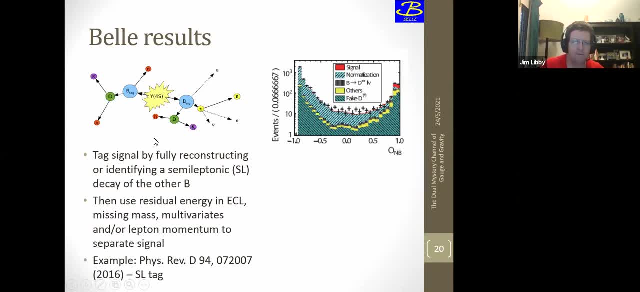 kinematics and you can the shape of the events and and the leptons and the leptons and the lepton momenta involved. you can distinguish these between the regular muon decay or electron decay of the b and the tau decays. and this is does some you know. I think this is a neural network. 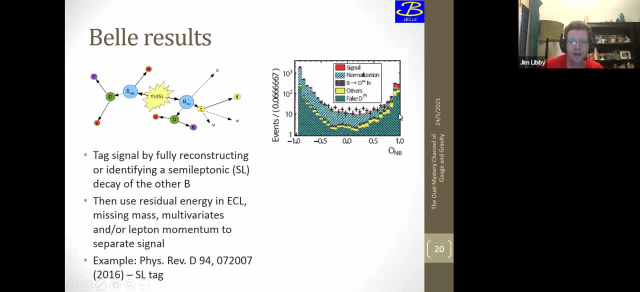 yeah, it is a neural network, not a boosted decision tree, and- and the signal here is this tiny red piece. but using this multivariate discriminant, the signal piles up here close to one. all the backgrounds are here at lower values. this is a neural network and it's a neural network. 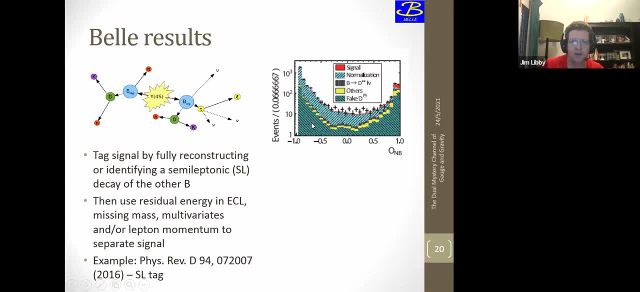 this is the normalization in the sort of turquoise hatch, and then there are combinatoric backgrounds and then some higher d star resonance stuff as well, where you're missing particles. but then you can select out that little region and because if you've really reconstructed everything in the event, 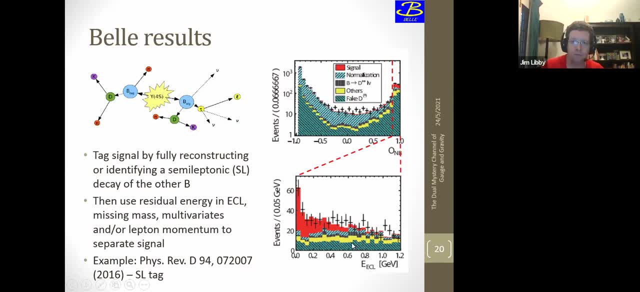 you'll have nothing in your calorimeter at all and this true signal piles up at zero extra energy in the kilometer. of course there's some photons flying around and you end up with a few hundred mev extra energy, some of the time from initial or final state radiation, but it's a. it's a clear signature and this is the signal. 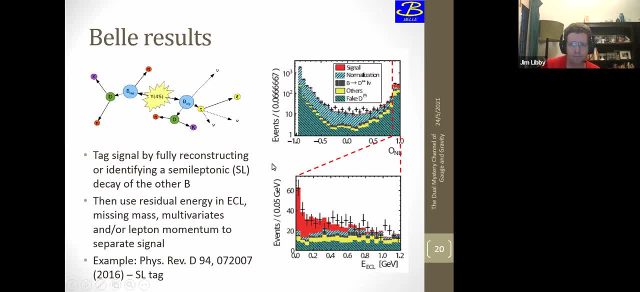 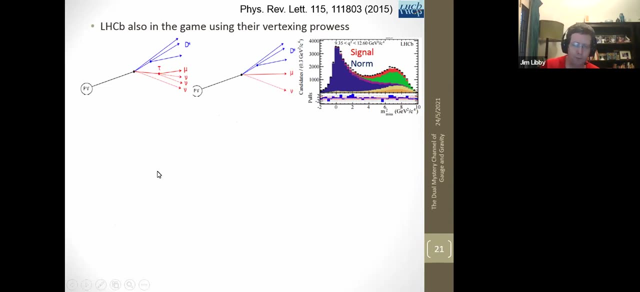 over background that they have for d star tau nu. and then there's also a semi-leptonic tag version where you it's not quite as clean but you have much higher statistics, so you gain something. now lhcb also do make measurements of of these b to c tau nu and they exploit the 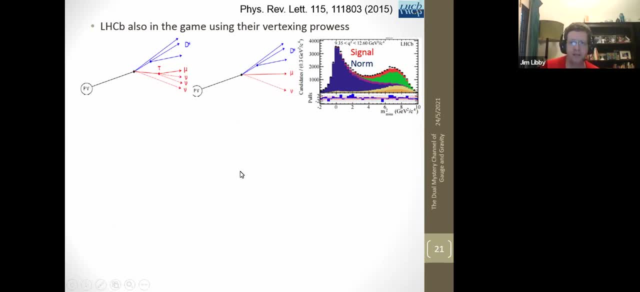 very good vertexing. that they do and they're very good at doing that and they're very good at that they have. this highly boosted b's into the acceptance of the detector means that they can reconstruct not only the secondary vertex where the b decays, but also the tertiary vertex, where 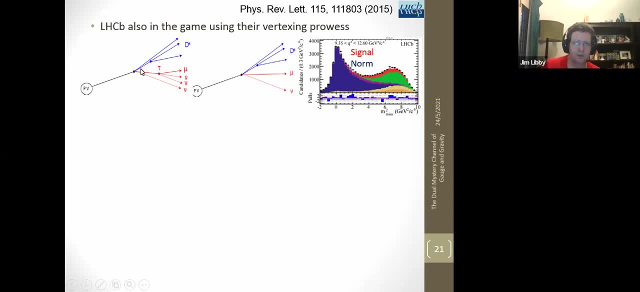 a d star. um, sorry, there you have the. this is the odd looking, the, sorry that where the d decays here and the d star. this is the slope ion from the d coming directly from this vertex. so they can reconstruct these three different vertices and they can distinguish. 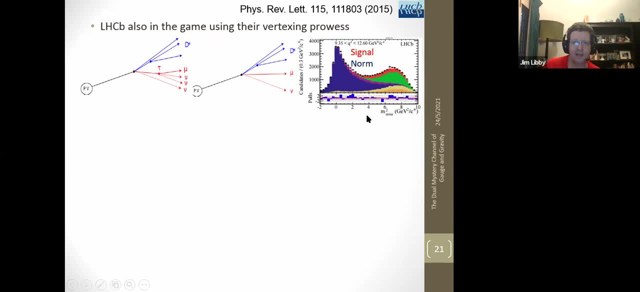 between the tau and the mu by looking at the amount of missing energy. however, their little red signal here is a top, a very large background and um this green in particular is where you have d double star decays, where you're losing some particles in the detector. 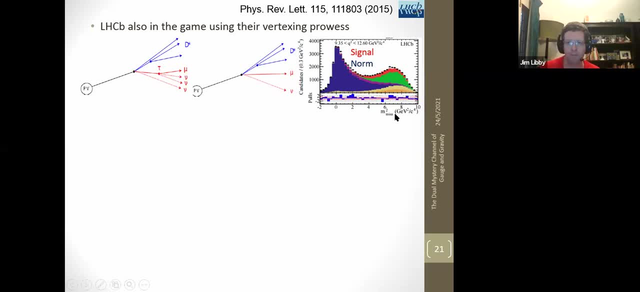 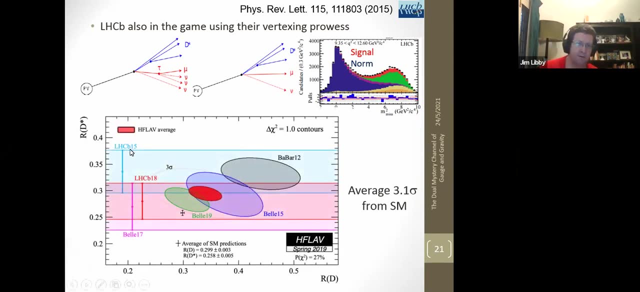 and this is very hard to understand. so this is, uh, quite a model dependent measurement and very difficult measurement, but if you put all this together, you have a set of measurements that are hijacked okay, so you have some reduced S torch of a star, but which then relaxes with the 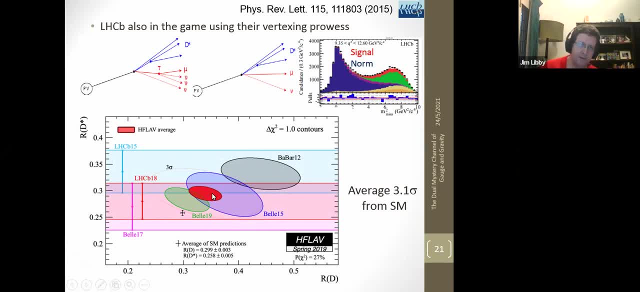 decays of saudianjat, but it's very, very powerful. okay, there is the big exploded системаhouse here. through this, gain a yet for diversity point. Shree Hari- and I'll come back to this- may want to just believe these two measurements. 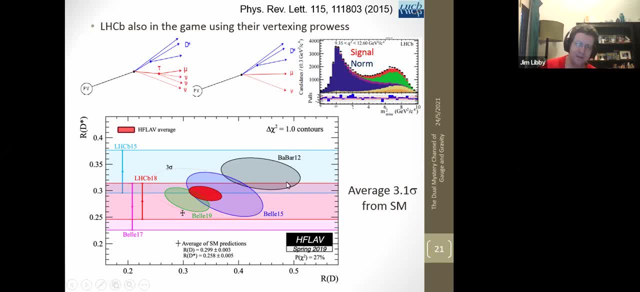 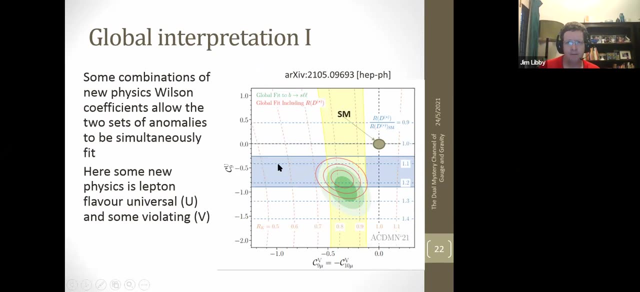 but this has held up over essentially three different experiments measuring this and it's still significantly disagreeing with the standard model. So, going back to these global fits, it's the same paper that I showed earlier. You can add in these RDD and RD star variables and you can fit again to these Wilson. 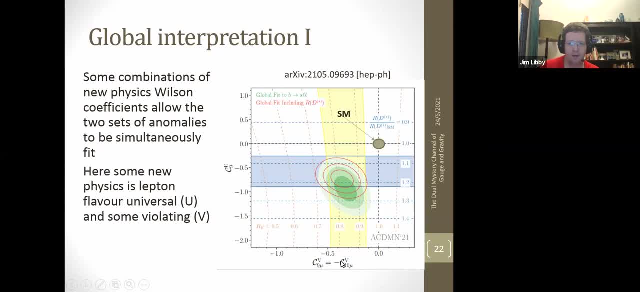 coefficients. So here you have V minus A, violating lepton number, not lepton universality, violating Wilson coefficients versus a new universal one as well, And with that you can actually fit all the data together. So the green is the B2SLL and then, if you include the RD, 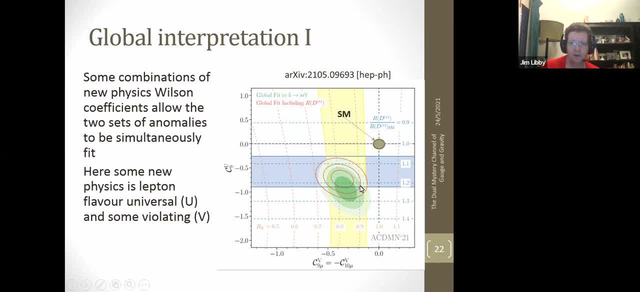 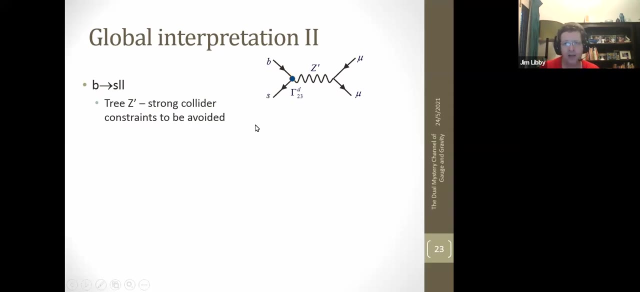 you get to the red region and that's a significant disagreement. Again, many standard deviations away from the standard. But of course, what is the underlying physics interpretation of such a scenario? Now, I'm not going to talk about this in great detail, partly because I'm not expert and partly 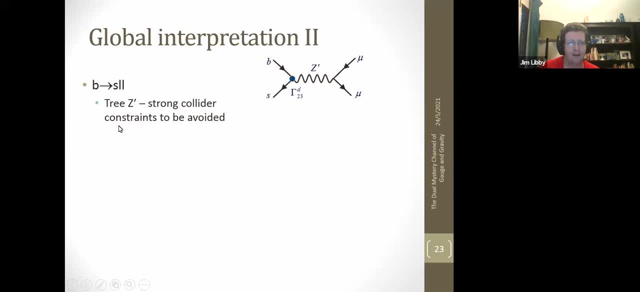 because I'm a bit short of time now. So you could think of tree-level solutions where you add flavor-changing neutral currents by having additional gauge bosons with off-diagonal couplings, so what we'll call Z primes. but there tend to be strong collider constraints. 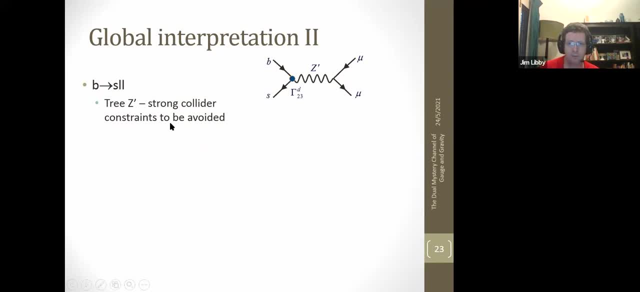 for such tree-level solutions to all of this. If you just look at B2SLL loop, you have many, many possibilities: scalar vector fermions, two-higgs doublet models, Z primes coupling to top and a doublet of these lepto quarks. But if you try and do everything together, 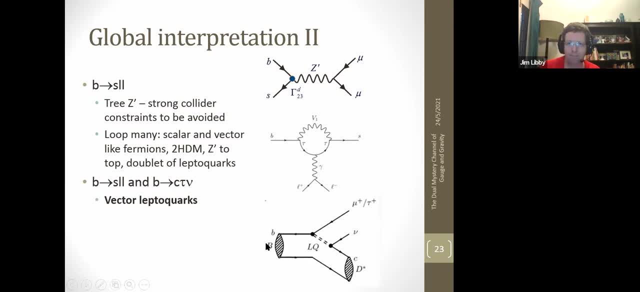 one beyond the standard model scenario sort of stands up and that's lepto quarks or vector lepto quarks, where you can have this lepto quark in the loop where you'd have a tau, and this vector lepto quark mediating your B2SLL transition, and you can also have that, as I've. 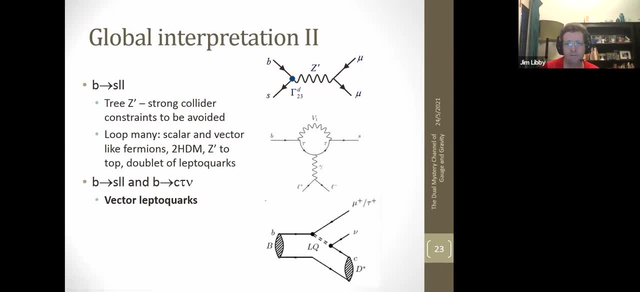 shown before, leading to this tree-level effect, And given it's got preferential couplings to the third generation, you can kind of escape other collider bounds on the lepto quark because of this. But there's no additional Higgs Sector being added for this, so the UV completion is a little difficult. 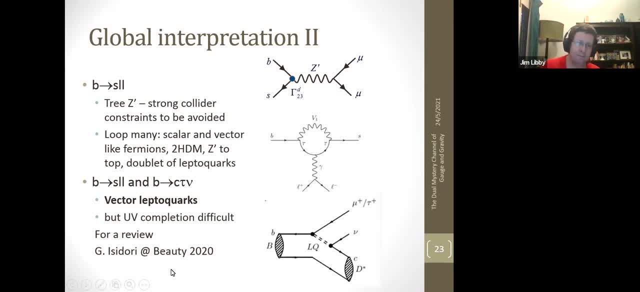 I don't want to talk too much about this, but there's a very nice review that Gino Isidori gives- One I saw was at Beauty- I think he's given it elsewhere- which really digs into these different possibilities And essentially he advertises what I'm going to say in the last. 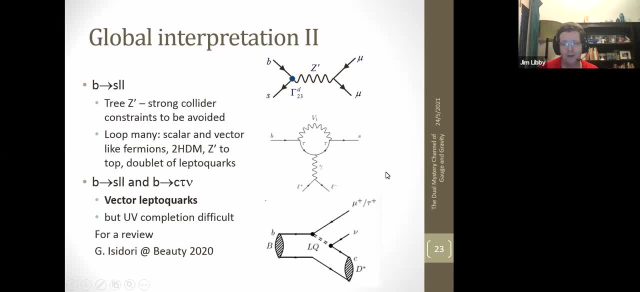 little bit of my talk. So, Ayan, how much more time do I have? 10 minutes, Okay. Yeah, that's kind of okay. I'm going to have to skip a couple of things about Bell 2, but that's okay. 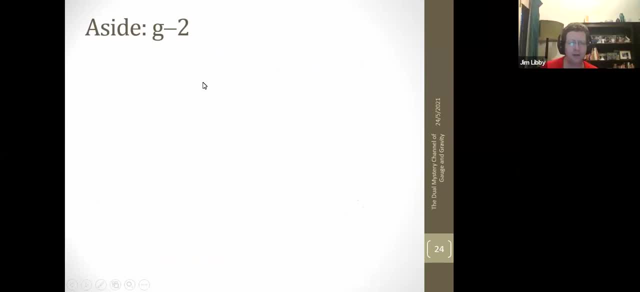 But you can take a little bit more time also, no problem, Okay, okay. So before moving away from the anomalies, I should say something about the other anomalies that are around, because they are often said to be able to be fit by this pattern. 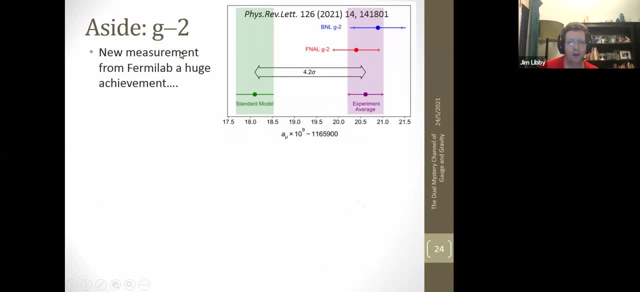 as well, Sorry. So the other mainstream media physics result, or particle physics result this year has been G-2, which has this very impressive 4.2 sigma standard deviation between the generally accepted standard model prediction, I should say- and the new measurements, And this effort to make this new G-2 measurement is hugely. 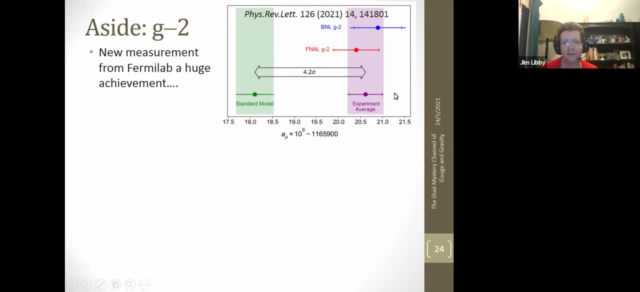 impressive And anyone interested in experiments and what they've done to do this in terms of the homogeneity of the magnetic field and the inhomogeneity of the magnetic field and the inhomogeneity of the magnetic field and the intense source of muons, and the careful analysis- blind analysis- that they do to measure this is a. 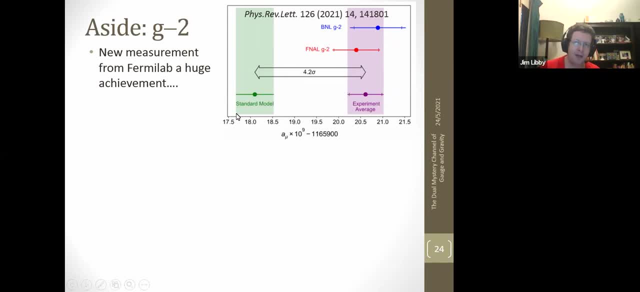 very interesting and extremely impressive endeavor, And that's also true of the theory which is producing this number. Now, this plot down here gives the various predictions for this anomalous moment of the muon from different theoretical approaches. All these in blue are: 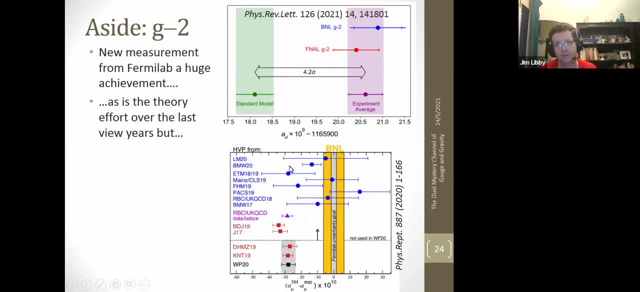 from lattice QCD ab initio calculations from lattice QCD And these come from interpreting other data in terms of dispersion relations to work out this hadron vacuum polarization. So that's a talk in itself. But these two down here are taken as a state of the art, which rely on E plus, E minus measurements to light hadrons and 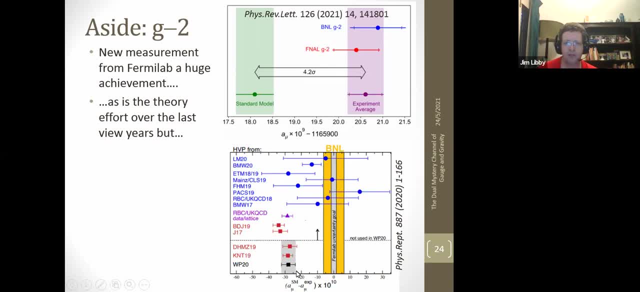 tau decay. And this gives the world average number that I show up here, But the eagle-eyed among the. And this gives the world average number that I show up here, But the eagle-eyed among the. and you've probably read about this. there is one of the lattice calculations which has the smallest. 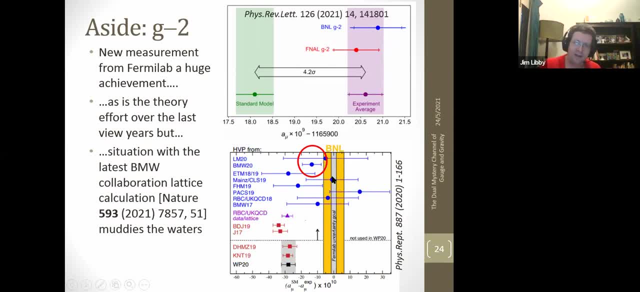 uncertainties, which is not that incompatible. This orange band roughly corresponds to where the experimental value is, So it's just less than two standard deviation effect And, as you see, all these lattice numbers are scattered around all the way between this dispersive relation number. 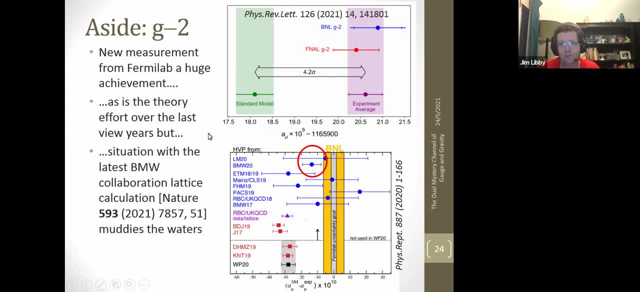 and the experimental result. So I must say I'm no expert on lattice QCD and I don't want to discuss the, the, the, the virtues or lack of of these particular measurements. i i can't comment on that, but i do feel that this is going to really muddy the waters on this g minus 2, anomaly for some. 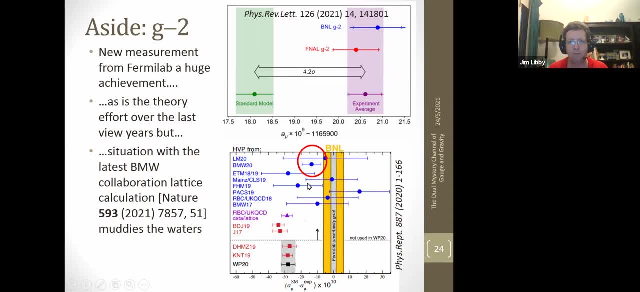 time until the lattice community can fully agree on whether these uncertainties are a good or how other collaborations can uh test this. so this is a somewhat unfortunate state of affairs, given the great fanfare this was announced with. i i i want to dig into this. i'm 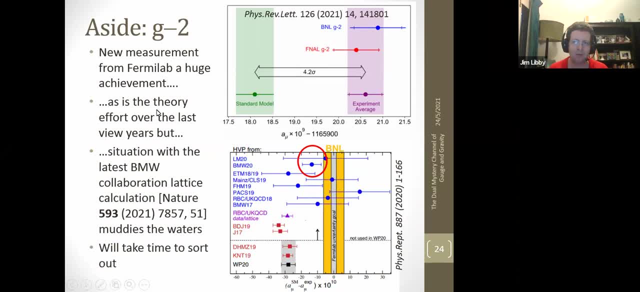 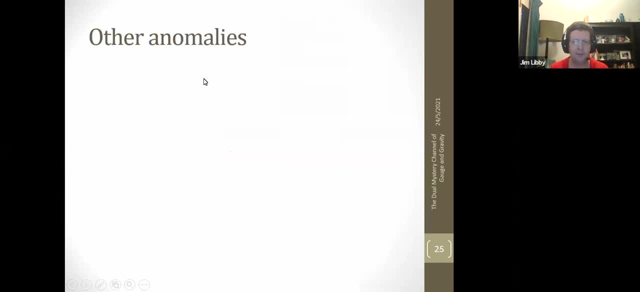 i'm a little, uh, a little less optimistic than i once was, but it takes nothing away from the experimental effort that's gone in to make this measurement. but there are other anomalies which are quite interesting as well. one is this kubibo angle anomaly, where you're measuring 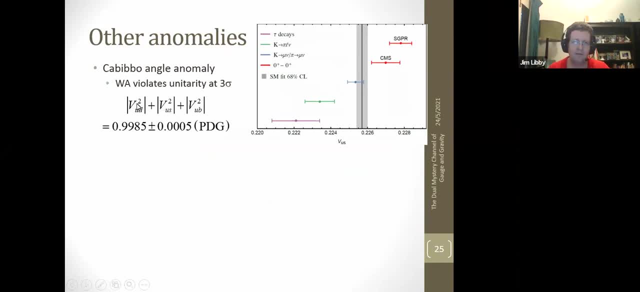 um, the coupling of the upquart to the strange quark. and if you take this sum of these three ckm matrix elements it should come to one. it's a unitary matrix but it's three standard deviations away and there are various ways of measuring this. you can measure vud and uh, then work out. 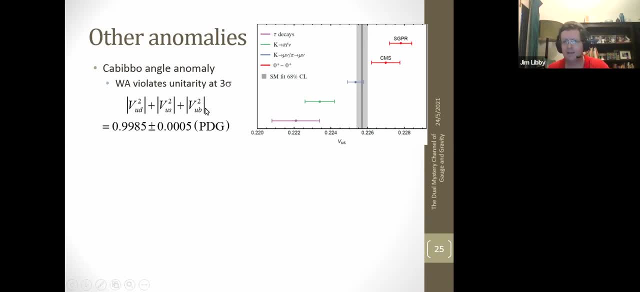 what vus should be, because vub is so tiny, it has little impact on any of these measurements. it's really about vud and vus. you can measure it in k on decay, or you can measure- you can measure us directly in k on decay or you can measure it directly in tau decay and you see that there's 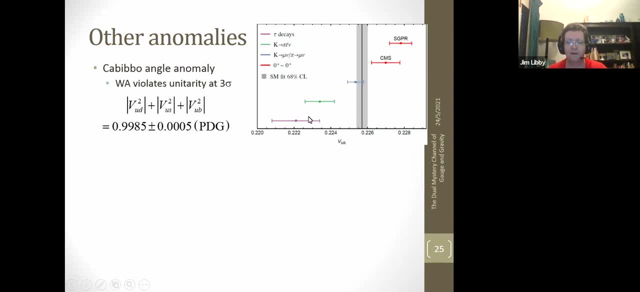 a trend amongst these, rather suggestively plotted in this in this way, and of course this buys into the idea that there might be something to do with lepton universality. this is measured in taus here, this is measured in mu's and this is measured with electrons. uh, and these are kind of largely theory. 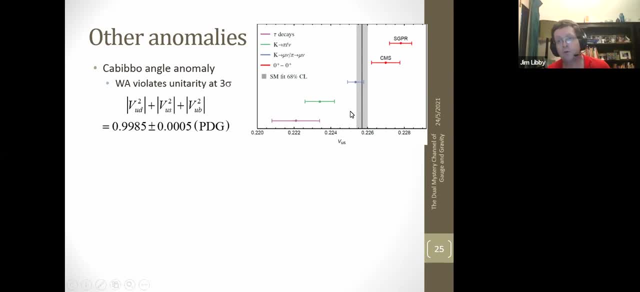 dominated in their uncertainties. but the tau measurement can certainly be improved experimentally, and that is on the list of things that we're going to talk about in a moment. uh, so i'm going to give you a list of things that bell 2 will do in the next decade, also with the taus. 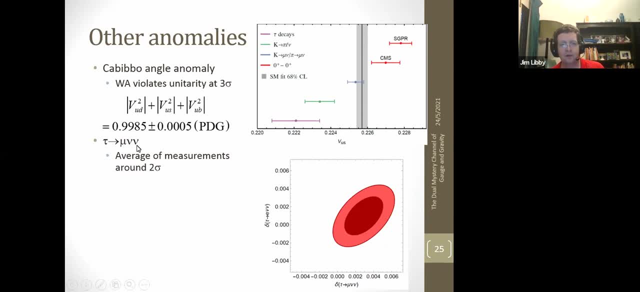 there's some tension between a tau decaying to a muon and two neutrinos from what you'd expect from the standard model um, and this is shown in this two-dimensional plot. that zero. zero is the standard model here, but the central value sits off a little bit to higher values for tau nu. 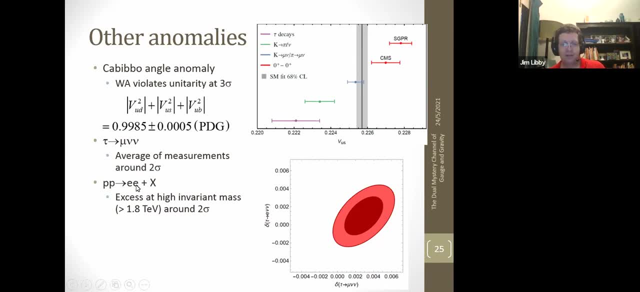 and there's also in hadron physics there's a hint of an excess of dielectrons at large invariant mass. but with my experiment- and these of course can all be linked to lepton universality, but with my experimentalist hat on anything- that's just two standard deviations. 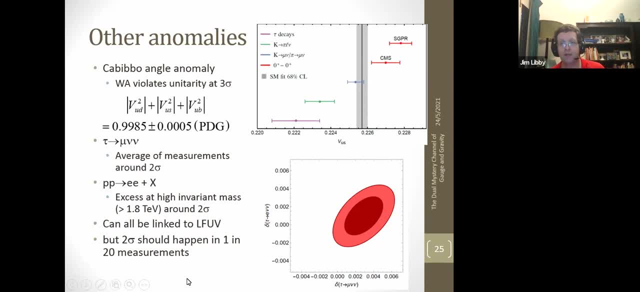 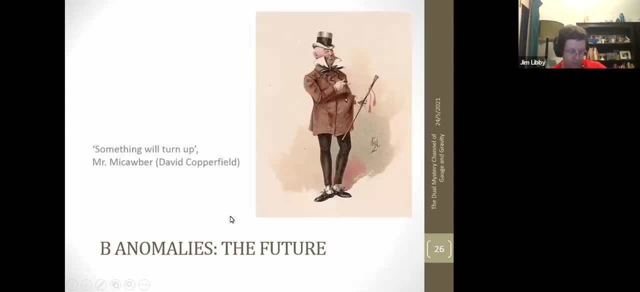 i, you know it's one in 20 measurements should disagree by two sigma. so we should always be careful. so the future i will. i i'm like mr mccall, where something will definitely turn up here, but it's the matter of when. so the lhcb experiment is currently being 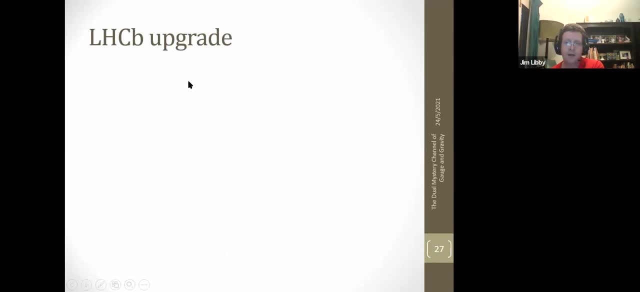 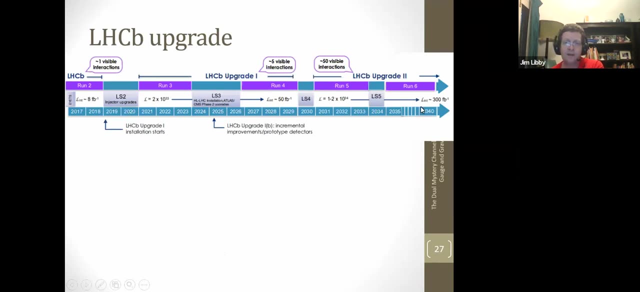 upgraded for the start of run three, which should begin early next year, and they have a timeline to continually upgrade their detector well into the 2030s and and finally accumulate um around 300 inverse femto bonds of data when they currently have 10, so 30 times more data. this is done by 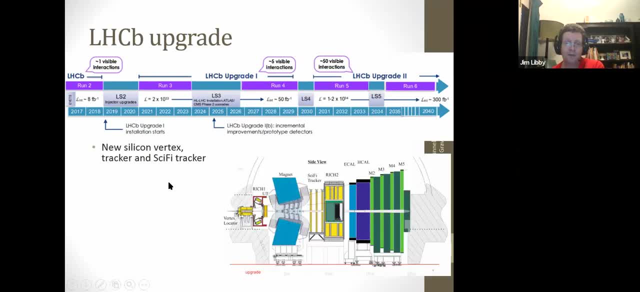 essentially surviving up to 10 times more data and which will end up in the second half of 2030.. higher luminosity and they've had to upgrade their detector significantly. so there's new silicon detectors downstream of the magnet and then upstream of that- sorry, downstream there's the 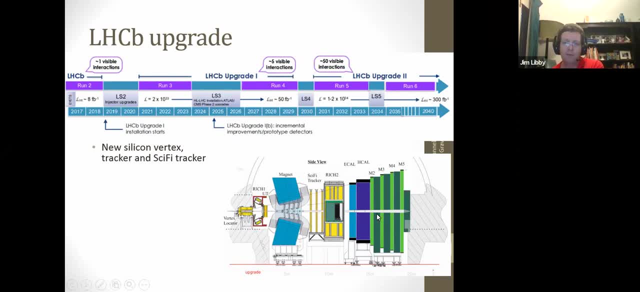 silicon, and upstream there's a new tracker, but no upgrades to their calorimetry, so they'll still have the same limitations as before. they are now reading out all their data at 40 megahertz, so the triggers purely in software, which is very good for hadrons but not so good for leptons. they were. 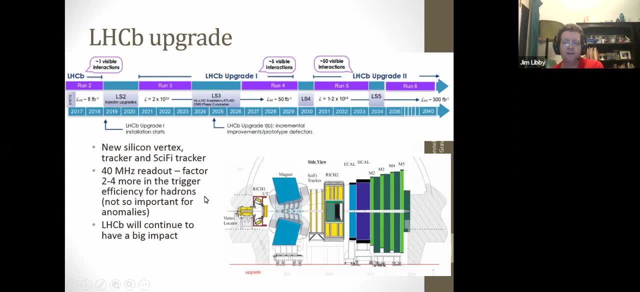 already very good for leptons, so this will continue to have a huge impact and will be the leader for some time in the years ahead. but i want to spend what time i have talking about um, so i should also say cms and atlas are forever putting more emphasis on b physics too. 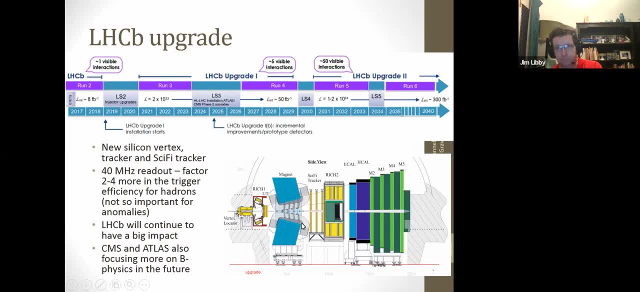 and they will come with results. but they have not quite as severe problems with electrons as they have with leptons, so they're not as severe as they are with electrons. lhcb does so that the lepton universality will be quite interesting when they, when they do this. 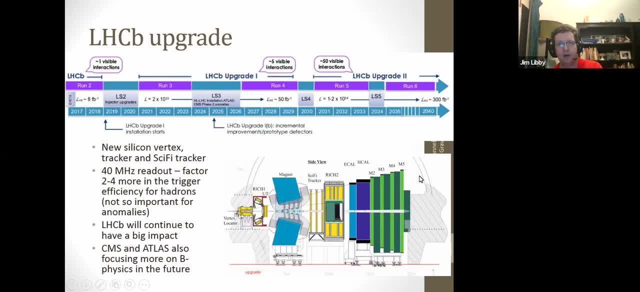 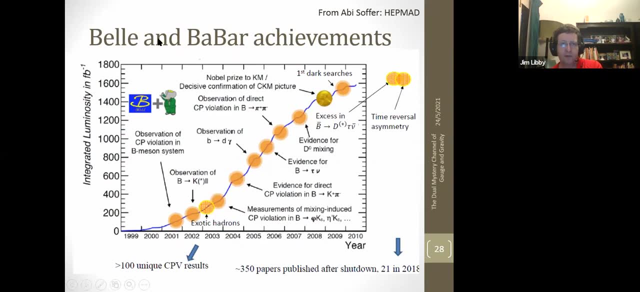 but it's a very busy environment and again it's it's much harder than what's possible at bell 2. so bell 2 builds on the success of the bell and babar experiments, which ran through the first decade of this millennia, where they collected around 1.6 inverse attabans of data. 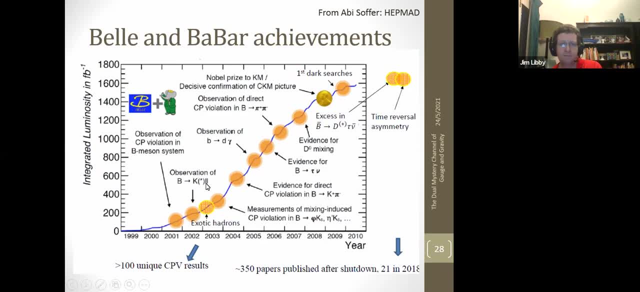 there are many significant achievements, some related to these beta sll and some related to these beta sll, and some related to these beta sll and some related to events. i talked about types of decay. there was a nobel prize for confirming the kabiba, my 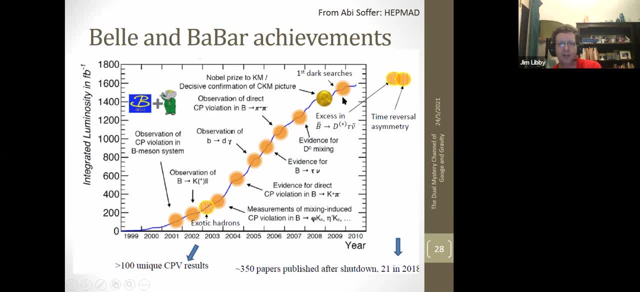 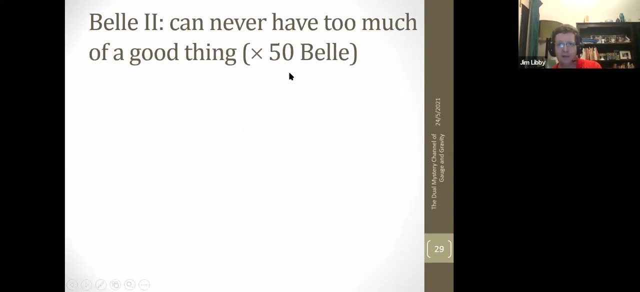 kobayashi- sorry, the kobayashi-maskawa mechanism for cp violation and of course, this excess in b2t star town u was also, after running, discovered by the very careful analysis. so bell 2 is essentially- you can never have too much of a good thing- and and it's an attempt to to collect 50 times more data than bell. 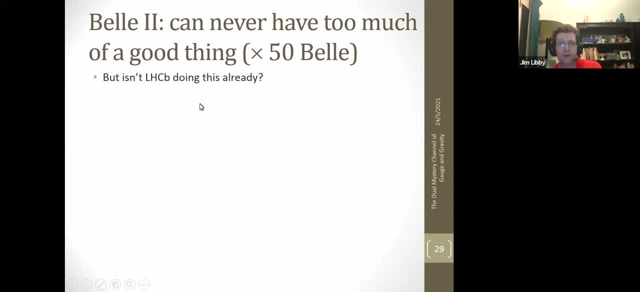 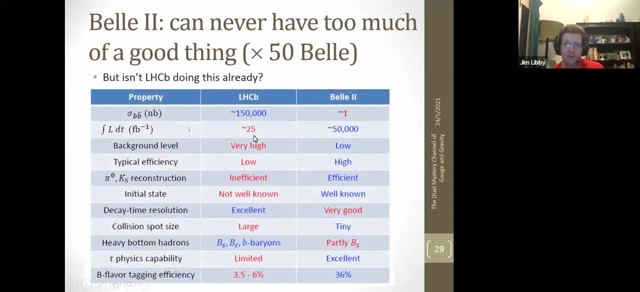 b2 star town u was also after running, discovered by the very careful analysis. so bell 2 is essentially so around 50 inverse attabans of data. so what? what would it be able to do that lhcb isn't able to do? so? lhcb has this huge statistical advantage. so this 1.6 inverse attabans corresponds to around 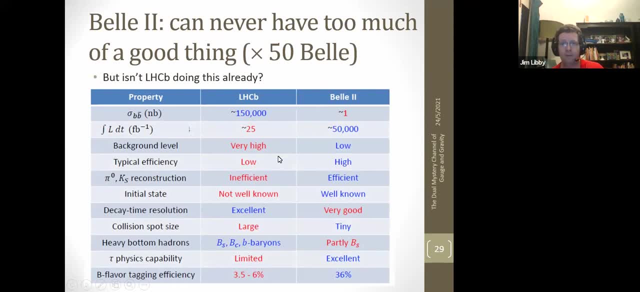 one and a half billion bb bars. so it's a much smaller data set in comparison to what's possible at the lhc, but um, it's. it can be a little bit more complicated, but it's a lot of work. um, we'll see a very high luminosity machine to partly compensate for that, and it has much lower backgrounds because 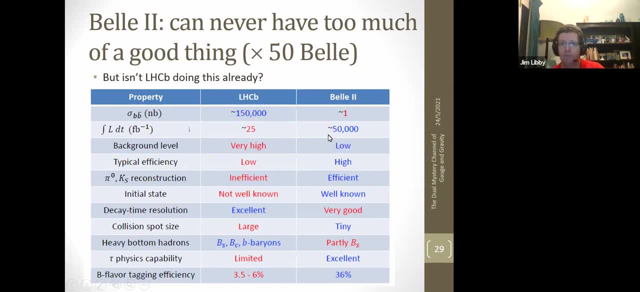 you're still producing, just like argus, a b0, b0, bar, a b plus and a b minus, and nothing else. so it's a very clean environment to work and hence you have very high efficiencies, and you're efficient for neutral particles as well. so we can measure all of these anomalies with k shorts as well as. 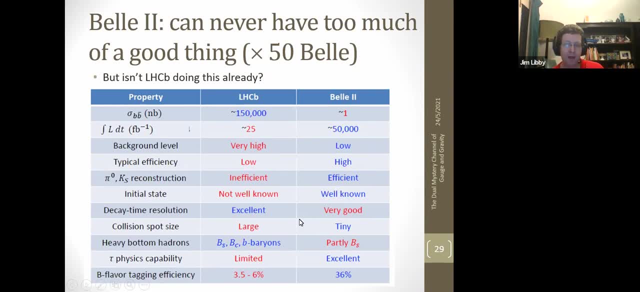 charged particles. we have this well constrained kinematics, unlike what you have in proton proton collisions. you have not quite as good vertexing because you don't have that huge boost. we have some boost because it's an asymmetric machine. it has a very small primary vertex though, which helps. 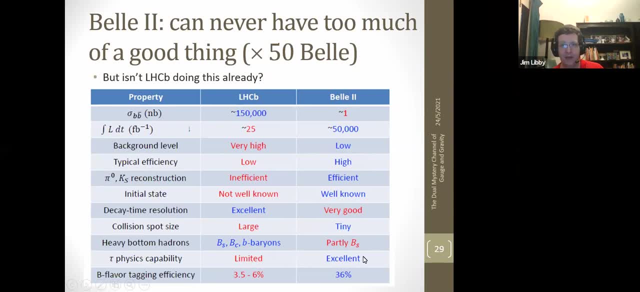 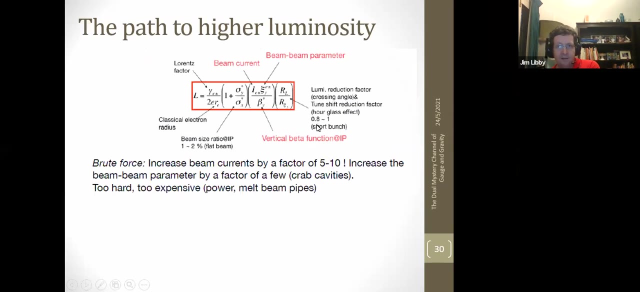 it doesn't produce all types of b hadrons, it only produces b0 and b plus has very good tau physics which i won't talk about, and this flavor tagging efficiency i also won't talk about today. so how this is being done is really an upgrade to the accelerator, it's not. 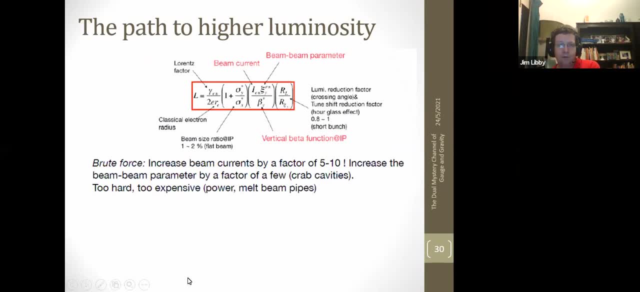 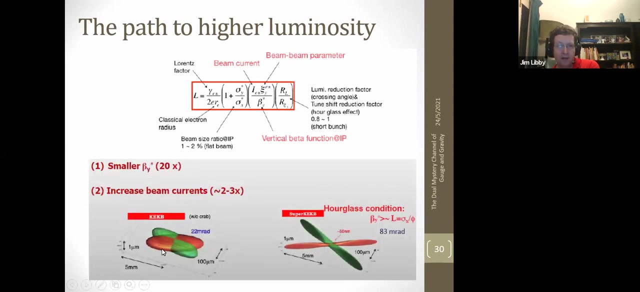 really to the detector. so this is the master formula for luminosity and there are two parameters i'd point you out. one is the beam current, so you can increase luminosity by boosting the current, or this beta star function here, which is basically the beam current. so this is basically how small you can make your beams. now the brute force approach of increasing the currents would actually melt the beam pipe through synchrotron radiation. so the second approach is taken where we've squeezed down how we collide our billions. so the green and the red are the electrons and positrons bunches colliding as they were in bell on the left and as they are being collided now in bell two. 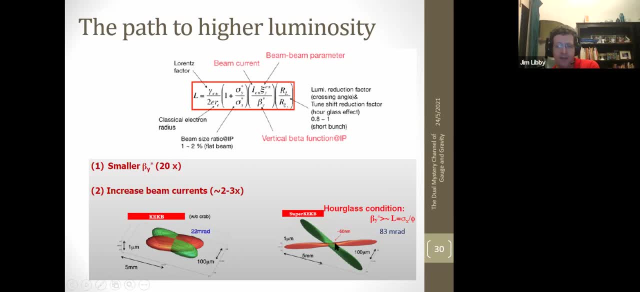 in super keck b and they have this power glass shape which essentially squeezes down this region to a few nanometers, tens of nanometers where they collide, and this allows for very, very small beta star function and and will get us to these very high luminosity is a factor of 30 more than was there a bell, so we can integrate this large sample. 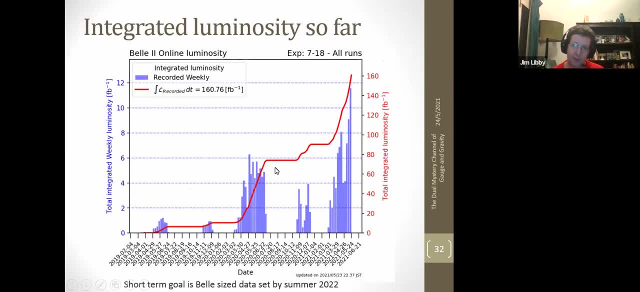 so i'll skip over the accelerator details, but you can ask me about that. but we're still a long way from that. this is a plot i took from the reconstruction last month, so you can get a very small sample from this map for this przykład. 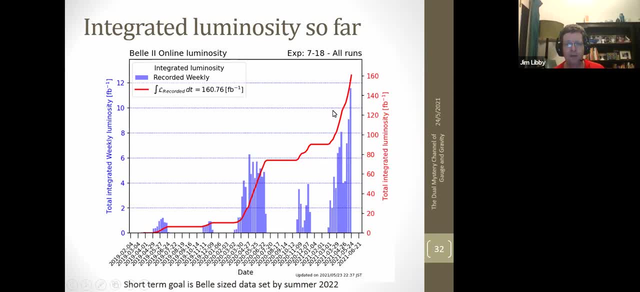 so in some way i think this is well. louisiana's explanation by it's not crying and talking to me is true, though. so these lethargy, sûr, that's actually needing some space, social ounce of world where these littleı arms will só for a long time, but I won't in this forum. but the long-term plan is that we're down here in. 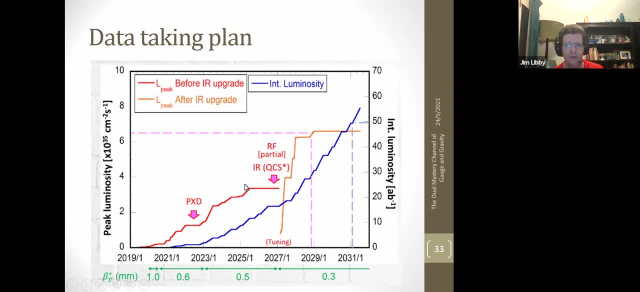 in 2021. the blue line is the integrated luminosity, the red is the instantaneous luminosity. we are still some way from our target of getting up to this six times 10 to the 35 instantaneous luminosity. we're still down here. actually, this is slightly out of date. 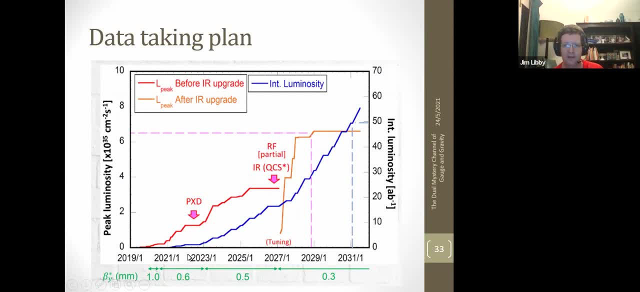 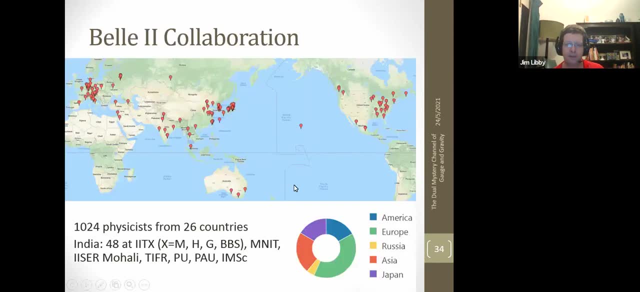 and there are some upgrades that are required for both the accelerator and the detector to get there, so our data will only come within the next 10 years. it's a slow process of accumulating this, so the bell 2 collaboration is global, with about five percent coming from India. 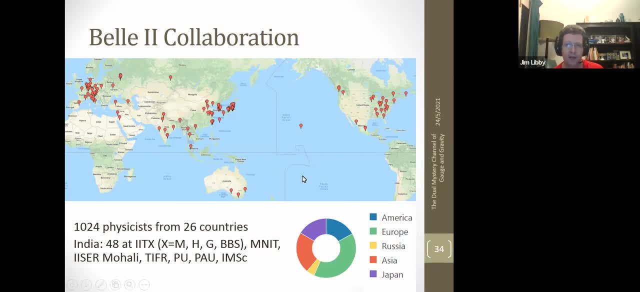 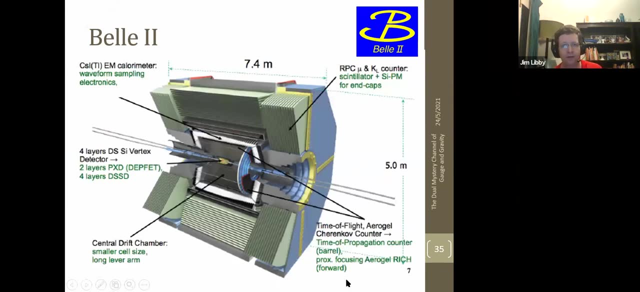 it's a thousand physicists, so it's a bit smaller than the LHC experiments and the detector is much more standard than LHCb. it has all the things that one normally expects from a general purpose detector. it also has that hadron ideability ability. it's been improved for bell 2 with a timer propagation counter and also the silicon is 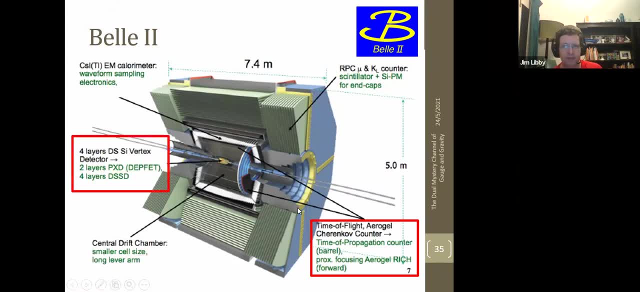 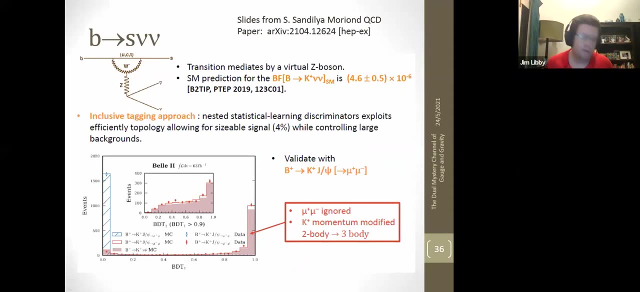 much improved as well, and various bits of the readout and other things were redone, but the larger upgrade was to the accelerator rather than to the detector, so even with the small amount of luminosity, we've actually got a measurement that's of quite great importance to what I've been discussing in this talk, and this is b2s. 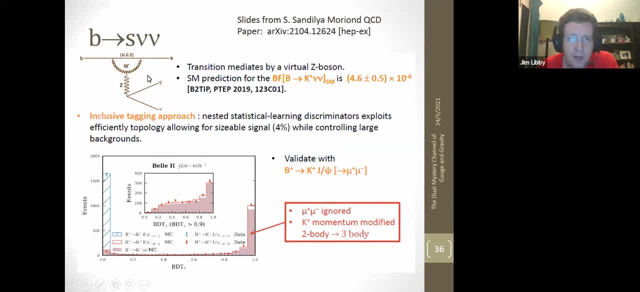 this is a new, new bar which goes through the same kind of penguin diagram as those b2s, LL anomalies, but here of course you'll be summing over all the possible neutrino types. so your new physics that might be contributing to the lepton flavor via. 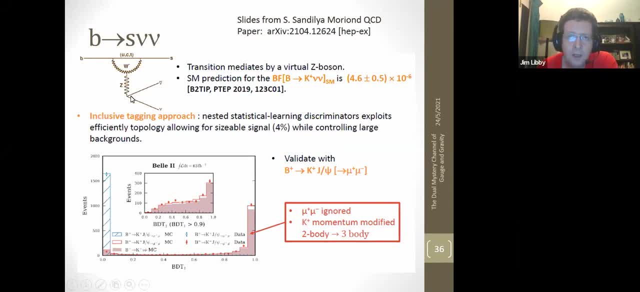 lepton universality violation that one sees in RK, for example, would impact this in measurement. so you can see that the standard model would expect the standard model prediction would change depending on the new physics. so this is a correlating observable and even with a very small amount of data and some extensive use of machine learning algorithms to identify a signal. 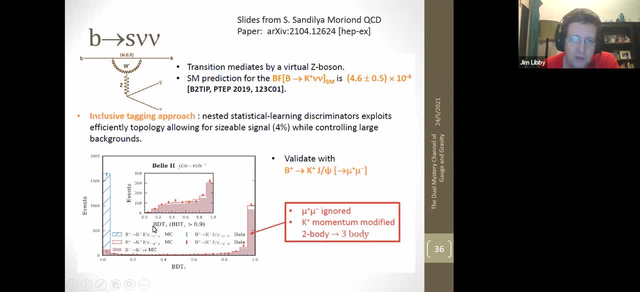 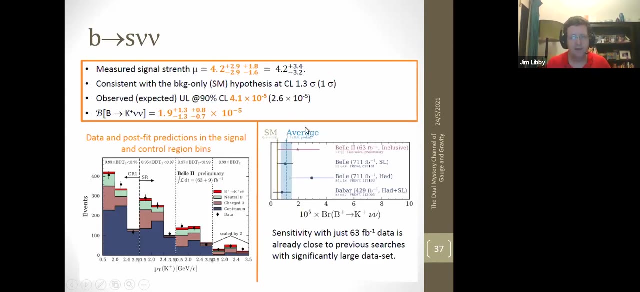 using, again, data driven techniques to do this. you can use a succession of boosted decision trees to actually isolate the signal. so the signal is here in in pink and an upper limit's been set with just 63 inverse femto bonds of data, which is competitive with 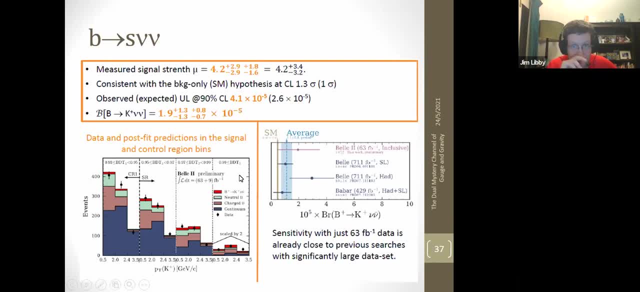 previous measurements using these combinations of boosted decision trees. so with the data we we will get by next summer, and also re-analysis, potentially of the bell data, we should be getting a very interesting measurement because it's getting very close to the standard model value. so whether we see an enhancement or a suppression of this would tell us a great deal about what 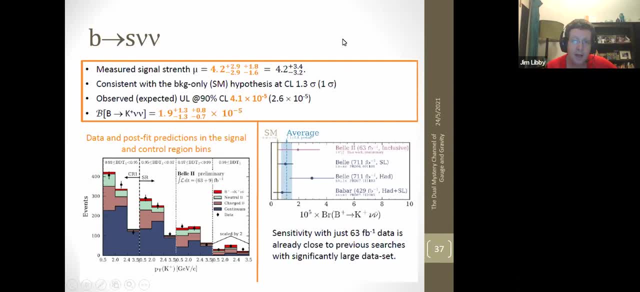 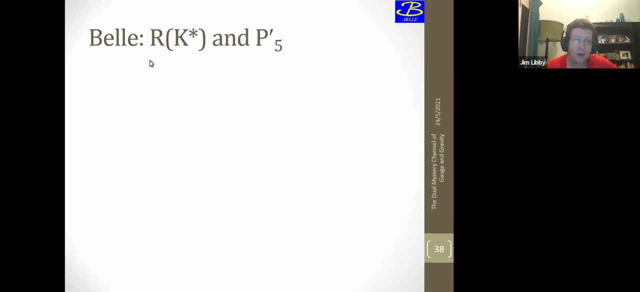 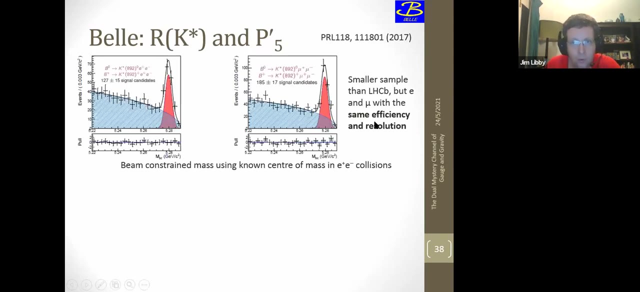 might be going on in the B2SLL anomalies. then finally- or not quite finally- finally on on the B2SLL RK star and p5 prime. the important distinction that's there between LHCb and bell2 is that we are highly efficient for electrons and we also have very good 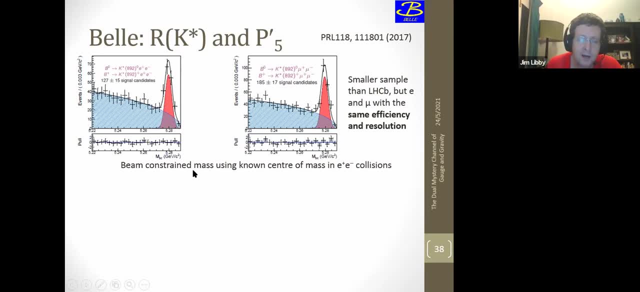 resolution by exploiting the constraints, kinematic constraints, that come from the knowing, the plus, e minus, collision energy and its momentum. so here on the left we have a bell measurement of k star LL for both electrons and muons, and it's roughly the same efficiency. it's 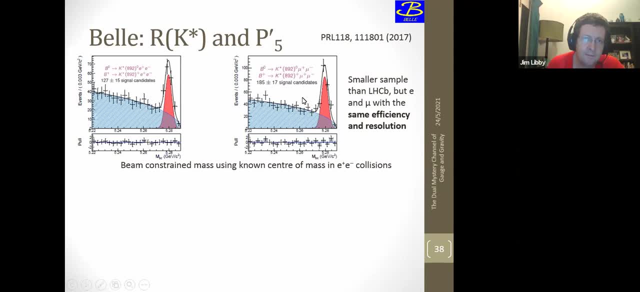 a little lower for electrons, but but not as dramatically as LHCb, and the resolution and the background levels are very similar. so this is a very interesting measurement because it allows p5 prime to be measured for both electrons and muons, and a very robust observable would be to take the difference between p5 prime, so-called 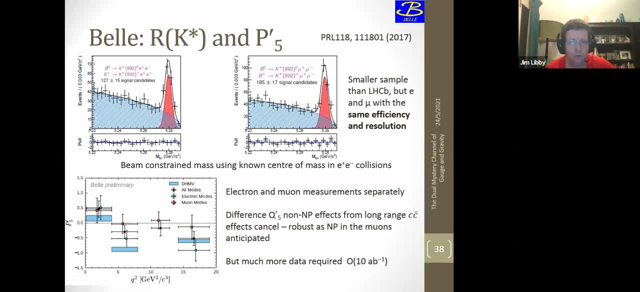 q5 prime between the electrons and muons, and there some hadronic ascertainties cancel out. and also you expect new physics in the muons but not the electrons in most of the new physics series. so this is a bell measurement, but we will do much better than this as we accumulate more data. but 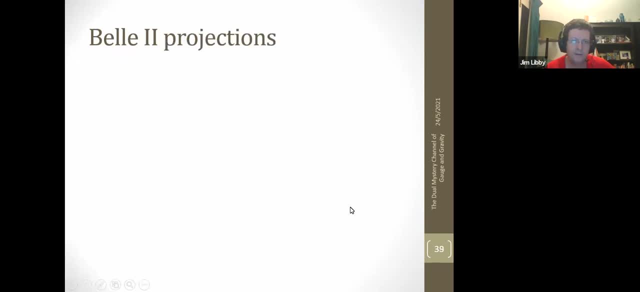 until we get to 50% of the data, we will still need to do this analysis and we will then work on it by adding at the very end of the nacional data. we already have 50 numbers of number of electrons and muons, and then we can also have 60 numbers of electrons and muons. and then what? 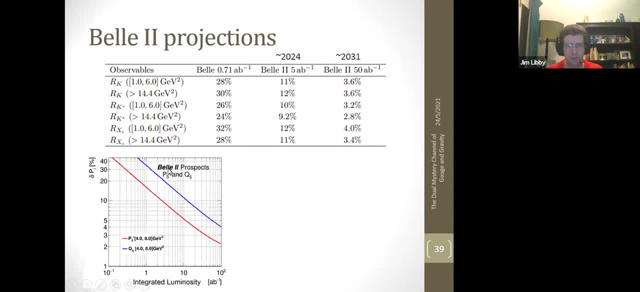 happens is that in the end we have a very largekre meidän 60 numbers and we can use 60 to say 70 km of of data. in that short time we could actually add at the very end of the data 42% of alter bonds of data before we'd have something very 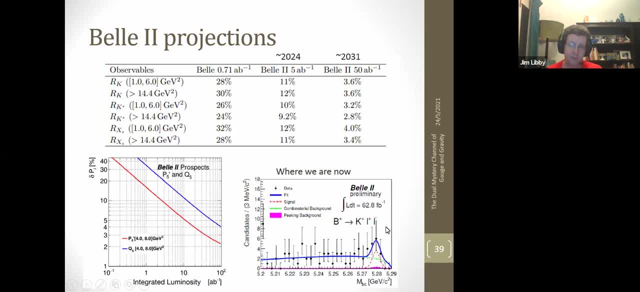 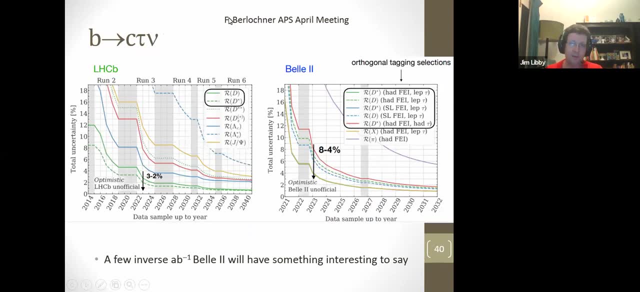 meaningful on this data set. Of course I should also talk about B2C town, new prospects at Bell 2.. I recommend Florian Bernlocher's talk at APS for a full discussion of this. These plots are busy but they show LHCb on the left and Bell 2 on the right where over the next 10 years, 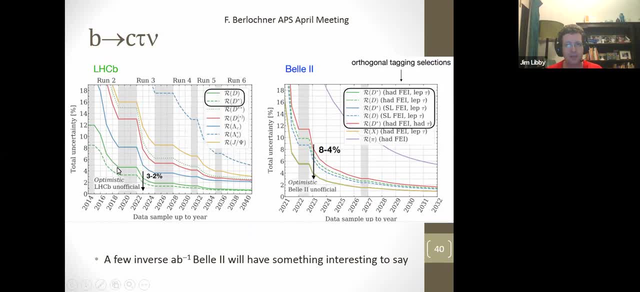 we're pushing down the measurements, particularly of RD and RD star, to a few percent. Some of the lines here on the Bell plot are overlapping with one another And we'll have something more interesting to say on this, particularly on Bell 2, within a few inverse. 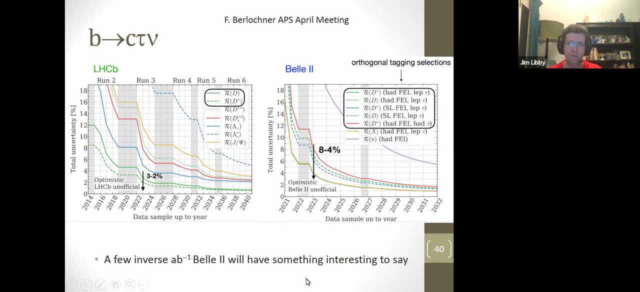 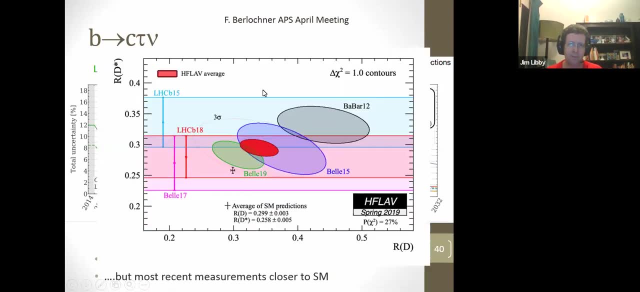 attabans, because we can average together all of these measurements. So I think the situation with B2C town new will start to become clearer. but I must be a little cautious and- something I mentioned earlier- there is some skepticism around these results. 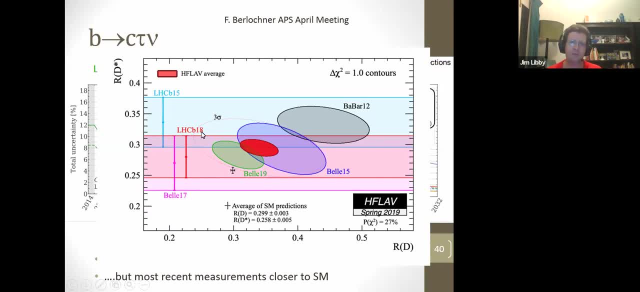 based on the fact that the most recent measurements from LHCb and from Bell are actually pretty much compatible with the standard model. So there is some tension amongst these results. It's not great yet, but it desperately needs more data and more measurements to sort out. 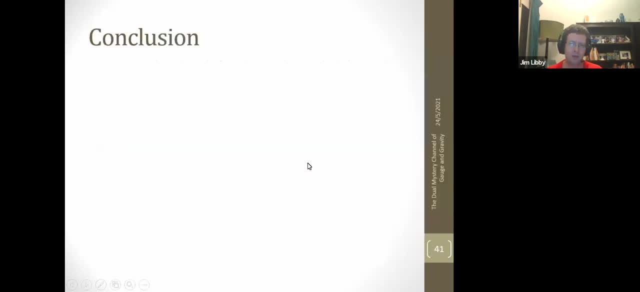 what's going on. So, to conclude, getting to my Dickens, I'll take a tale of two cities. In some ways it was the best. I think it was the best. I think it was the best, I think it was the. 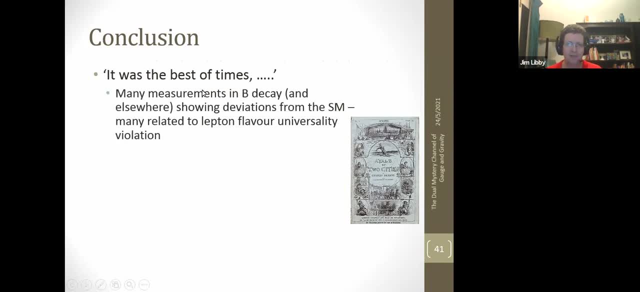 best of times. We have many measurements in B2K showing deviations from the standard model and many are related to a single source, lepton flavor universality violation And we seem to see perhaps consistent new physics models can accommodate them. But it's also the worst of times in that there's no single five-sigma observation. 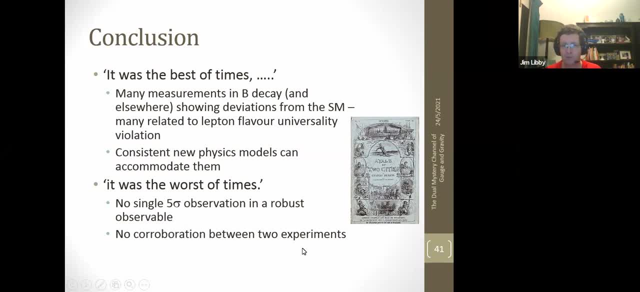 in a robust observable. There's no corroboration between two experiments, And new data coming from both LHCb and Bell 2 requires patience. It's going to take several years before we'll be able to resolve the status of the anomalies. So that's it. Sorry, I overran. 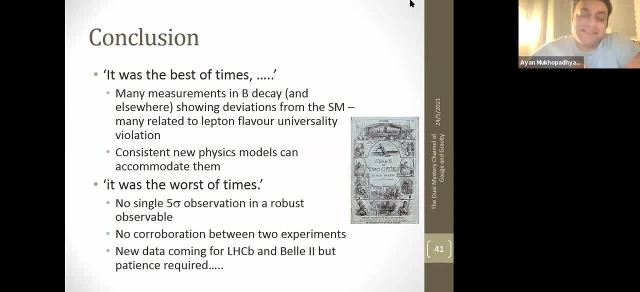 Thanks, Jim, It was a very great talk And it was, yeah, thanks for this very detailed story And it was quite. we have some good idea now, hopefully. So some questions now. Hi, Can I ask a couple of questions? 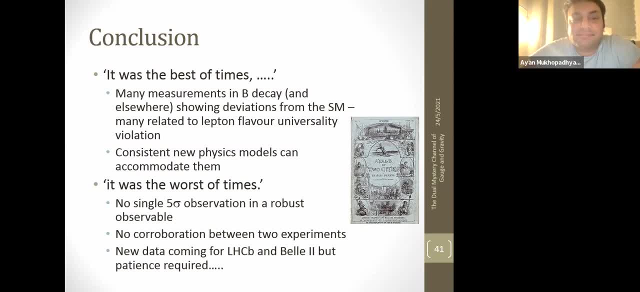 Yeah, sure, sure, Okay, Yeah, just this first point. it was the worst of times. B2K star LL, isn't that single one? more than five sigma? No, no, none of them. None of them are five sigma. 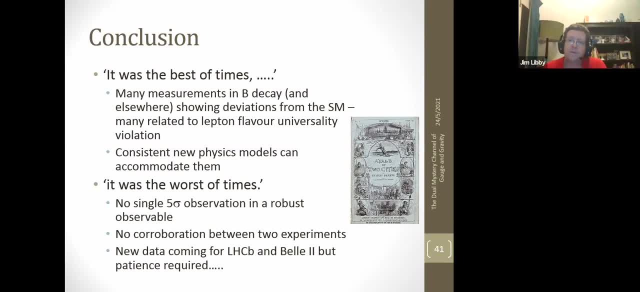 So only this, only the global interpretation. once you put all the measurements together and you do the Wilson coefficient analysis, you'll get something that's five, six, seven sigma. So there is a consistency. B2K, star LL, the angular distribution. that alone is how many sigmas. 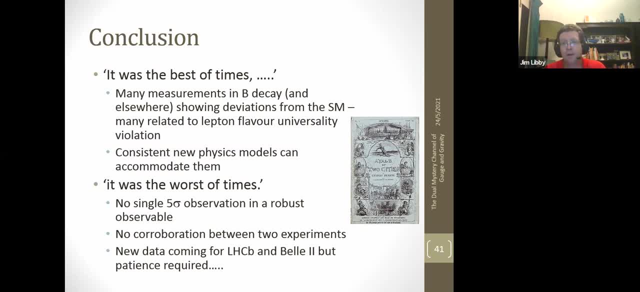 Three, three, just over three sigma. So one expects an LHCb update on this at some point. It's been due for some time. They've got more data. That's just from one data. It's not all the data, But it's not going to be enough. 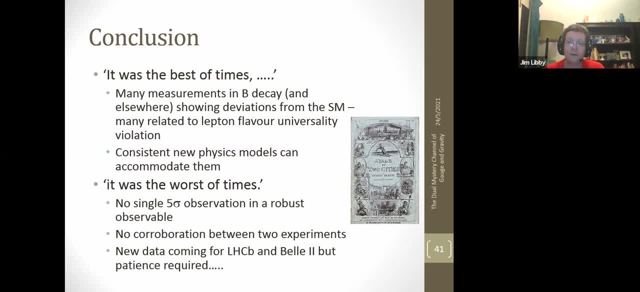 It's not going to be enough to push it to five sigma. It's not that big of an increment. So one other thing about this. I guess the RKRK star, I think you said that you would expect a larger deviation in the muons in most models, but I thought you also said that the experimental 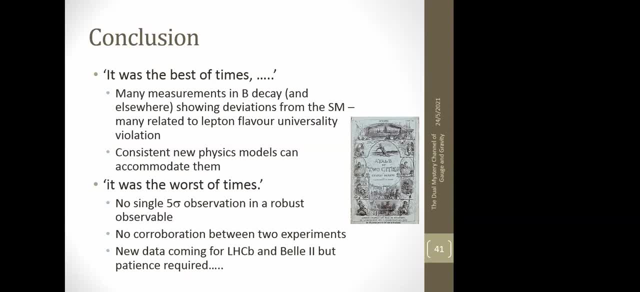 mu is the one that's showing the deviation. Yeah, that's right. Did I gather that correctly? I mean, these are odds, right? Yes, so if you do a branching fraction measurement from the lhcb data, it's the electrons are spot. 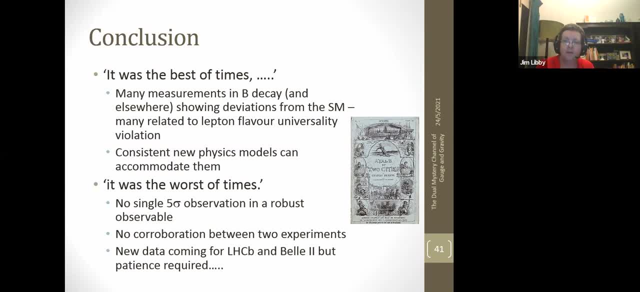 on the standard model prediction, the muons are low but the uncertainties are larger then because it's a branching fraction. you know you don't benefit from the ratio, but it looks like the the electrons are correct and the muons are low. yeah, i suppose it's just a prejudice and there is. no real- uh, you know, experimental justification for why we should think that deviations in muon is going to be more? no, that there are. there are um i, i have seen talks on this. there are. there tend to be better constraints coming from other measurements, if it were in. 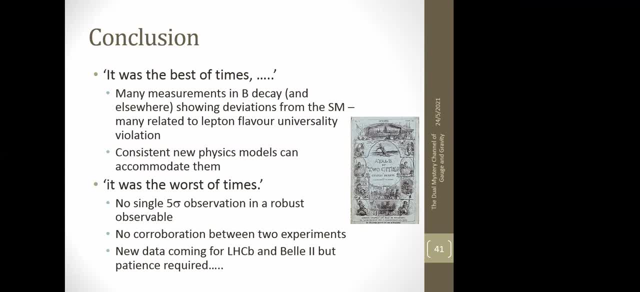 the electrons i see so. so it does make sense that it might be in the muons and it's related to second and third generation rather so. so it's. it's actually it's relatively these models that you have to build you. they pretty much could have minimal coupling to the first generation. 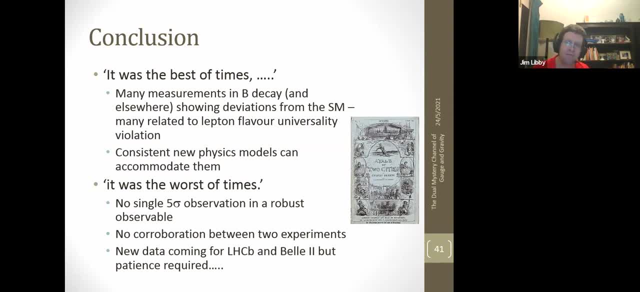 to escape things from the lhc essentially, otherwise you'd have up down quad couplings and things, so they've all got to come in in loops and it so so it's basically second and third generation. into is where you'd expect to see deviations. oh so it is the experimental results. 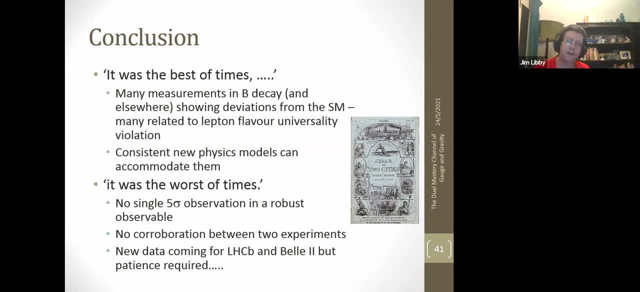 are consistent with that. yeah, yeah, okay, i thought i got it. sorry, no, maybe. yeah, okay, no, i think i misunderstood. okay, yeah. so even that, well, even that kind of a Kibibo angle anomaly, you put the new physics in the muons and the taus and you can explain it. 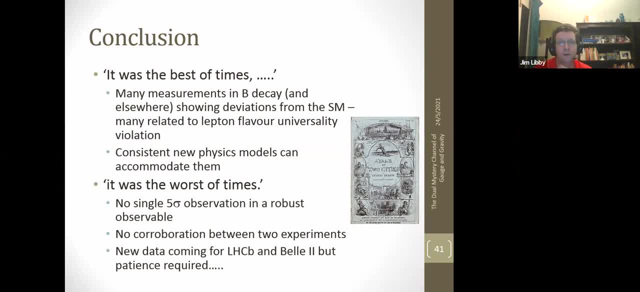 so so that's. that's actually quite an interesting one, because that's also at this three sigma level, and these are very well understood measurements essentially, but so that that's something that I think will be talked about more and more in the years ahead. yes, so you showed this. 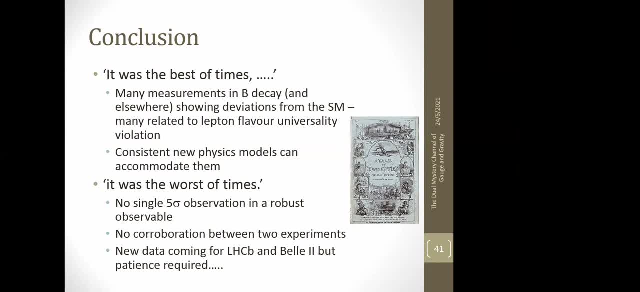 b to sll and then also the tree level b to d, star tau mu, with this lepto quark kind of. you know an explanation, I think, and so putting them together, you know a single mass scale would do. do it for both of them, or do you have to assume different things, or what? yeah, so my understanding. 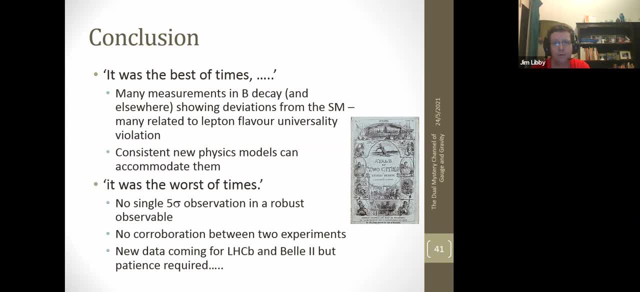 is, you can do it and again you, you tweak the couplings, so it's very much second and third generation only you only have minimal couplings to first generation and and you would have to have a sort of tev range, lepto quark to do this. and there are quite a few papers which I probably 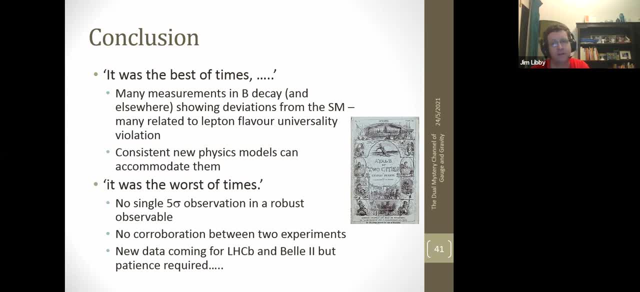 if I'd had more time I would have looked at where they then talk about complementary signals. that would be there in high pt physics. if you have such a lepto quark, I can't remember what they are off the top of my head, but I have seen talks about this. so there is some complementarity there, but the problem that 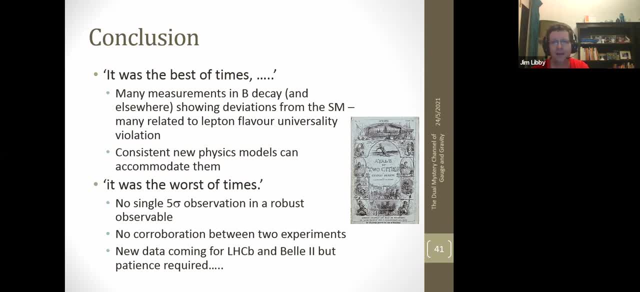 people always talk about is this uv completion, because you're not adding additional. you need to add additional higgs sector to make it stable in some way, and and that's not there and I think people have a hard time, they, they- there's talk of patty salam and things you can. 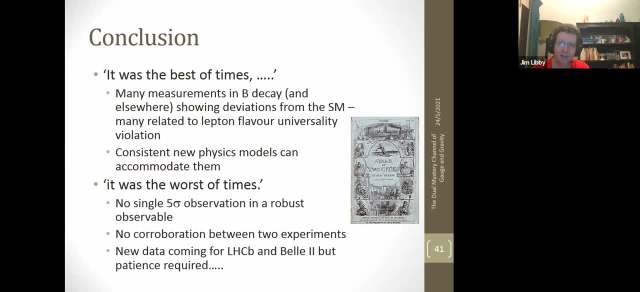 do, but I'm, I'm, I'm out of my comfort zone when I start thinking about all of this. so yeah, I actually have a related question. Sreerya, can I ask, or you have time? no, I was, I have one more. so if there is time, I can ask later. 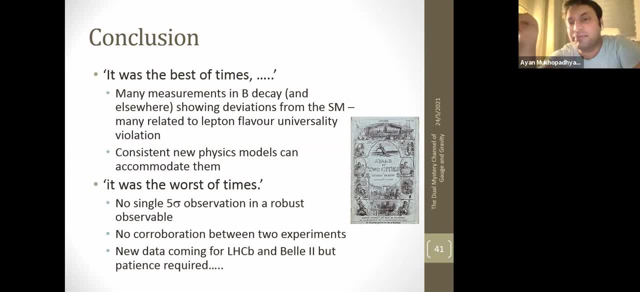 oh, no, no, okay then. okay, maybe, okay then, but my question is slightly related to what you're asking. so this and also what I was asking before, so this four, four quark operator is something that we must have seen and we can, of course, see it, but, as you said, it is only makes sense if it involves. higher generations. but then my question actually is that is it? is it because it involves higher generations is hard to directly see it, otherwise I don't see why it cannot affect in general some higgs decay also in a from effective field theory point of view. it cannot, but because it's involving 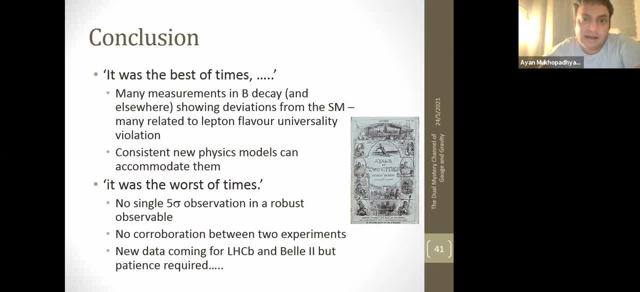 higher generations is harder to. it will be harder to see it in in in other other processes. that that is my understanding that you can escape. so, um, so, but so if you are trying to in b2sl, if you're trying to use a z prime where the constraints are actually pretty stringent in in terms of the lhc, 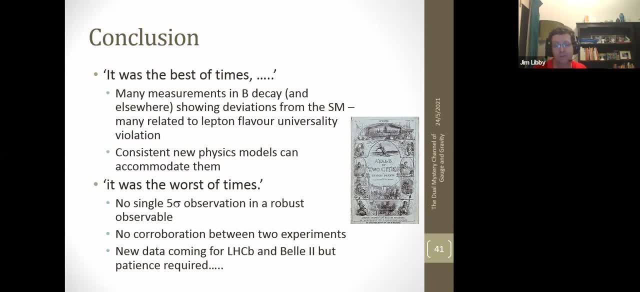 you can do it if you say, oh no, it's barely coupling at all to anything other than the third generation and you just put it to be coupling to the top and your leptons, and then you can say, yeah, you wouldn't, you can escape all the limits, but you have to make it um, very much, uh, generation specific right, or? 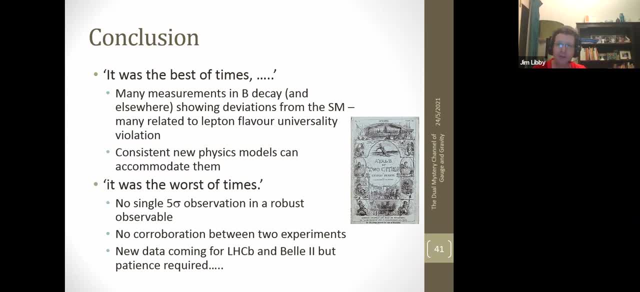 there'll be some coupling between the second and the third, but there'll be limited coupling to the first and you can escape it. but if you say that there's going to be, that it might be some universal coupling amongst generations, it just won't work. yeah, so you've. you've got to say: 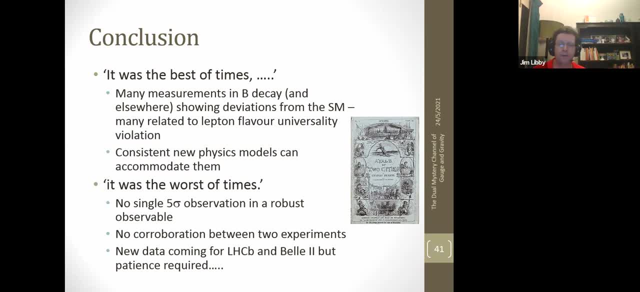 there's something special about the higher uh, the more the second and third generations, particularly the third generation, and this is precisely what is making it harder to. even if you look at the differential hdk cross-section and certain processes, it's really hard to get enough background- i mean enough high limonicity- to 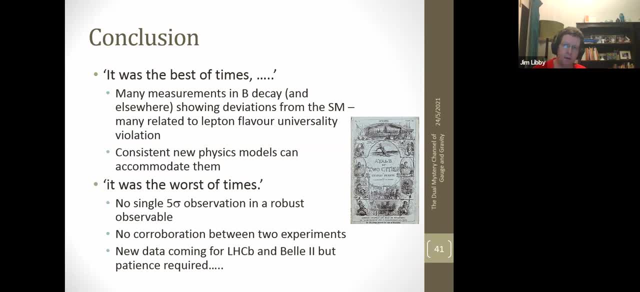 to see such effects there. yeah, yeah. so i so things i've seen have been talking more about. it's probably higgs to tau tau, i think you can see something. and there's, uh, i know i'd have to look back. i, i, i, i, i remember seeing a talk. 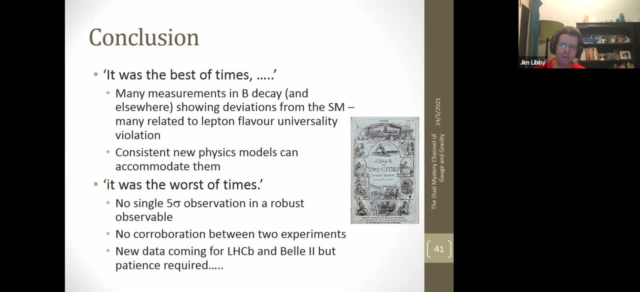 maybe in gino's talk. actually there is some discussion of this where he has the potential signatures that are there. and then, of course, now people are getting interested in this excess in cms at high, uh, dilepton mass in the droian cross-section and okay, it's two sigma, but you know people are. 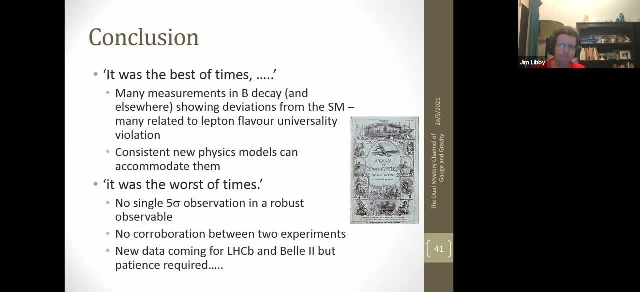 now starting to wonder whether they're going to be able to do it or not. i think it's going to be a bit of a wonder whether something is going on there. that sort of then would go against a lot of this, though, because that seems to be a first generation thing then. 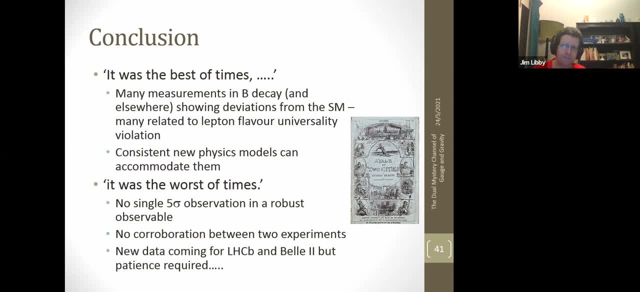 so i, i'm not sure how they square the circle with that, unless it's somewhere somehow in the loop that it is affecting in the loop when it's a higher dimension operator, sometimes it can, yeah, yeah, i, i it's uh. anyway, this, this is. you know, all we can do as experimentalists is just measure as many things as we can and as 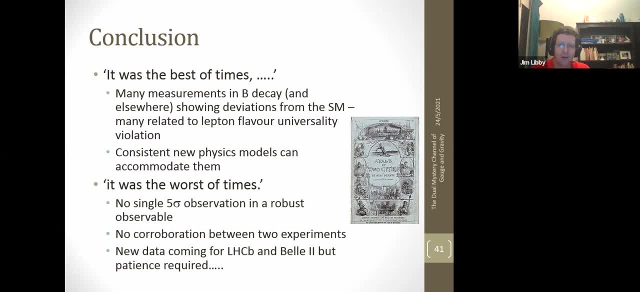 precisely as we can and um you know i ultimately the gold standard it will be if lhcb and bell 2 agree on all these things experimentally and and they are very different measurements. we have very different problems in the two experiments and and it would give great confidence if 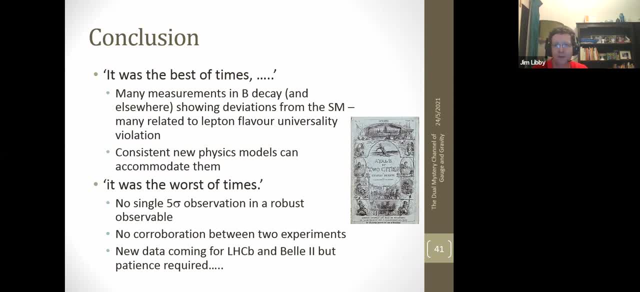 in three or four years time. if we all agreed on the value of rd and rd star, then i think everyone would accept that something is going on there and it will take longer in rk and rk star. but again, i think that will be a similar situation where, if 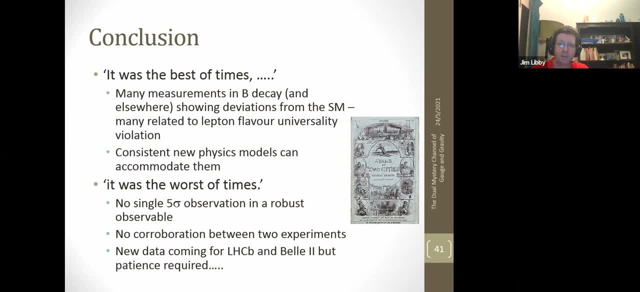 both experiments see the same thing. it's unlikely to be the same mistake, given that the experiments are so different. and yeah, for example, in the uh, in the beta c, tau nu lhcb's problem is the background, whereas our problem is really just efficiency and and signal. 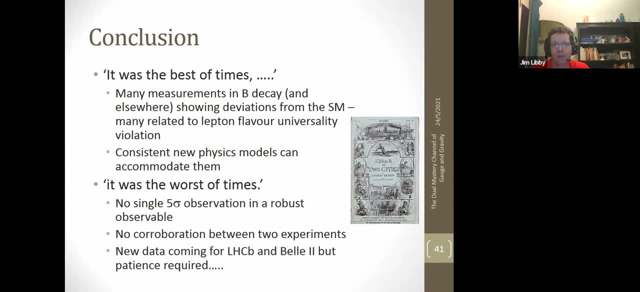 extraction because our rates are lower. but, um, we're, you know it's a different, different set of problems. well, uh, you had more questions. yeah, i have just one more if there is time. oh, sure, sure, yeah, so so i just. there was uh one which i thought was um the c9. 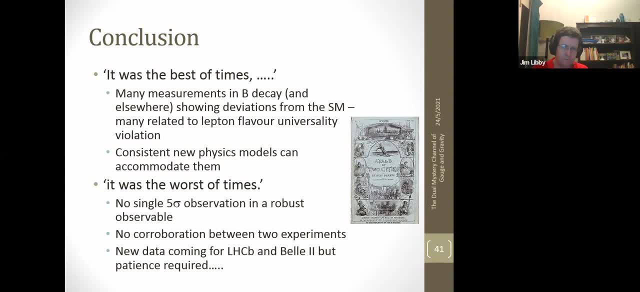 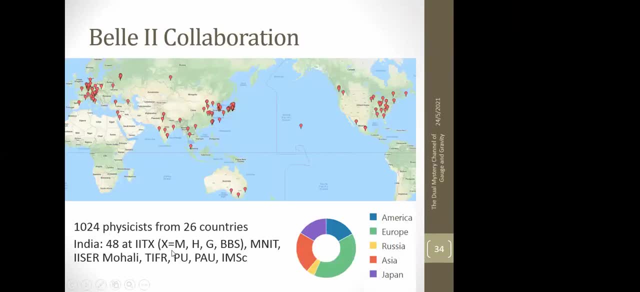 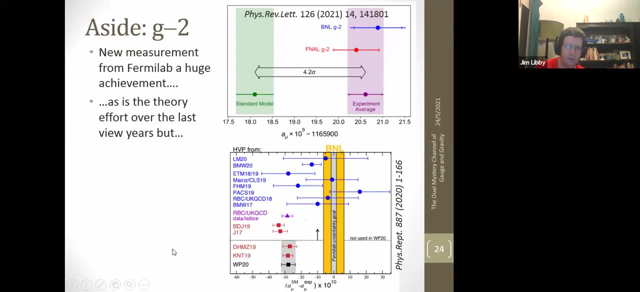 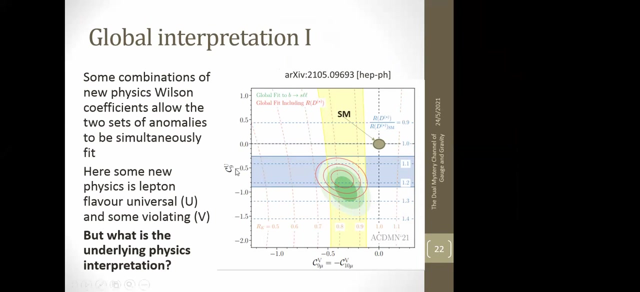 interpretation: c 9, c 10 prime, i think, for um b to d star town. you also put into the thing i missed what was there was a c9 prime you. oh, yeah, this this one. ah, yeah, okay, sorry i went, i was getting stressed about the time. this one, yeah, so this one, so um. 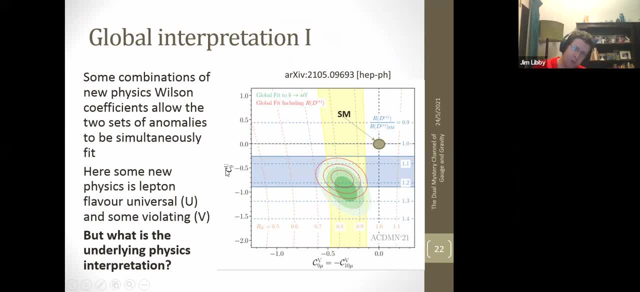 this: yes, so that means this is stopped by any random here. then g, but it only means that it's not just a quatre v magistrateاس model, like in terms of weak couplings. so this is, this is universal. so there's some alteration to: yeah, well, this is also v, this is just c9. c9 minus c10 is effectively v minus a in this. 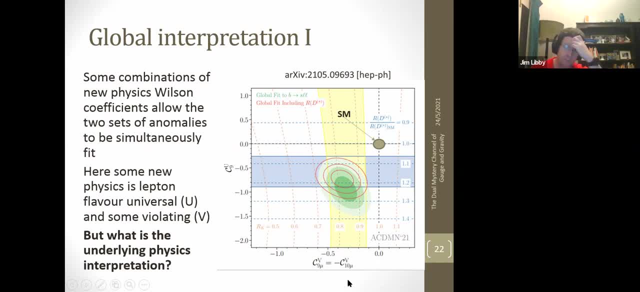 as far as i understand it. so this is just adding more left-handed current, okay, of some type less left-handed current, yeah, yeah, um, but to, to do all of this together, you've got to modify uh c9 differently in the different generations, so that, so this one will be affecting 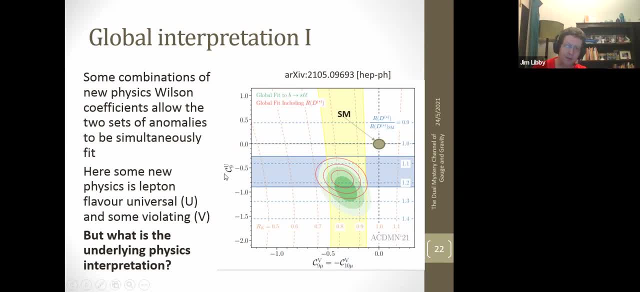 uh, just, i guess it's generations two and three and and this will be affecting one, two and three, and by doing all of that you can, you can fix this up. so, uh, so the new, is it like at the x-axis, the? so yeah, i, i, i, so i, i think yeah, it started in, only yeah, i don't, i guess i get. 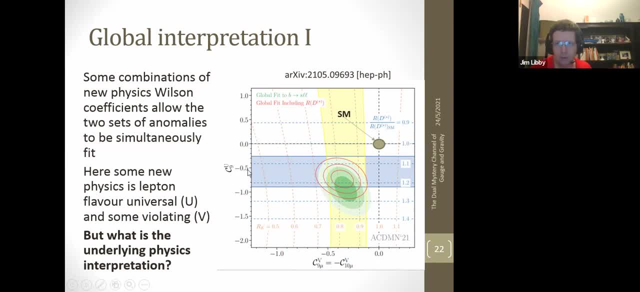 yeah, so this would be affecting the tau and the muon, okay, and the electron, and you can get. you can get this, but i i'd have to. i'd sorry i didn't read in detail. this is this paper post morion. okay, all right, which? uh, where? so this is sebastian and collaborators. 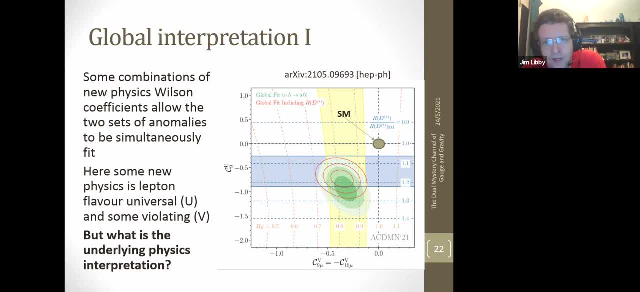 so who's one of the leaders in all of this stuff? so you are convinced that we are seeing new physics in all of this. i i slowly get more and more convinced and i think the rk was just certainly a step in the right direction. it's a variable which is, i think, very 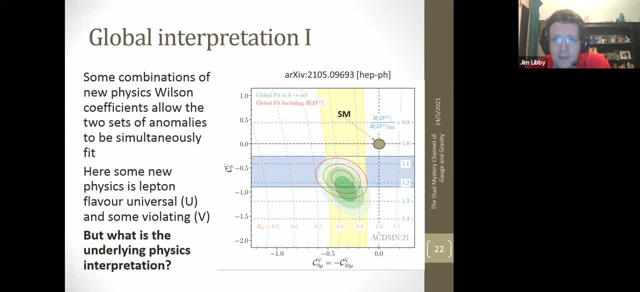 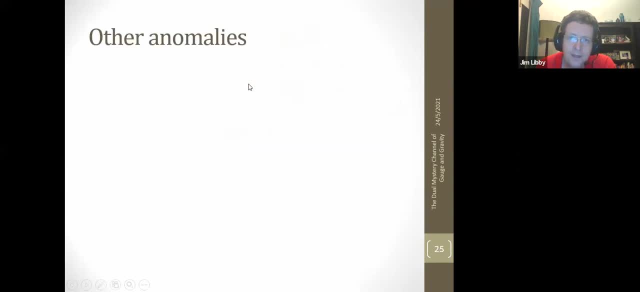 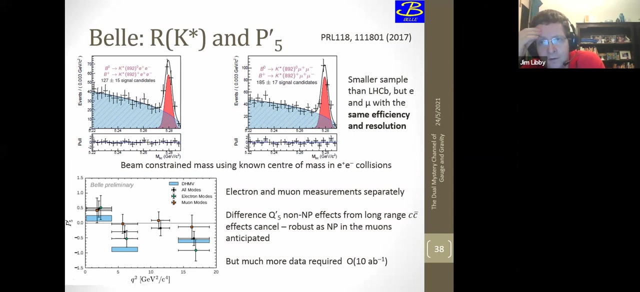 reliable. the measurement that would really convince me, which i think is a long way away, unfortunately is- sorry, i'm, it's this one. if you, if you see in the differential distributions a real significant difference between muons and electrons, that would be really quite convincing that there's some new physics there. 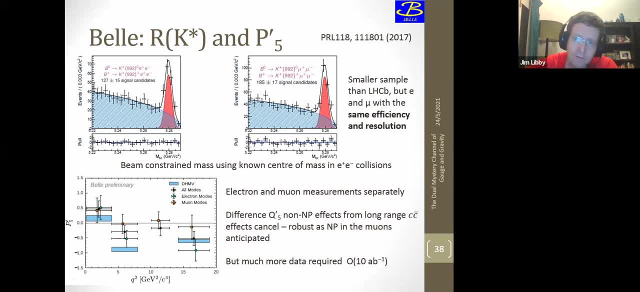 because it. and then you you're taking the difference, so you're taking out a load of hadronic uncertainties and doing that. the only thing that can be driving such a difference would be some, um, new physics going on in that penguin loop. but you know, there are other things that 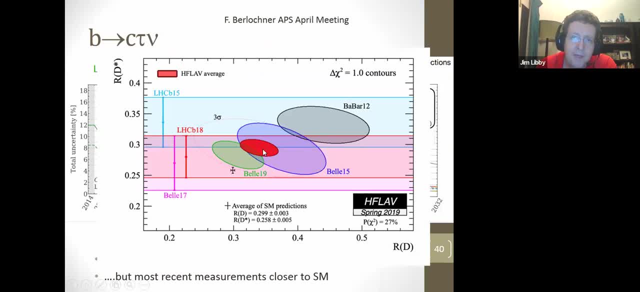 can happen. as i said, if, if LHCb and Bell two converge on the same value for rd and rd star, then i see nothing. you know, i don't see why anyone would doubt these measurements. there has to be something happening there as well. um, and you know, rk is 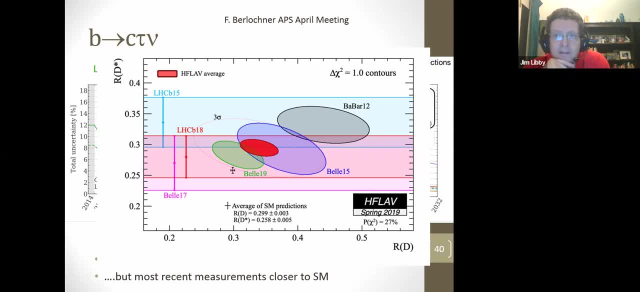 as i said, a robust variable, but you'd like it over five sigma and you'd like to see it in bell two as well, where there'll never be a doubt about the electrons compared with the mutual speed of the jumper. so we'll see if that's going to happen, but it would be a question you 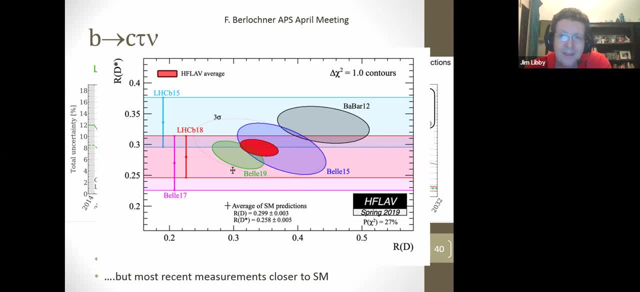 know as a option. if LHCb and Bell 2 converge on the same value for rd and rd star, then i see where there's there's always. people always worry. however much work lhcb do on their electrons, people are always going to point at that plot where you have the huge background. 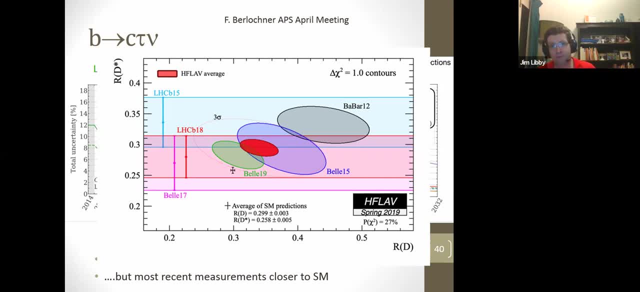 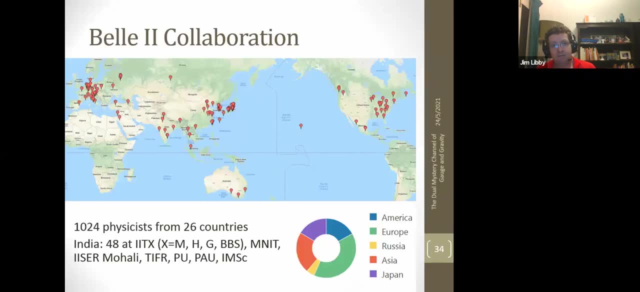 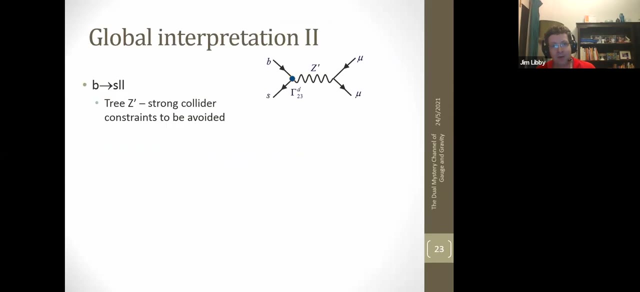 compared with the muons and say: do you really understand this? to 15 percent now, that i think is really unfair, because i think they've done a a good job. and you know i'm i'm an xl hcb person, so i'm probably a little biased too. but 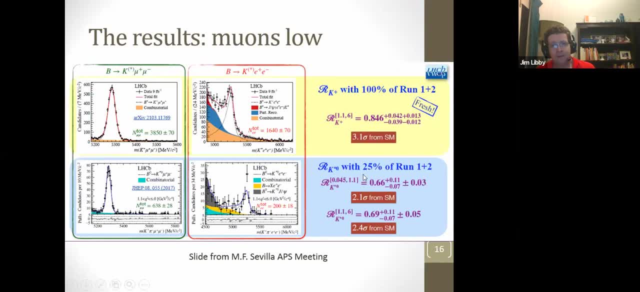 i think when this finally comes, when they've got the extra 75 percent- and these numbers are significantly lower than rk- if these come out low as well and with some significance, then i think it's starting to look relatively convincing. but again, everyone will say it's the same electron. 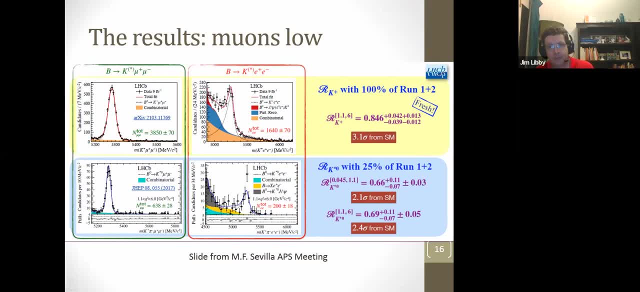 reconstruction. so if that's wrong- but I don't- so yeah, that's a hard one without Bell 2. but Bell 2 just needs a huge amount of data and needs tens of inverse attabonds to do this. but given that statistical disadvantage, yeah, given that. 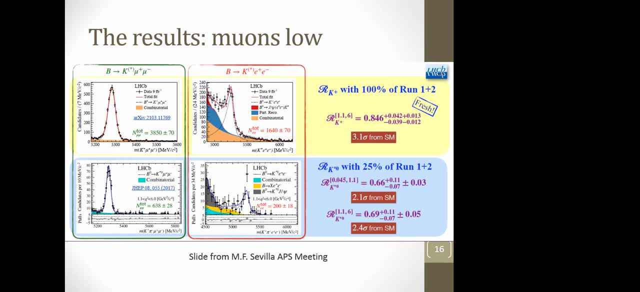 JSI is a controlled thing, you know. it's hard to see how it can go wrong. I suppose right as you said. yeah, but okay, so to go with the naysayers. the thing you must look at, then, is this background underneath. okay, what they're saying is: 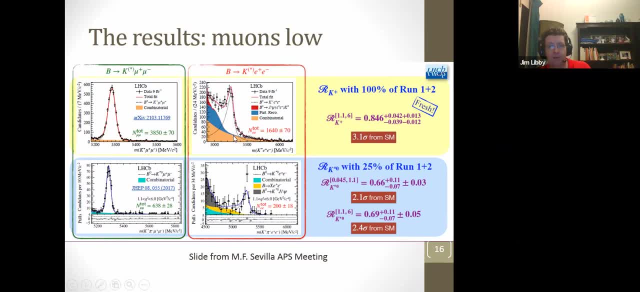 they know this shape of this blue stuff really well. yeah, so if, for example, you've got this wrong and you've bled in 10% extra background here, that means your electron signal would then agree with the muons and RK is one. okay, if you've. 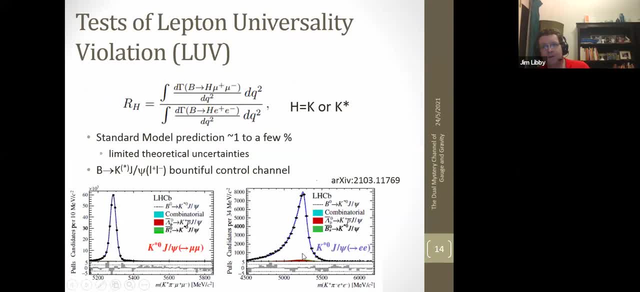 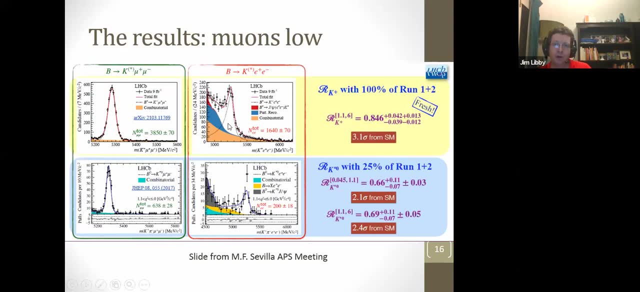 got the background wrong. then you look at JSI: there's no background. so you, you can't, it's not, but it's hard to know how they get that wrong. that's from an experimentalist point of view, but this is the concern that you have, that this 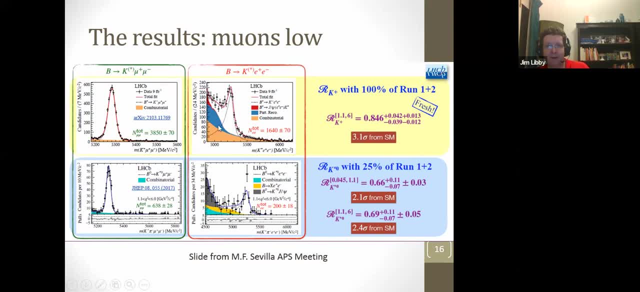 is not a pure signal, background signal it's not as high purity measurement. so therefore you have scope to you know. just parameterizing your background incorrectly can change your yield. sorry, if you uh get this blue thing wrong, then your JSI is going to go wrong, right? 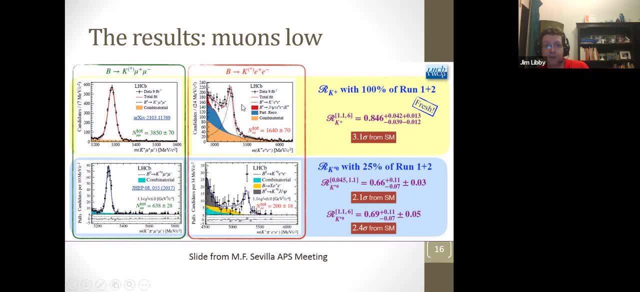 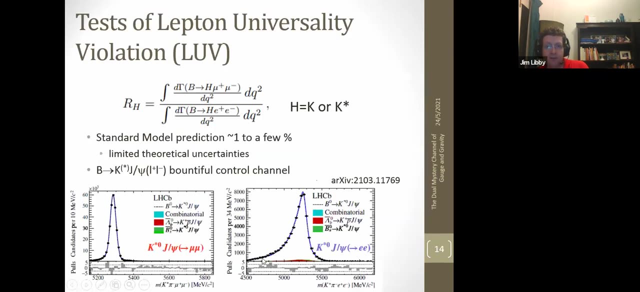 that's no, no, no. this is purely there for the. this is only there for the R BK EE signal, because, sorry, there is some background down here, but you can't see it. you can't even see this combinatorial, because it's just so much signal. 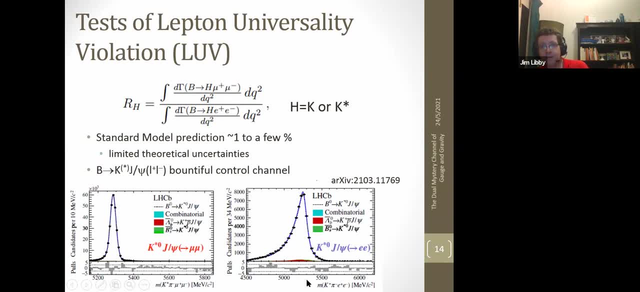 over background. so there's no way they can even control the level of the background because it's swamped by signal. of course there are sidebands and all sorts you can use and they do this, but yeah, I'm just telling you what the doubt is. I 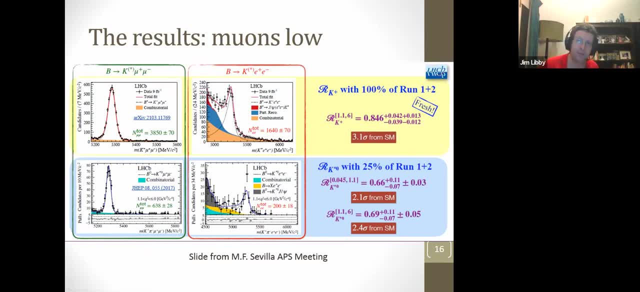 you know, I don't really believe that's a problem, but it's just a very different scenario to to the muon measurement, for example. just looking between left and right here, you can see how pristine this is in comparison. and it's all down to this, these issues. 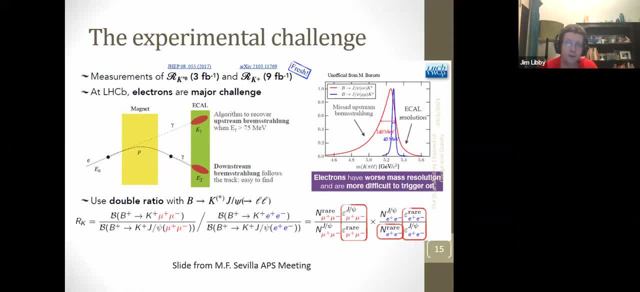 of the brim strata. okay, great, now, if you, if you'd listen. so, LHCB, if they had millions of dollars, they'd upgrade their e-cal, but no one has millions of dollars anymore. so it's, I think they could build a very nice calorimeter. 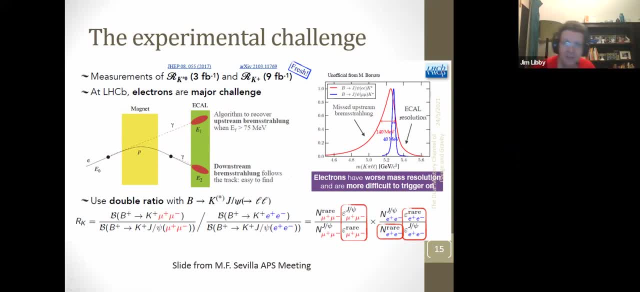 for like a hundred million dollars or something, and then they could. they could probably for possibly the only signature of new physics. doesn't the world have a hundred million dollars? it did in January 2020, doesn't anymore? I don't know. I don't, I don't. 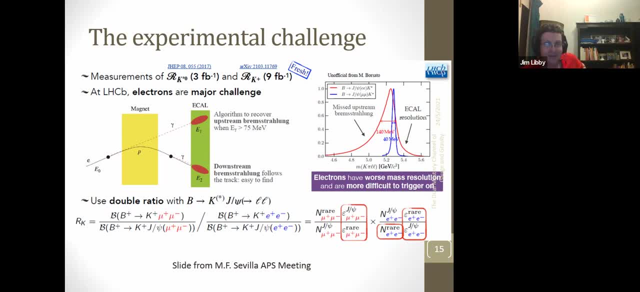 think India's going to be contributing to that effort, I'm afraid. so, yeah, yeah, I know, but now it's a bit. there are. there is talk for their future upgrade, of upgrading their calorimeter as well. you should hear Sheldon Stone on this and Bell is going. 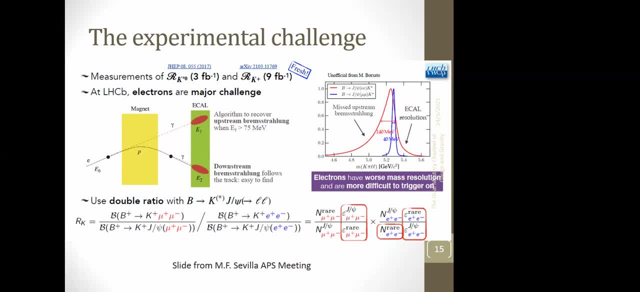 to say something about this at some point. I guess: right, yeah, but we require tens of inverse atom bonds. I think we'll have something interesting around 10, I think. before that we won't have the statistics, we just and then. and Jim, are you there? sorry, I lost. 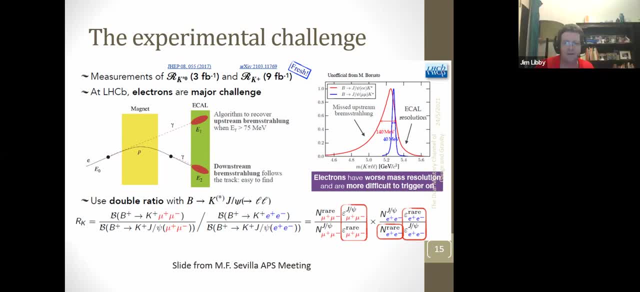 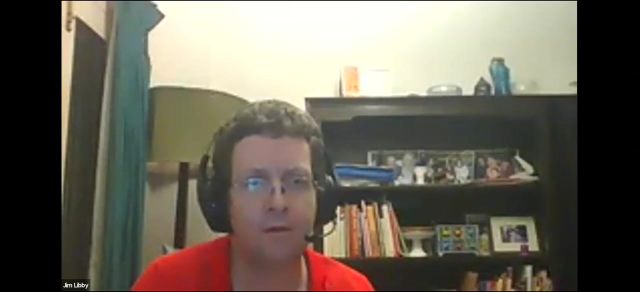 the connection also. yeah, I think he's having some connectivity problem maybe. yeah, I I think we need to end too. yeah, thanks for entertaining my many questions. sorry, you know, might have asked too many questions. I think we started the recording. yeah, yeah, I think we have to. 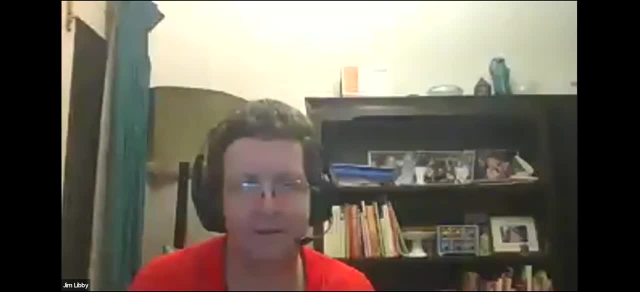 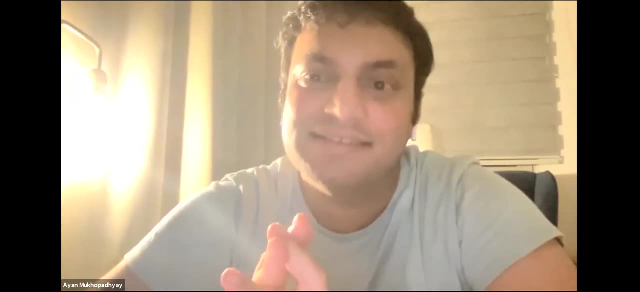 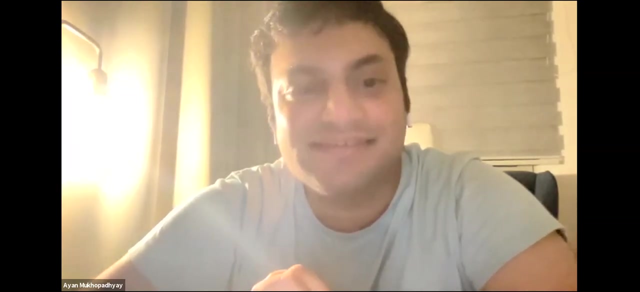 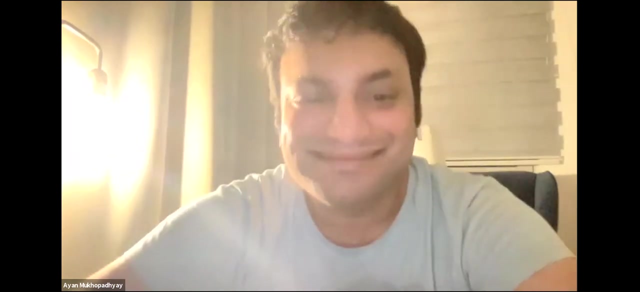 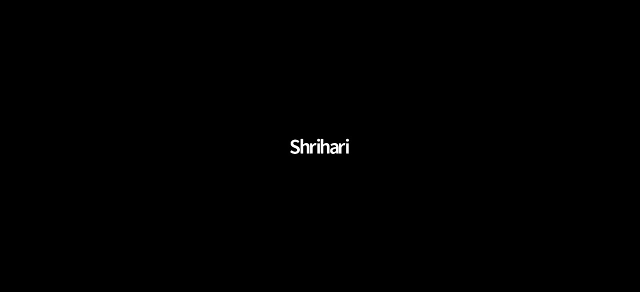 stop now. anyway, it has been quite long, yeah, so, yeah, so thanks, thanks, Jim again for this very detailed talk and thanks everybody for participating. and so goodbye, and then have a very nice evening. and uh and uh and jim, see you around at some point. fire zoom, okay, thank you okay. bye-bye, all right, thank you very much. bye, bye, bye.